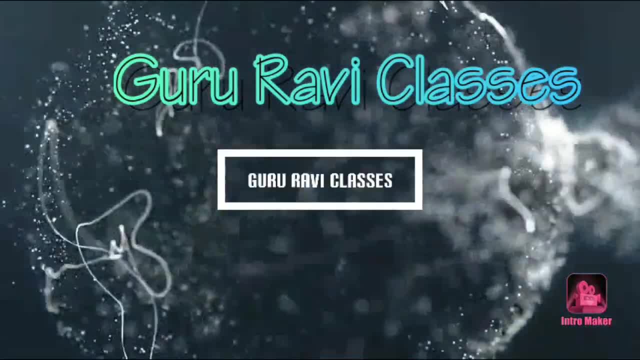 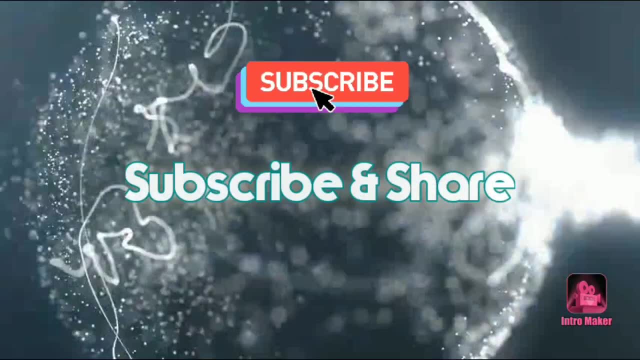 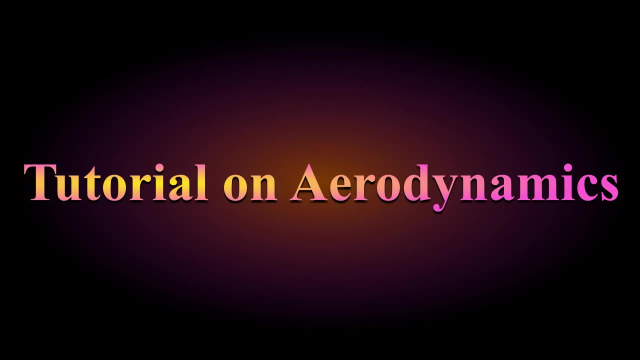 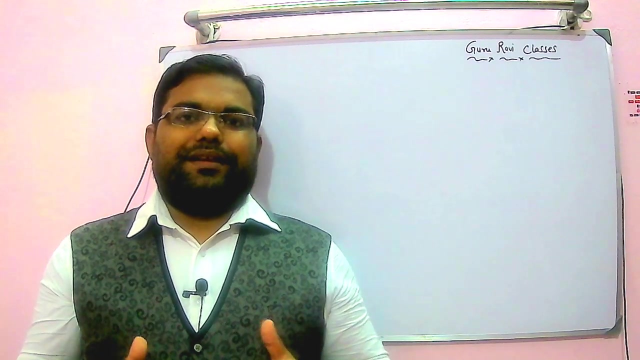 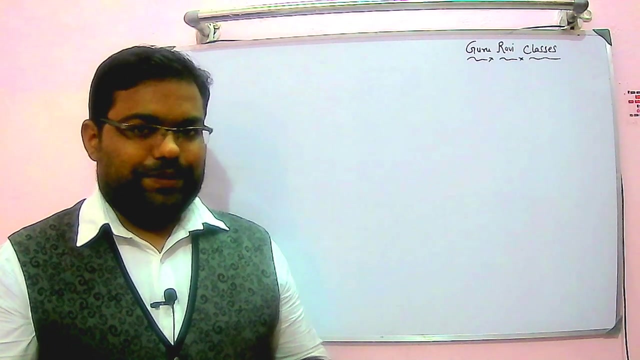 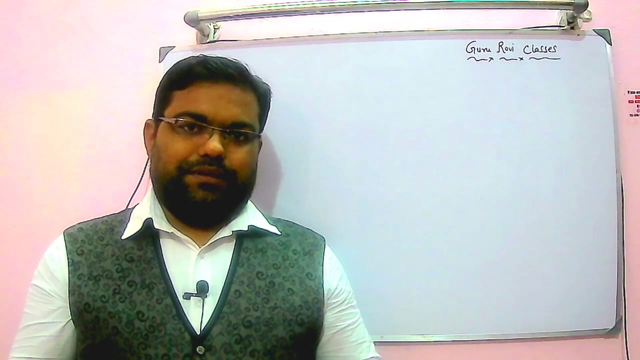 Hi all here Professor Ravi Kumar from School of Mechanical Engineering, Shastra, DM2B University. I welcome you all to the next lecture today in the Introduction to Aerospace Engineering Today we are going to see some tutorial problems on basic concept of aerodynamics. 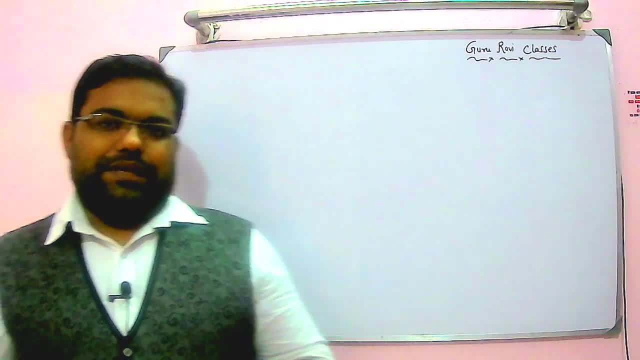 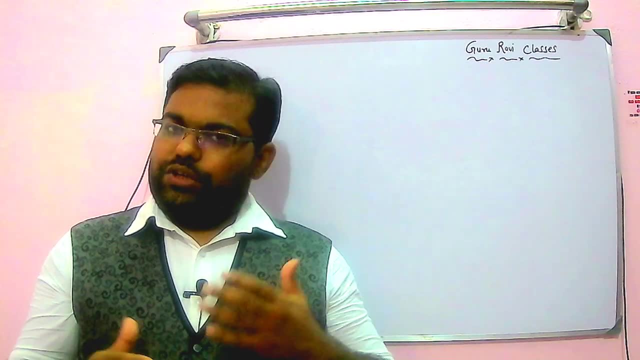 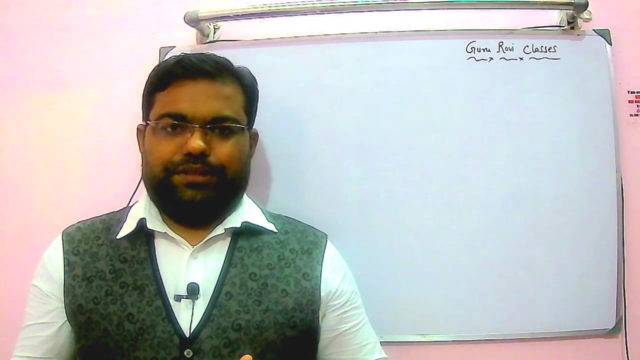 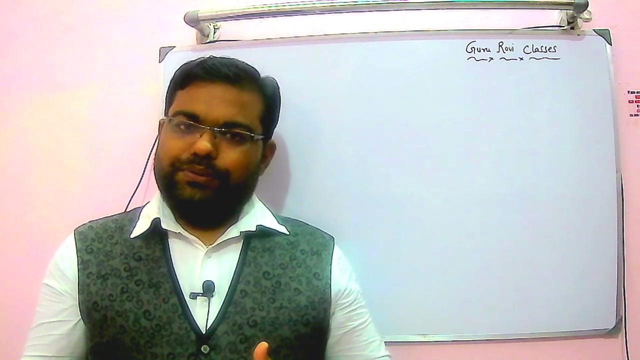 In the previous lecture we have covered the high lift devices. that was the last topic of the basics of aerodynamics. Today we will see some of the numerical problems based on the concepts that we have gone through in the basic fundamental of aerodynamics. So I request everyone to have a calculator with you to verify the answers for the problems that we are going to discuss today. 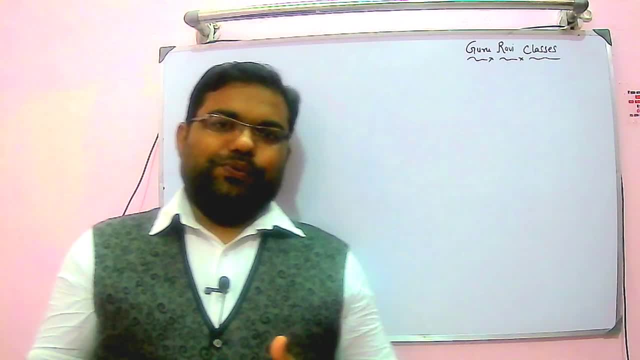 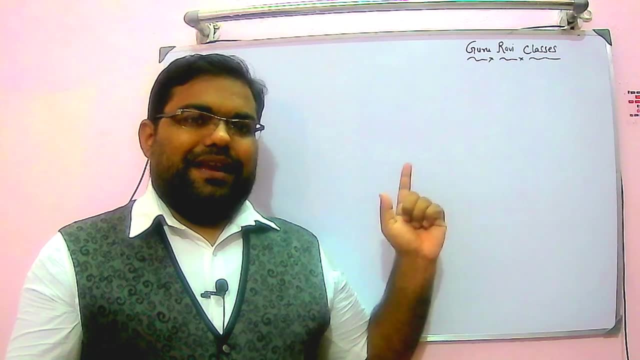 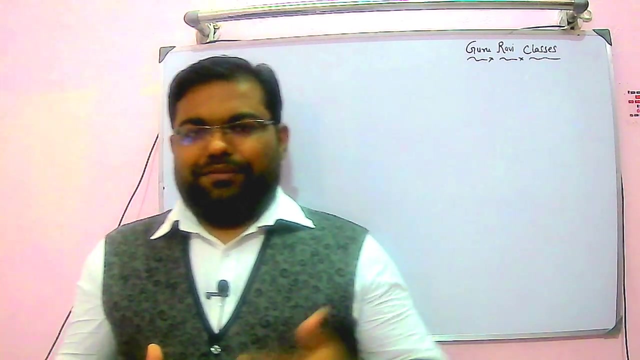 And prior to that, I would request to the newcomers, those who have come today to view my lecture, please subscribe and like my channel. So let's come to the discussion today. So today I will start from the prescriptions of the flow. flow, or that we say descriptions of fluid flow. 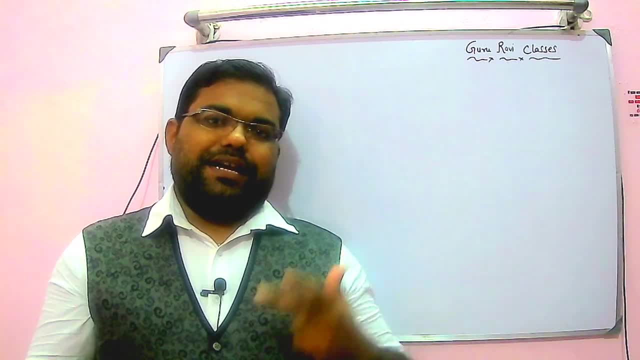 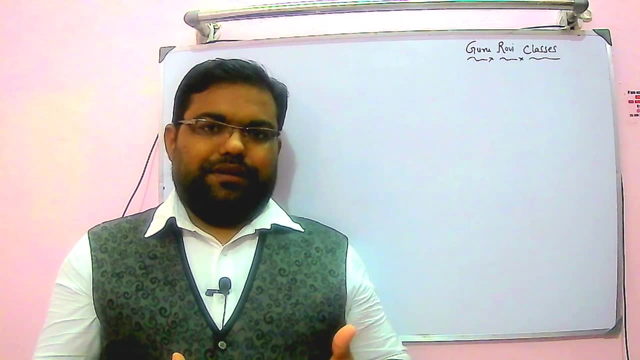 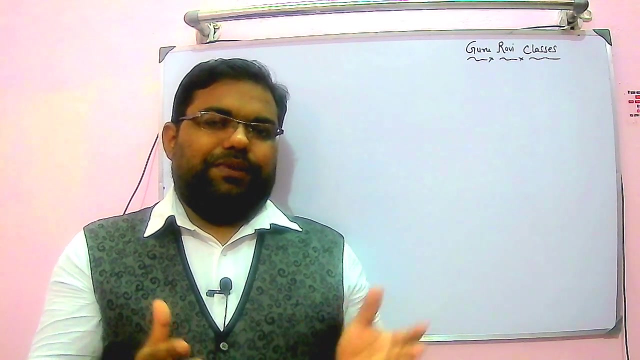 where we have discussed about two approaches: Lagrangian and Eulerian approaches. Right, Lagrangian approach talks about the individual fluid particle behavior. Right, when we are we wanting to you know, know the behavior of certain domain, that domain will have a number of you know particles and we will consider 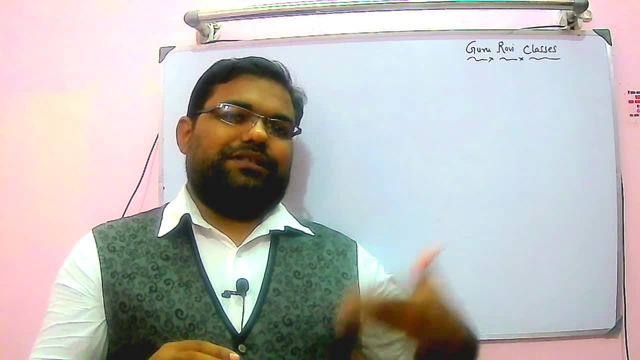 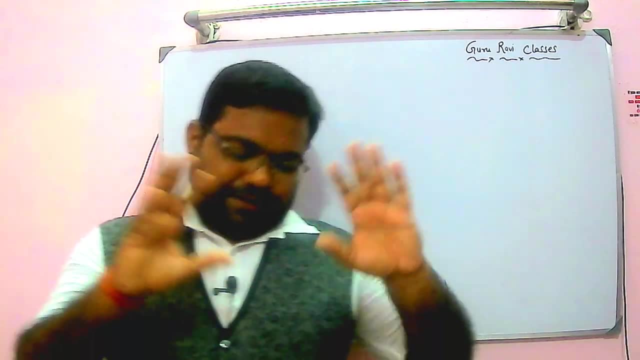 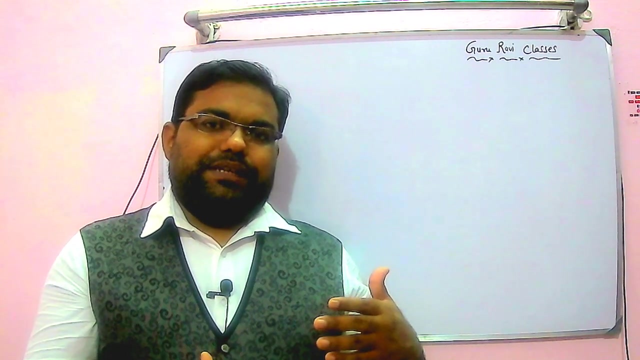 We will consider certain set of particles and we will move along the particles and we will measure the velocity, acceleration And finally, we will say: this is the desired effect, which is create, which is have creating in the given fluid domain as their individual particle need to be, you know, focused. 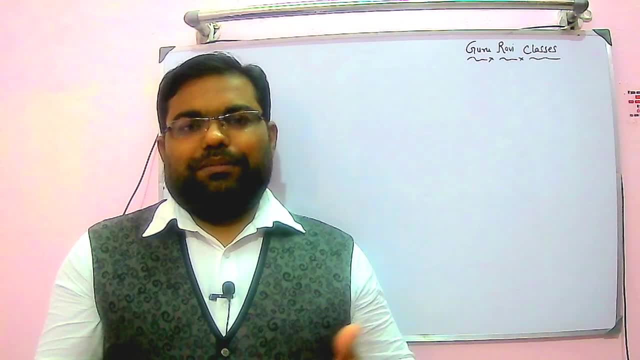 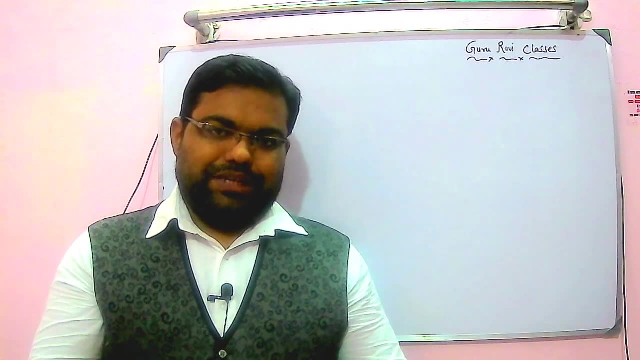 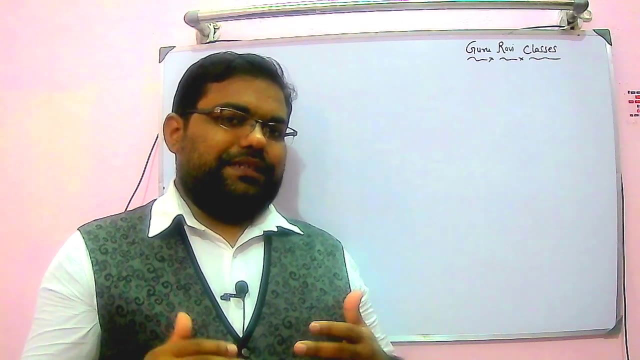 So it requires a number of equations to come up to find out the overall behavior of the fluid flow. So it is very tedious process To counter that problem. the second approach came into the picture, that is, Eulerian approach. In Eulerian approach what basically we do? we fix a certain you know station in the fluid domain and there will be seating. 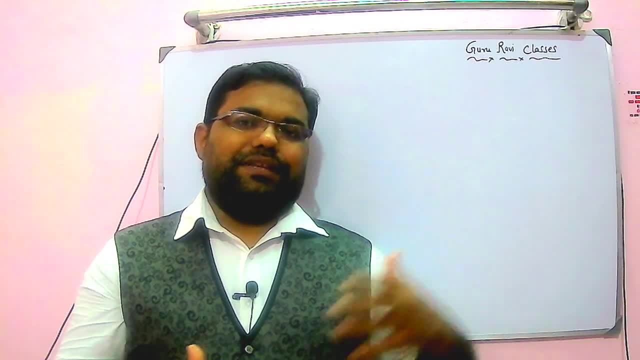 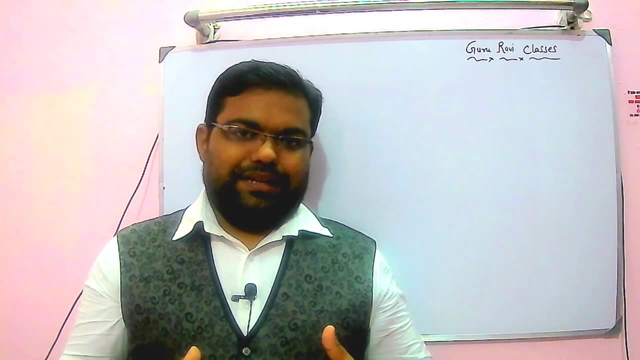 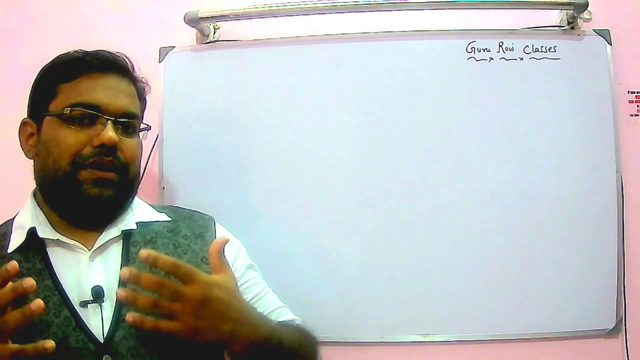 and certain quantity of flow will be entering and leaving the fluid domain. We are simply measuring the fluid velocity and acceleration right, at a given extent. So by a Eulerian approach, right, we can exactly say what is the actual flow behavior. right, and in a very simple way. 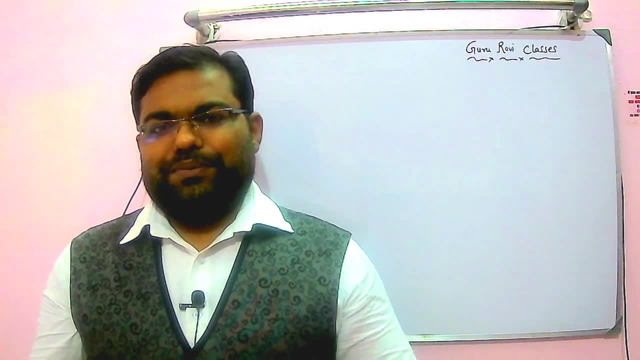 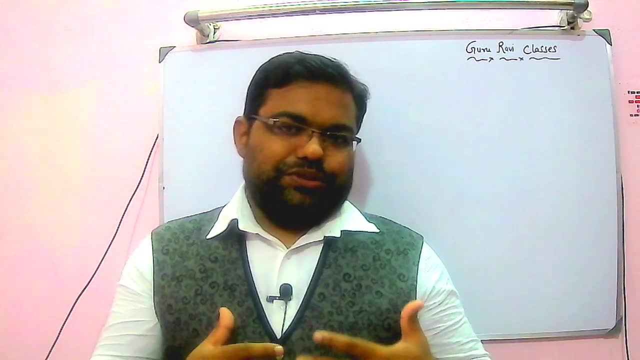 And it requires less number of equations right to come up to the conclusion that certain, you know flow is going to create this kind of effects. So as from these two approach, basically, we came to know that a fluid flow will be described by its velocity vector. 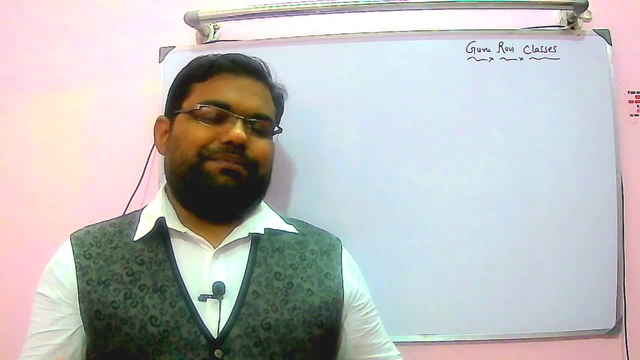 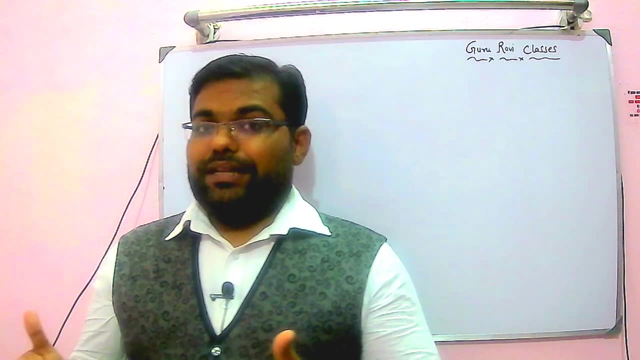 The moment we know the velocity vector, we can find out the remaining parameters, like: what is the force it is going to exert, what is the force it is going to exert over a given, you know, object which is moving through it, and what are the different aerodynamic. 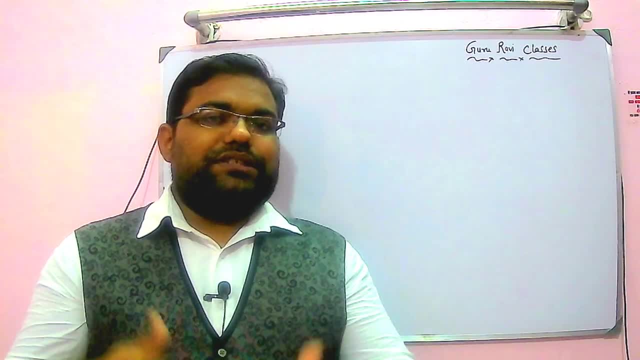 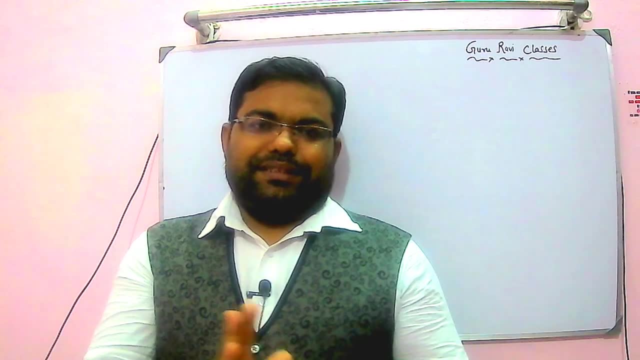 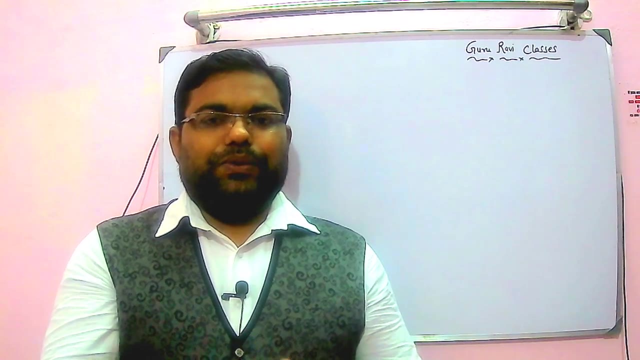 forces right that that are going to be influenced because of the this velocity flow over a particular object. so velocity vector is the necessary thing. so once we come to know this is a flow, the necessary condition for a flow to be existed, like if somebody asking you whether given flow 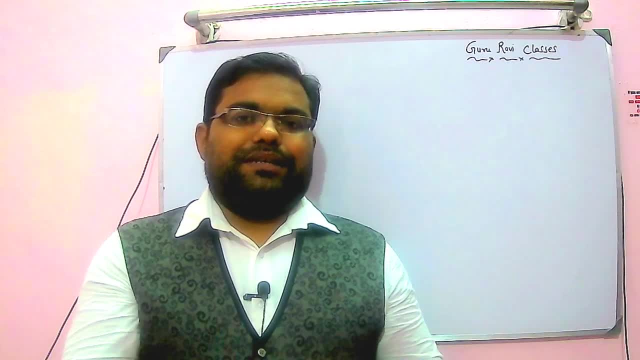 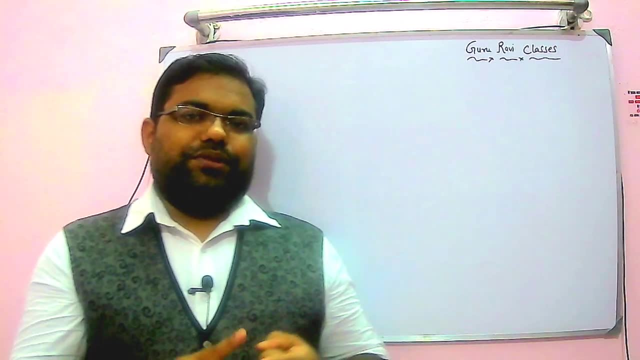 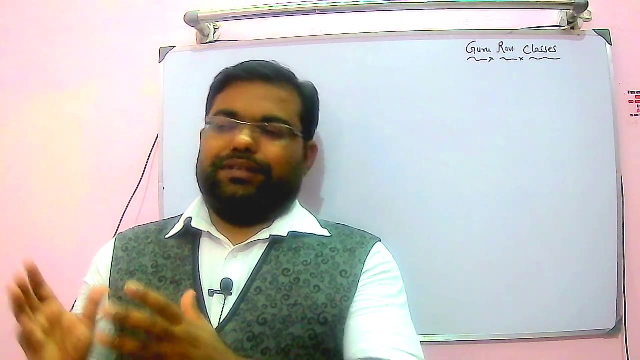 is possible or not. the requirement, mandatory requirement. it should satisfy the continuity equation. so continuity equation is must. right before you know, we can come to the conclusion that the given flow is possible or not. so we start from the dedication. from there we will say, okay, this flow is possible once. once we have decided flow is possible, then we go. 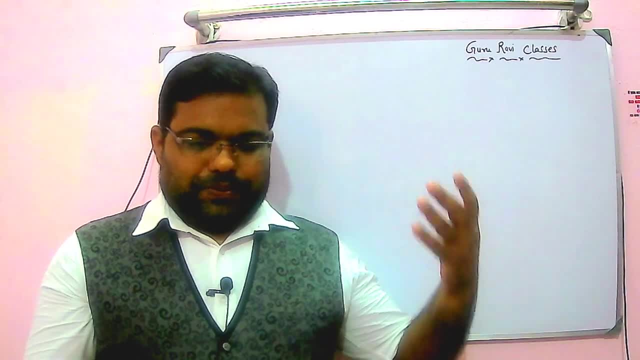 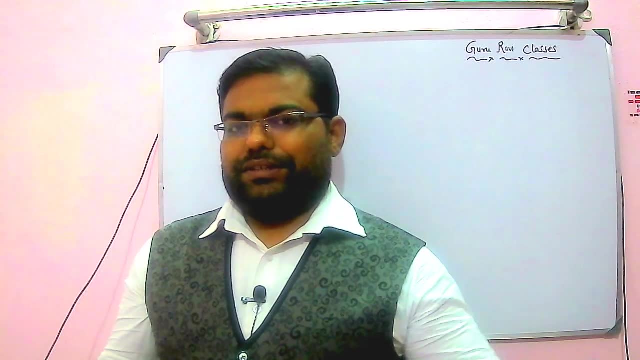 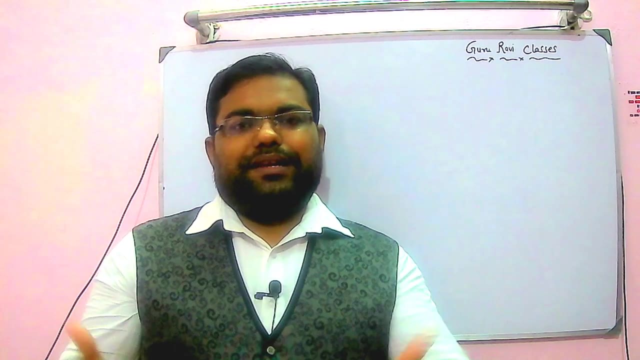 for remaining calculations, right. so we will start today our numerical problems also from that concept, only from velocity vector. then we will see whether it is possible or not. then we will come to the rotation circulation, those all terms that we have already, you know, covered in previous lectures, and then we will come to the wing aerodynamics, right, so some. 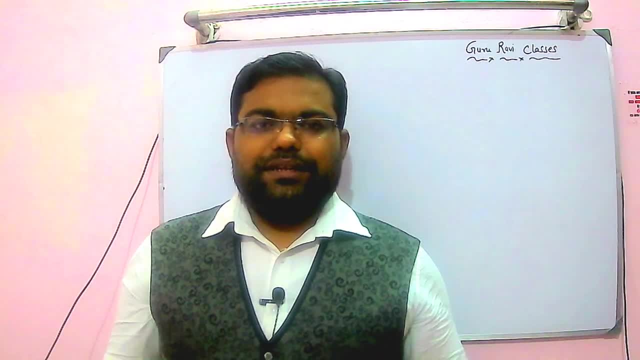 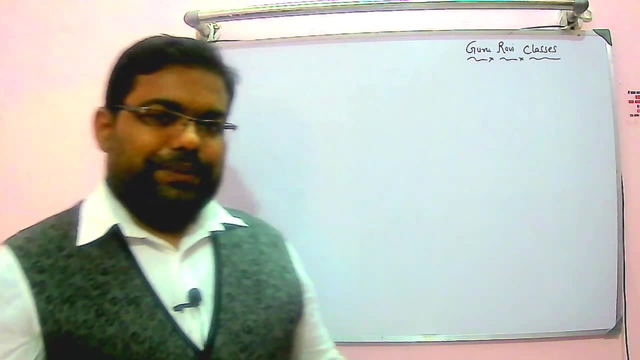 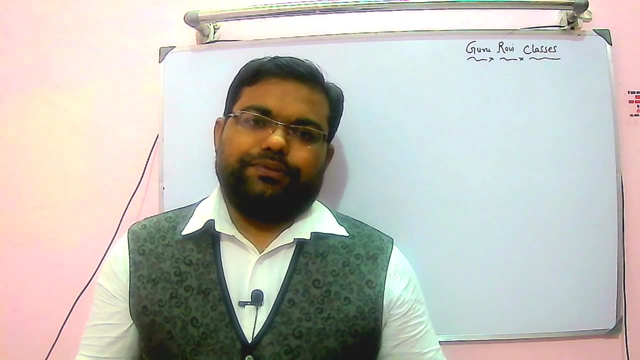 numerical problems based on the wing. aerodynamics will also be discussed today, so i will take the first numerical problem right, based on the velocity vector. so please note it down, i will be dictating here if velocity vector for a given flow demand is given by the air. 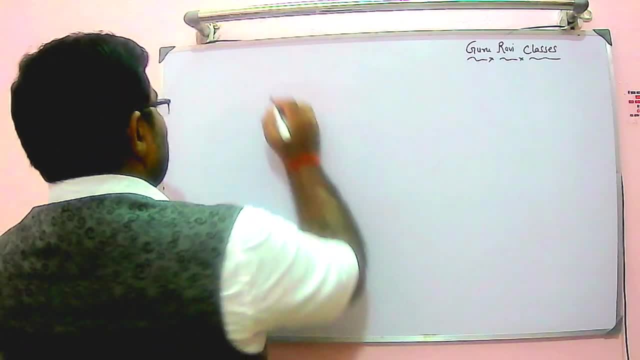 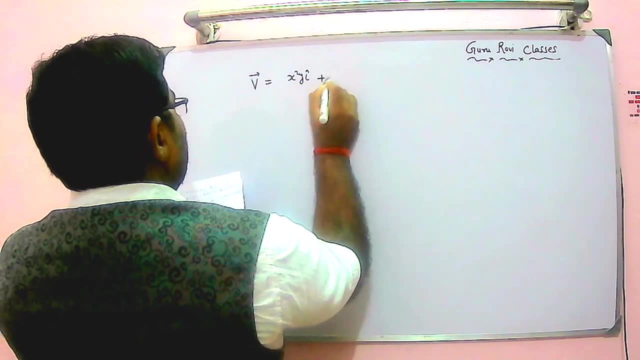 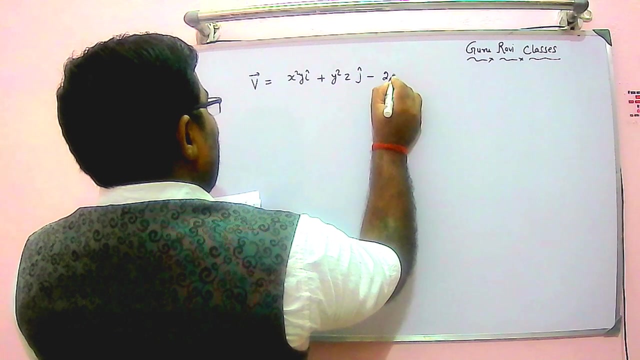 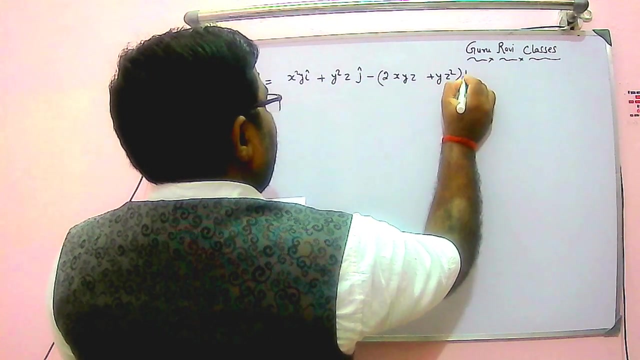 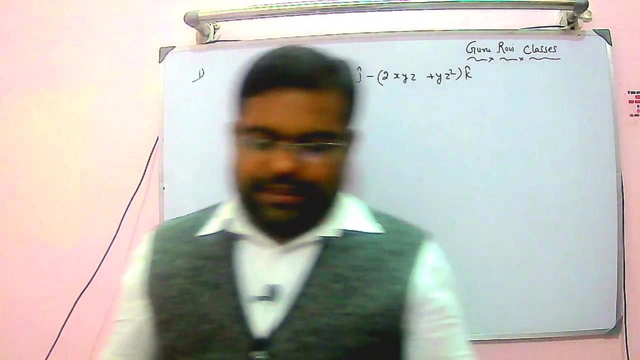 equation i am writing here. so this is the velocity vector which is given as x square y, i plus y square z, z minus 2, x, y, z plus y, z square k. this is the velocity vector which is given for the first numerical problem. proof prove that it is a possible case of steady, incompressible flow. this is the first segment. 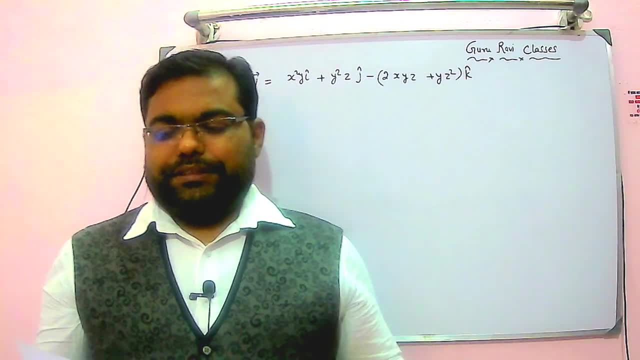 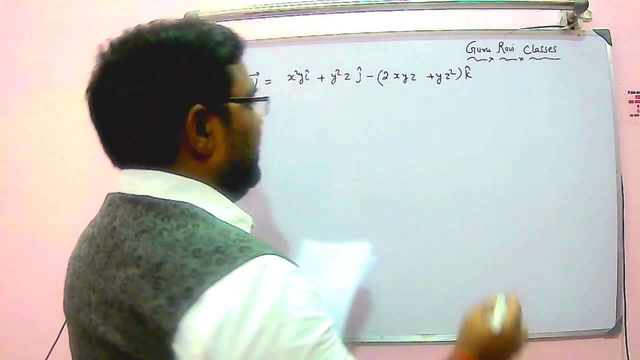 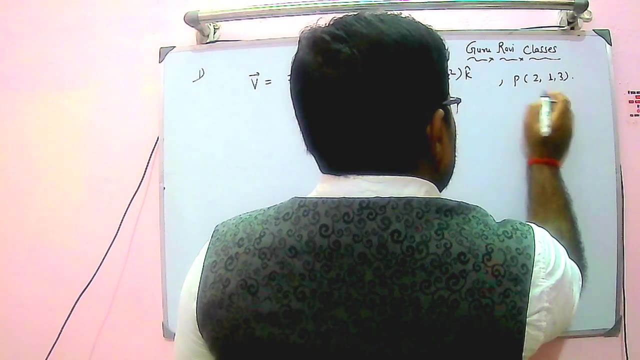 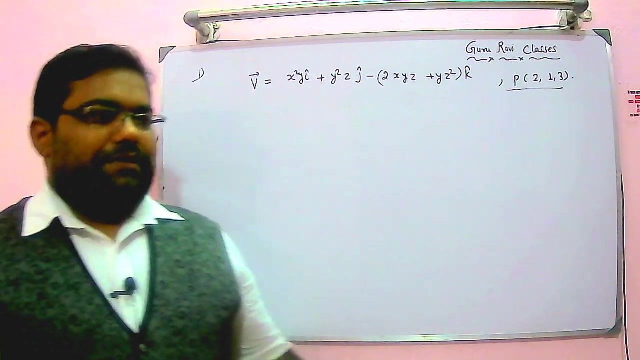 of the problem also make calculations for the velocity components at the point. at the point. one point is given: 2, 1, 3. so at this point we need to find out the velocity components. so i am repeating the problem right. the velocity vector for a given flow domain is given by. 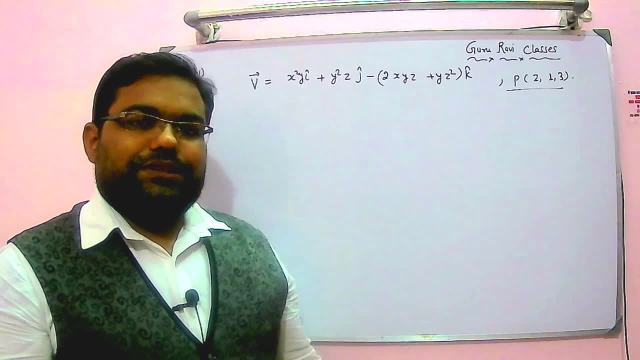 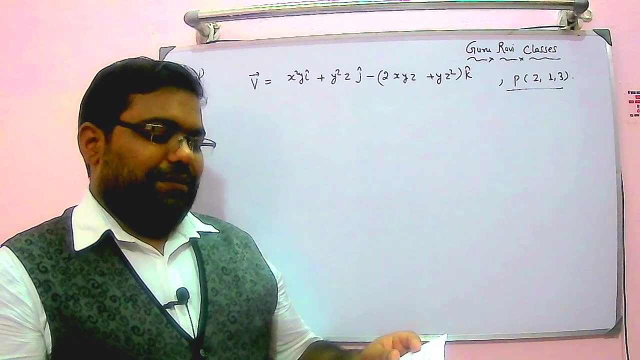 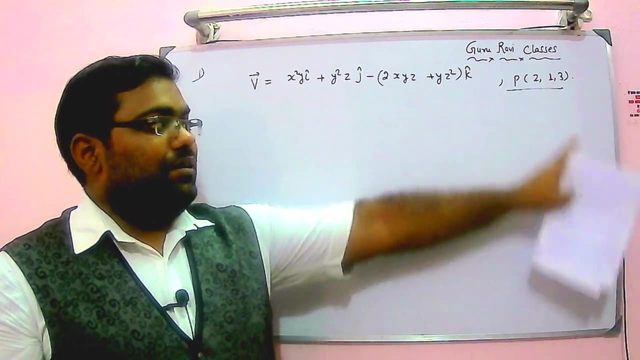 this equation all right, proof that it is a possible case of steady, incompressible flow is stopped. also, make calculations for velocity components. at the point 2, 1, 3, 2, 1, 3, x, y, z are given, those coordinates are given and at this coordinate right we need to find out. 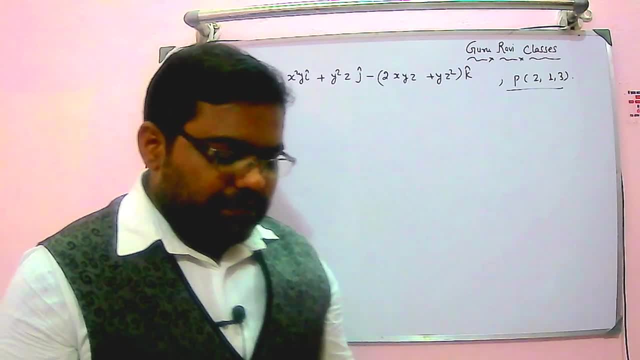 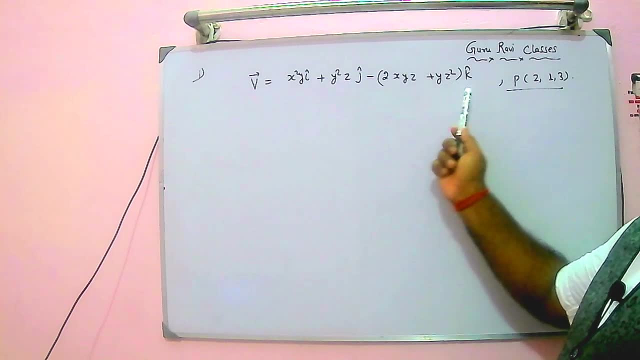 the velocity components. alright, this is the main thing that is given, the first number one thing. so how to approach that? so, if we look at this equation, nowhere time parameter is there. right, time is not given, so that means it is definitely a steady flow, right, steady flow, and is a three dimensional flow, because we are 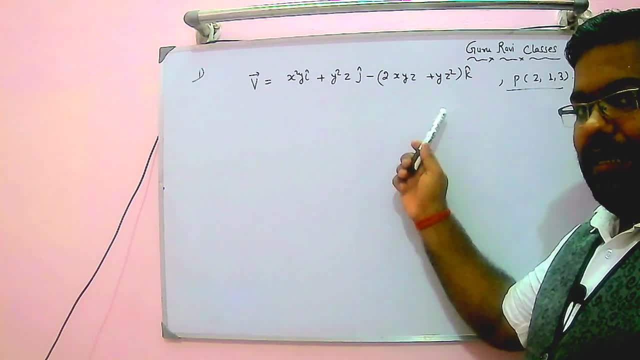 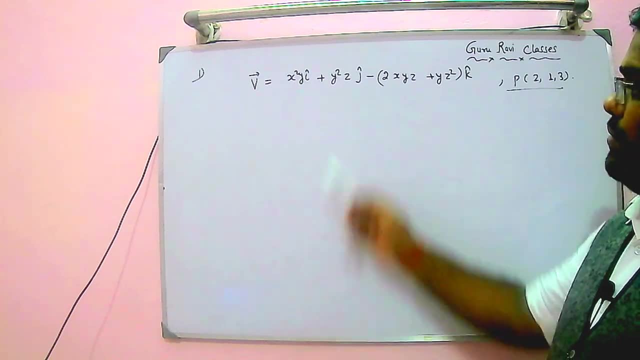 having X, Y, Z. you know these, all things are here. so this is basically a steady three dimensional flow, but we don't know what is incompressible or compressible. so look at here. density term is also not present, so it is an incompressible flow. 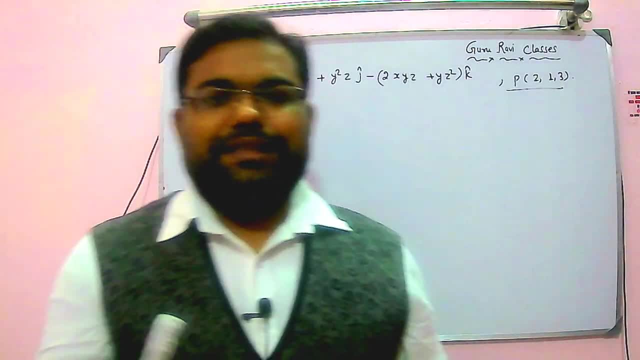 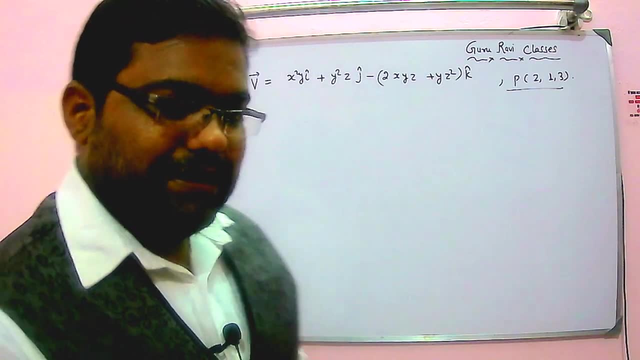 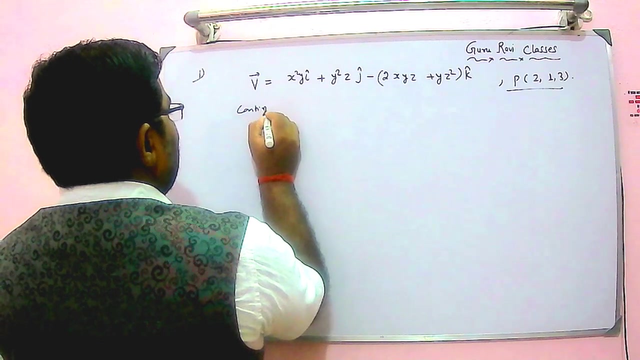 so we now know it is an incompressible, steady three dimensional flow. but we don't know whether it is possible or not, so we need to apply the continuity equation. that is divergence of velocity vector- right, it should be equal to zero, right? so so the continuity equation. continuity equation- divergence of velocity vector. 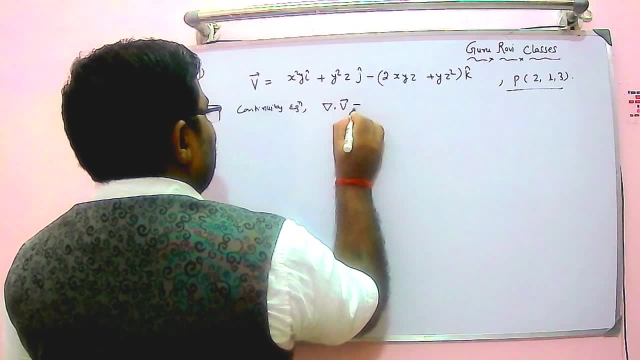 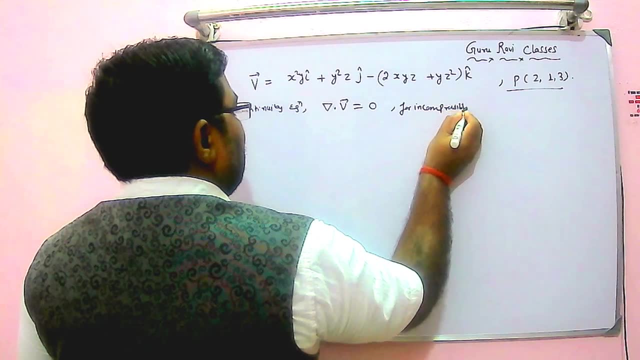 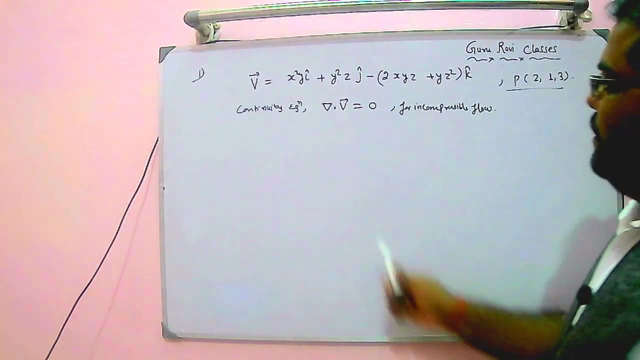 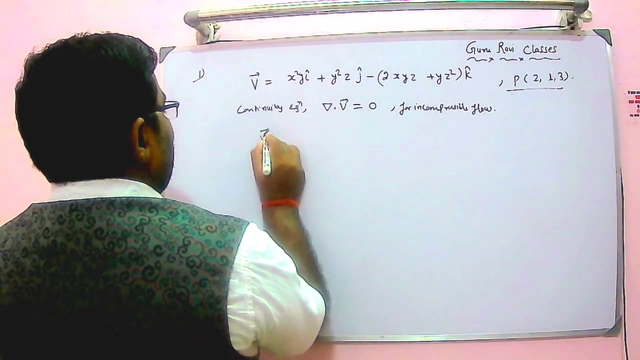 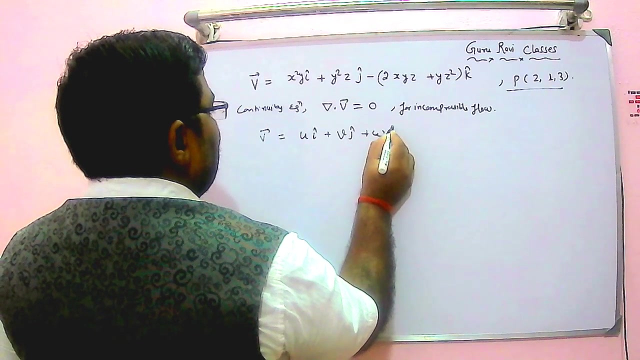 not curl dot. product of velocity vector should be zero for incompressible flow, incompressible flow. so we need to prove that right. divergence of velocity vector is zero. so if we look at these, this equation right, this equation can be comparable. like we can say, velocity vector is nothing but ui, vj and wk. so 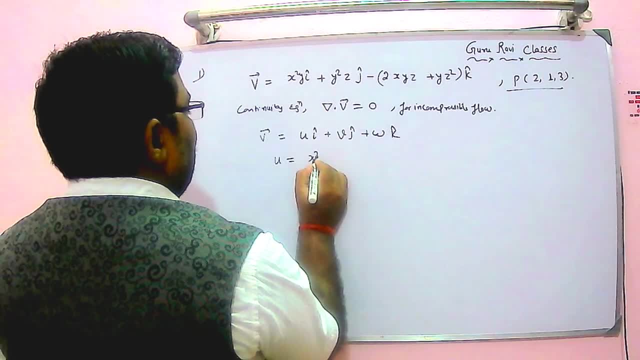 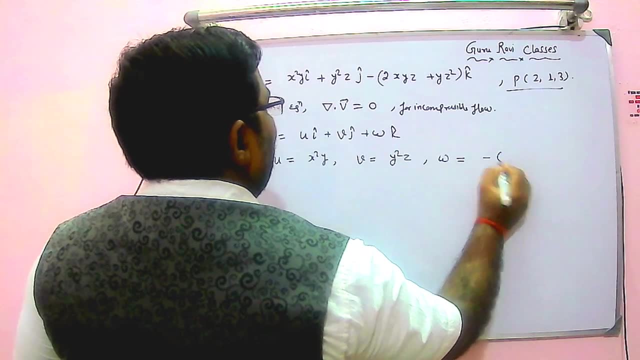 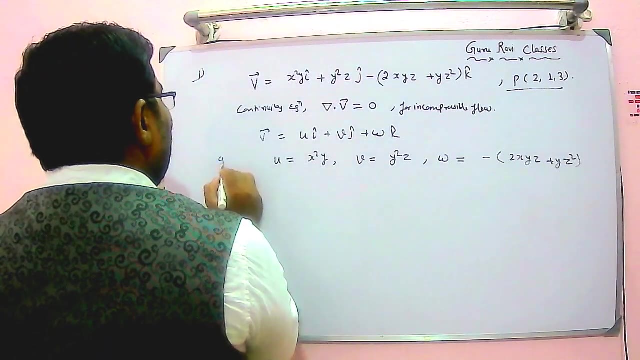 from here we can say: u is equal to x square y, v is equal to y square z and w is equal to minus 2 x, y z plus y z square. so this is basically given already. from there you can taken out. so: u x square y. 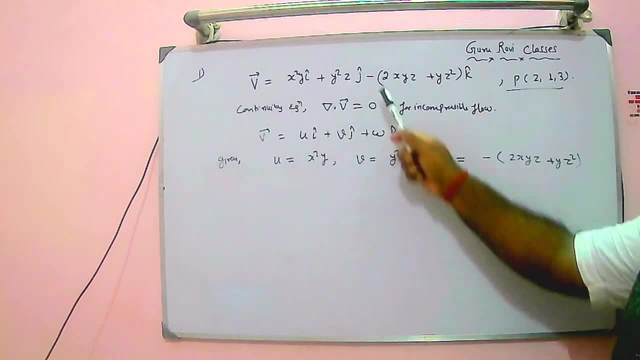 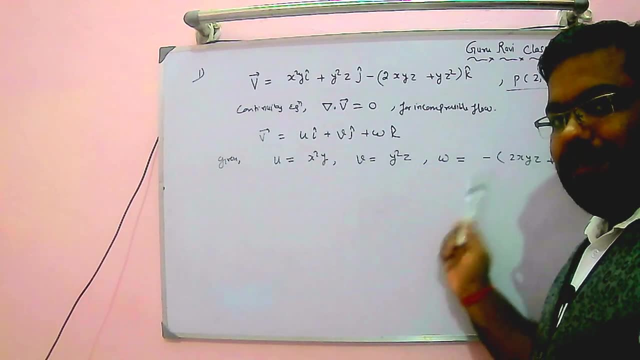 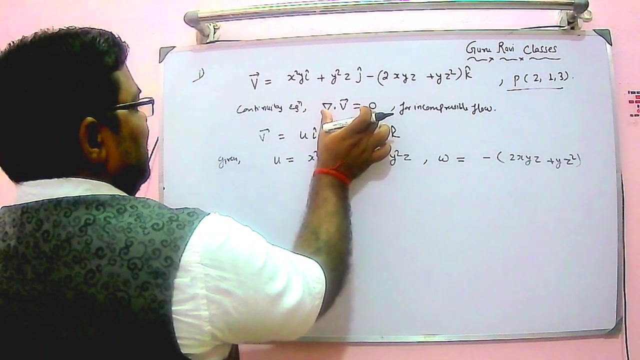 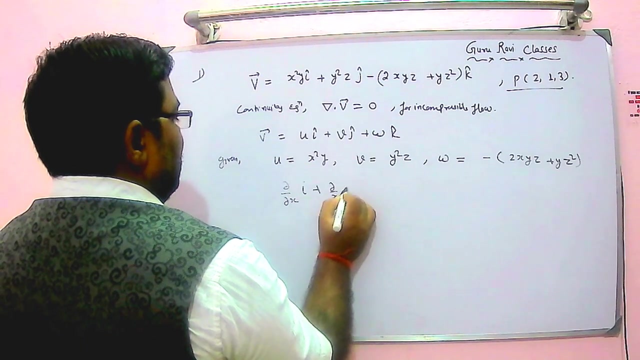 and v, y square, z and w. this complete thing is w. so these are the velocity components along the xy and is z direction directions. right Now, we will take the divergence of it when you are going for divergence of that if you expand this equation right? this equation can be written as: dou y, dou x, i, plus dou y, dou y. 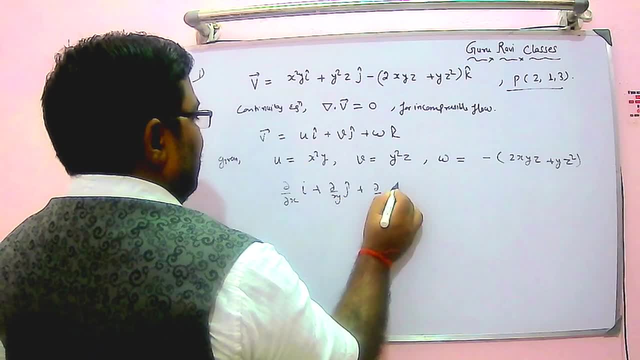 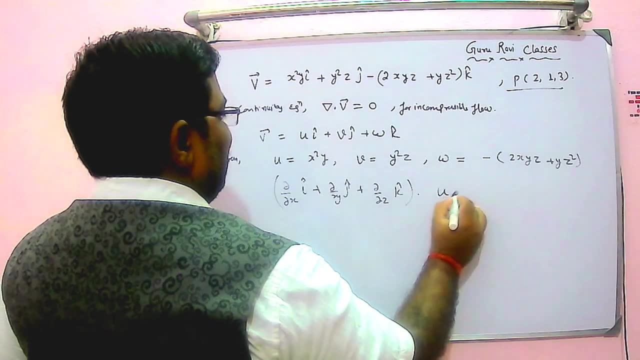 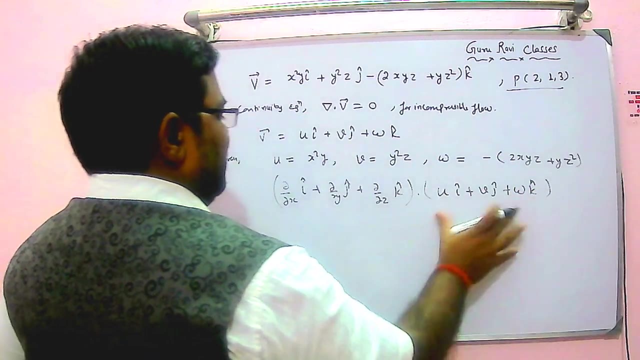 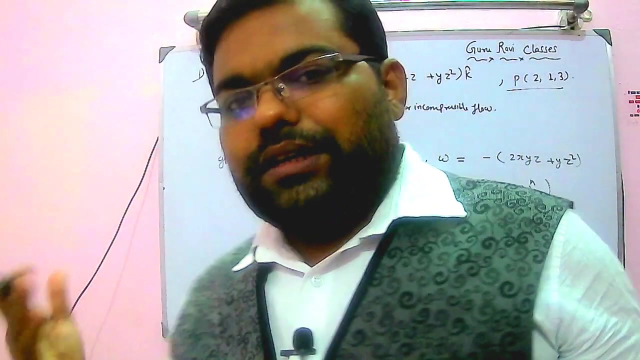 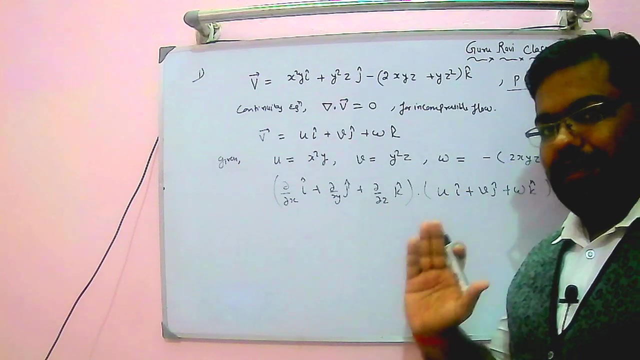 z plus dou y, dou z k right and into dot product of. I will just write ui, vj and wk right. if you just put the dot product of this, so i dot i will become 1 j. dot j also will become 1 k. dot k is also becoming 1, but i dot k is 0 j. dot i is also 0 j. dot k is also 0. 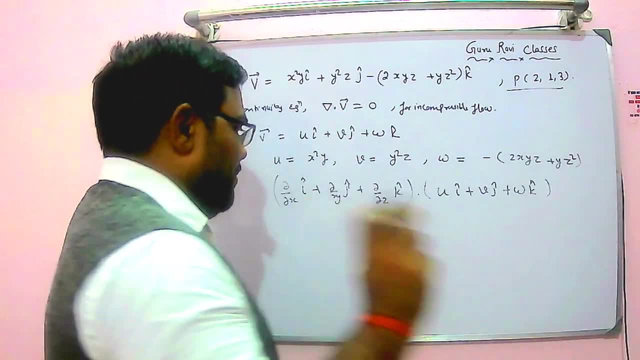 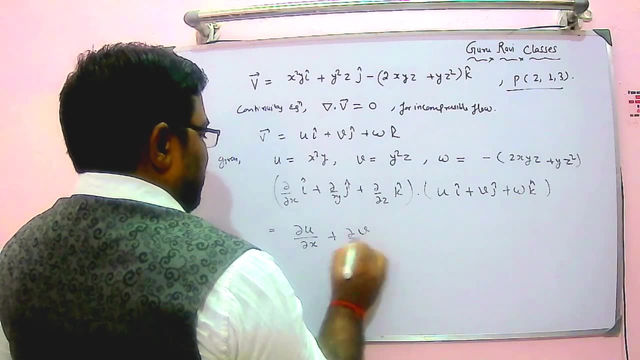 now only i dot i even same. you know, things will be equal to 1.. So if you multiply that, this will be simply: you will get one equation: dou u y, dou x plus dou v y, dou y. you will get one equation: dou u y, dou x plus dou v y, dou y, dou x plus dou v y, dou y. 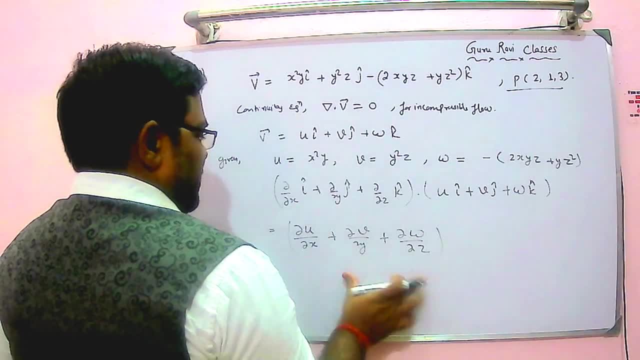 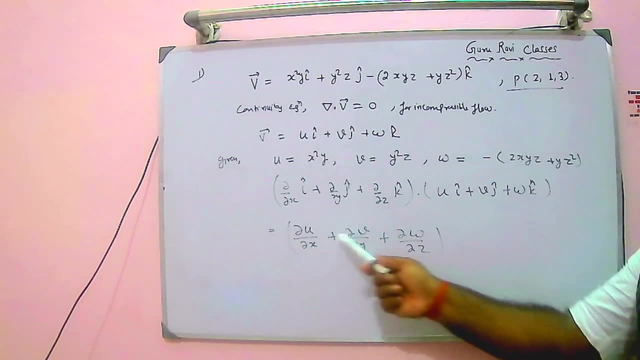 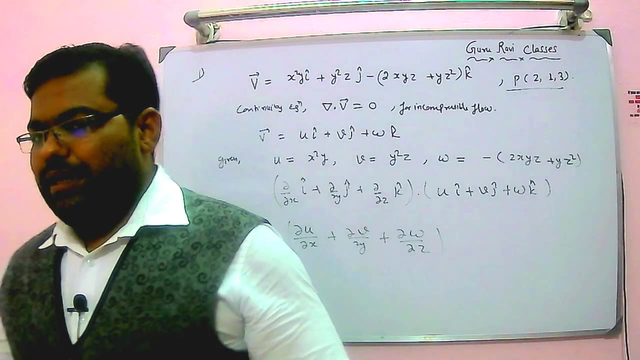 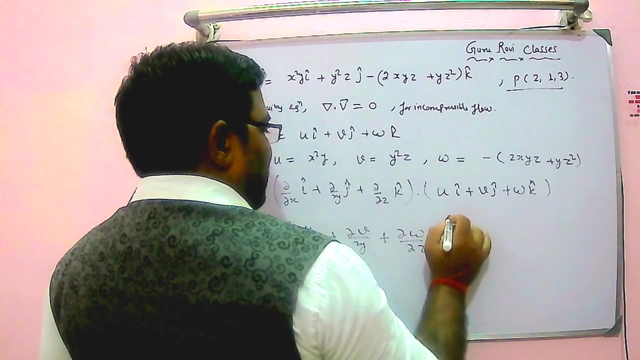 dou z. so this equation we are getting, and we need to prove that this component, whatever partial differential equations of u v, w, this should come equal to 0. that is our requirement. so now we simply differentiate, right, the velocity components. so velocity components are here, right. so i will take 1 y, 1 here. so dou u y, dou x. we need to find out. so. 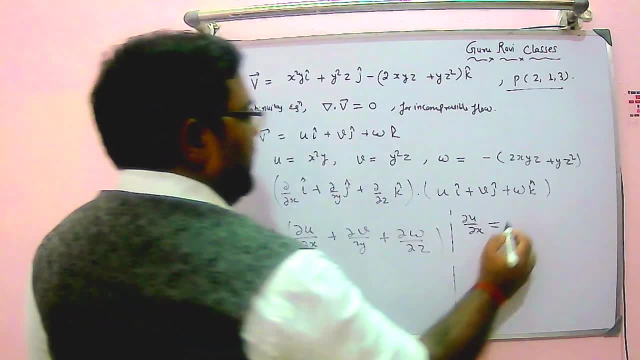 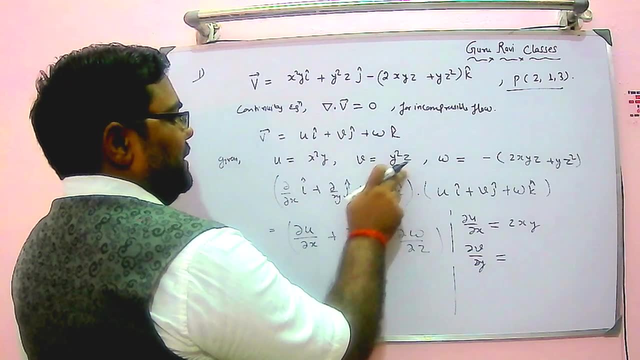 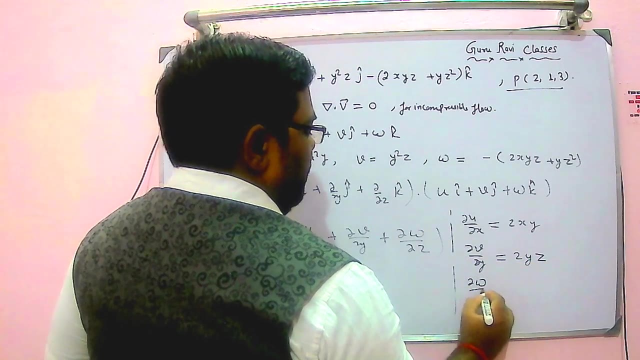 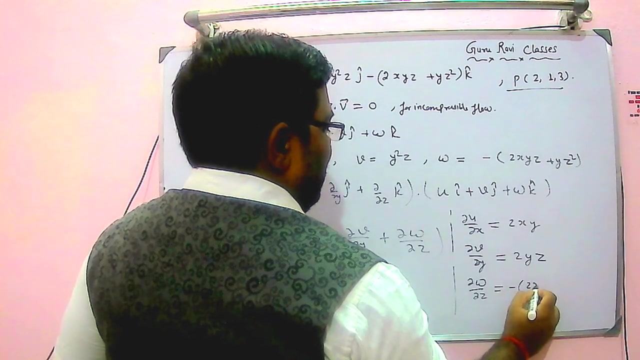 is here. differentiate with respect to x. i will get 2 x y, 2 x y and dou v y, dou y. right, if you differentiate this equation with respect to y, you will get two times of y z, then dou w y, dou z. we need to differentiate this equation with respect to z. i will get minus 2 x y, plus 2 y z. 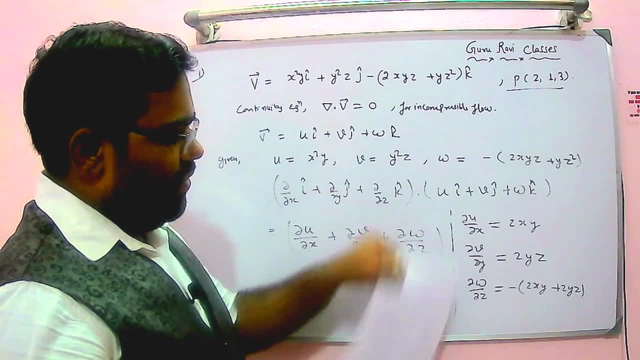 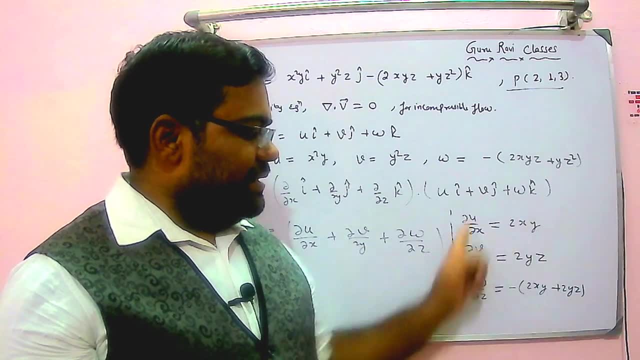 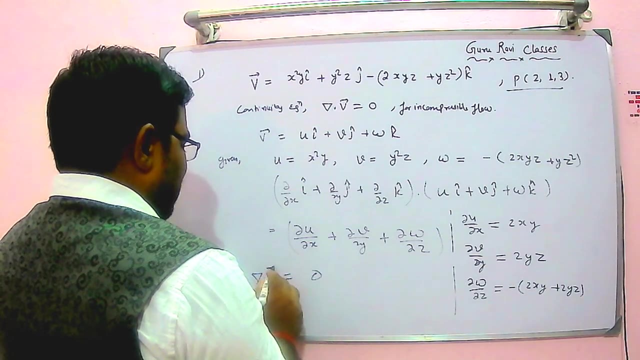 just look at if i add these all right from here, we can see if we add 2 x, y plus 2 y, z and this, everything, this is becoming zero. basically so when we substitute these all things here, we are getting this equal to zero. so that means divergence of velocity vector. 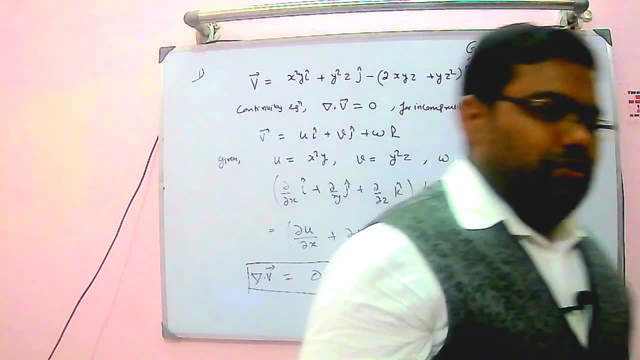 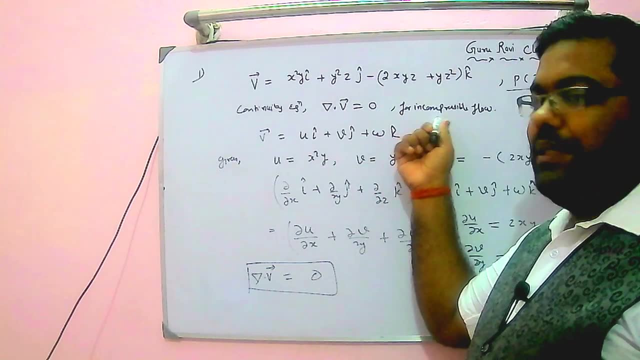 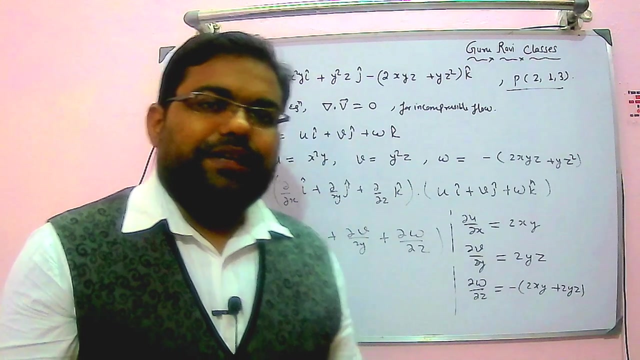 is zero, basically. so it is going to be zero. that means what divergence of velocity vector is zero. so it is a possible case of incompressible, steady, three-dimensional flow. right, so it is a possible case of fluid flow because it is satisfying the continuity equation. is satisfying the continuity equation, so it is a possible case of fluid flow. 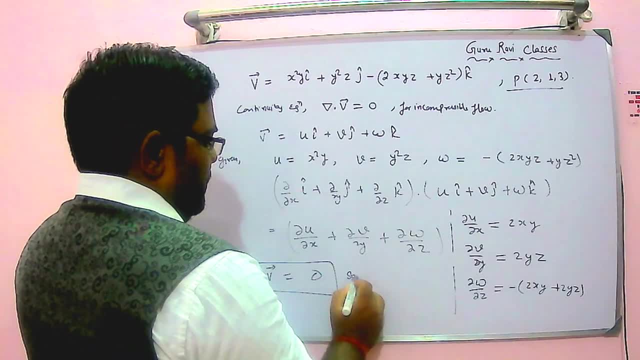 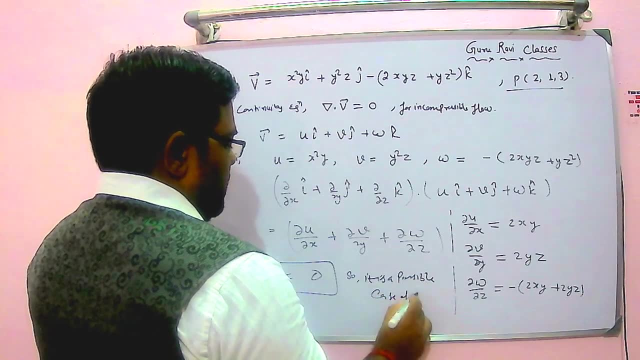 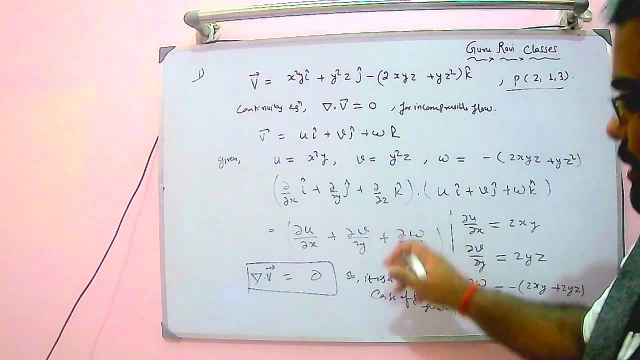 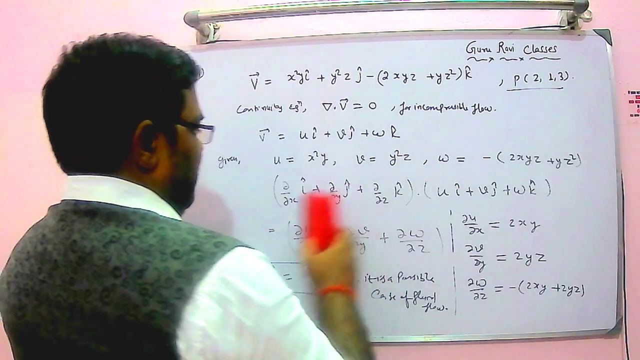 so one thing is over, right, so we can say: so, it is a possible case of fluid flow. okay, this is over, so one part is over. now we will go for the second part, which is talking about the velocity right vectors at this point. so I am raising this, so if I raise this, I will. 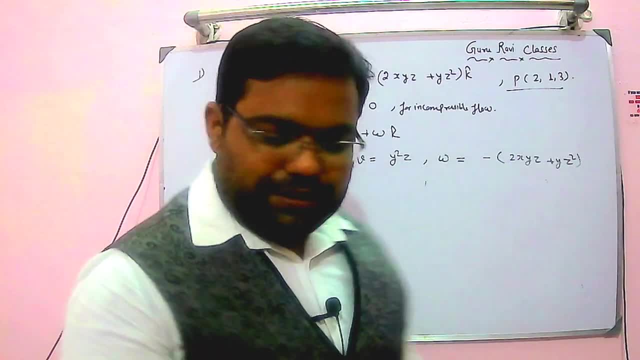 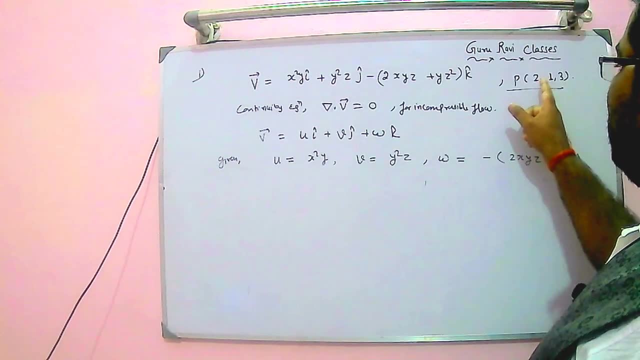 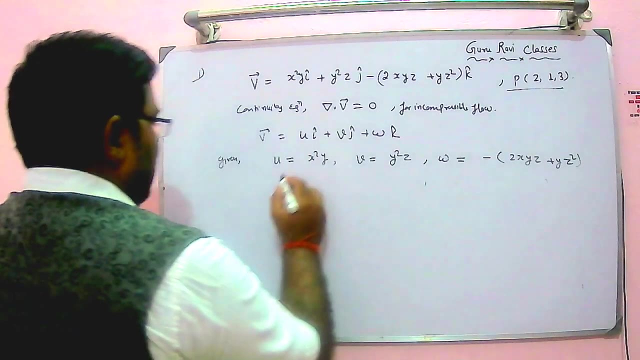 come to here. so velocity vectors, velocity components, are here right, which are given u, v and w. these are given right. so just have a substitute value of x, y, z, x 2 and y 1 and z 3, just substitute here, right? so if you substitute here u will become x, that is 2, square into. 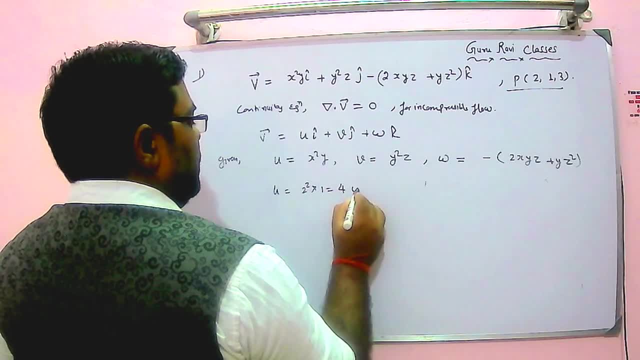 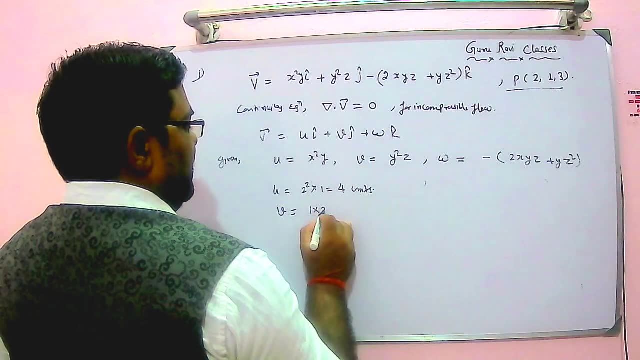 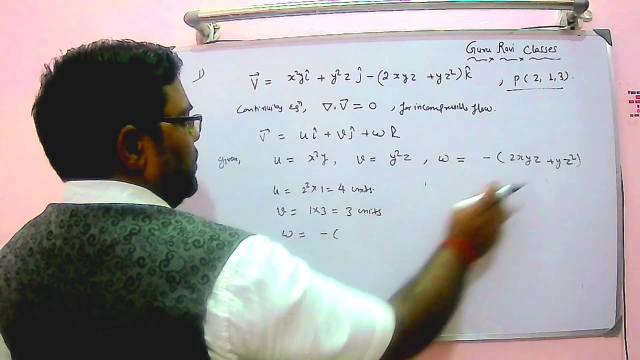 into y, 1, that is 4 units right, and v, this y square is 1 and z is 3, that has become 3 units right and w. w is minus 2, x, y, z, so 2, 3, 6, 6, 2. 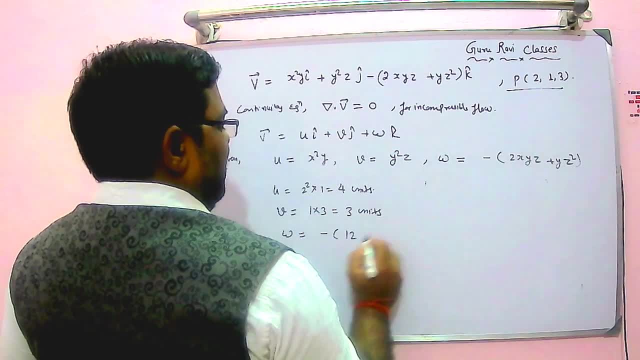 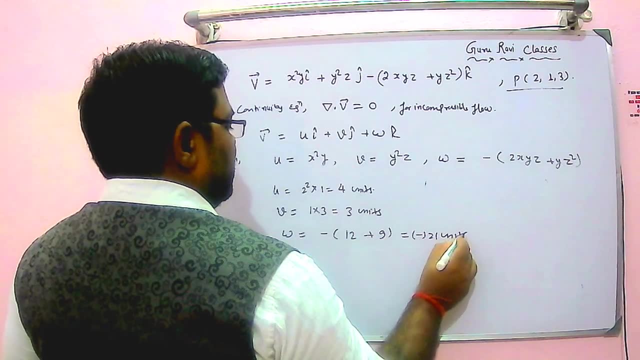 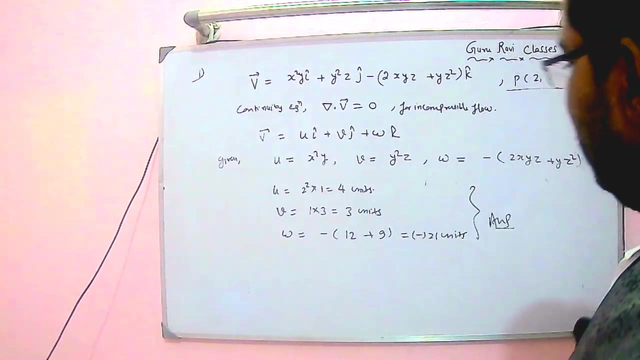 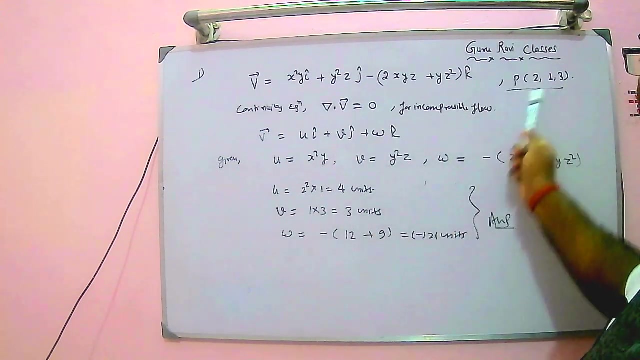 right here: 6, 12 plus 9, right. so this is becoming minus 21 units. so these are the answer. so velocity component at point p can be calculated in this way. so just substitute the value. so I substitute value of x here, this is becoming 4. and put y and z value here, this is becoming 3 and then minus. 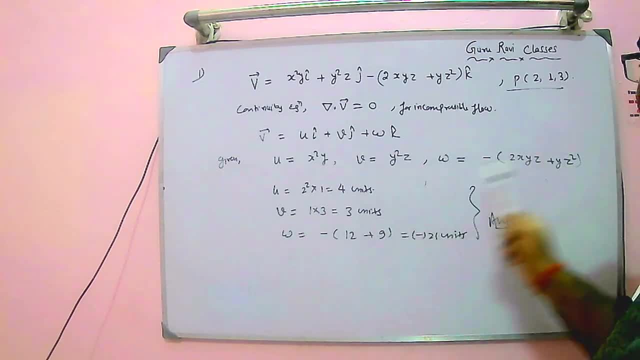 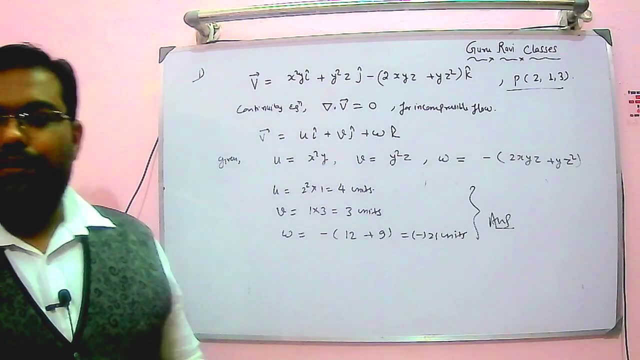 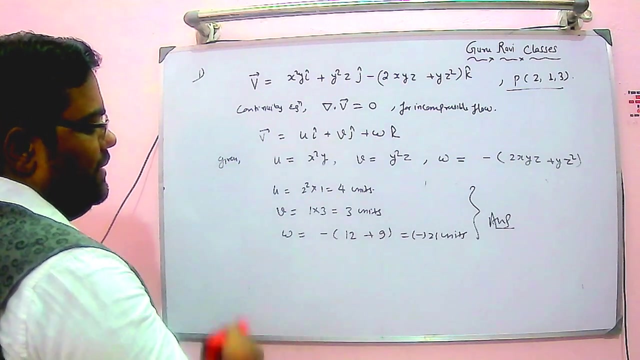 time times of x, y, z. everything is this is 12 and this has become 9, so 21 units. so like that, you can solve this problem. this was the first problem. very straightforward problem, easily you can find it out. so let's go for second problem. I am raising this. these are the answers: 21 units. let's go for the second. 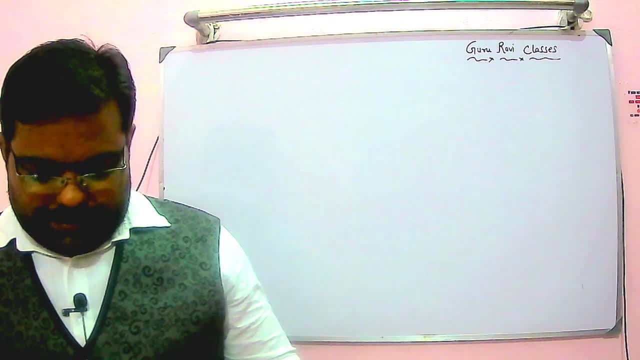 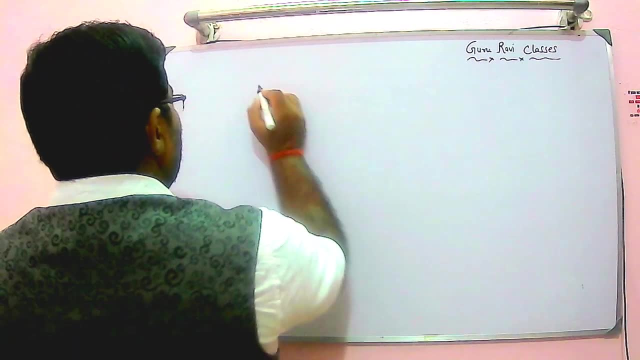 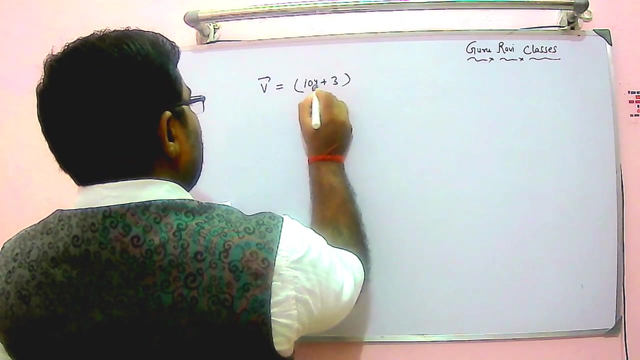 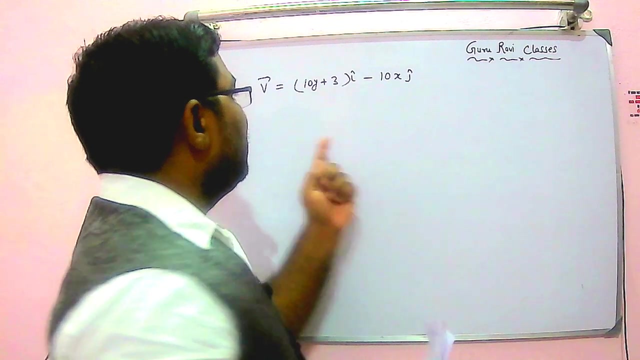 numerical problem. so second numerical problem is saying that if velocity vector for a given flow domain is given to a given flow domain, then the velocity vector for a given flow domain is given by this equation. this is the equation: 10 y plus 3 i minus 10 x, z. this is the velocity vector. 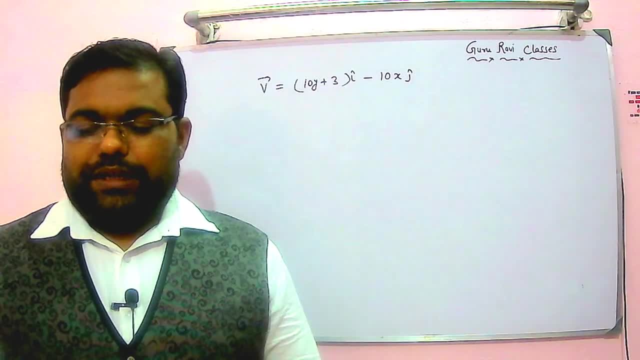 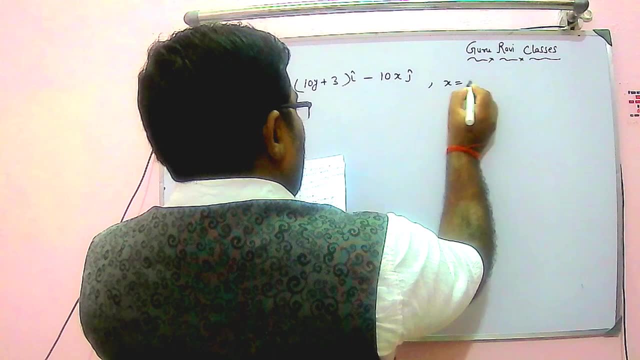 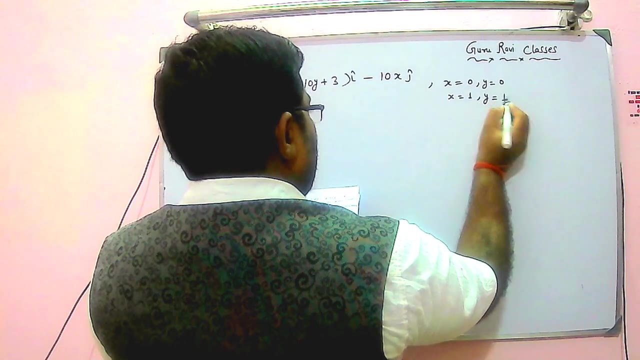 which is given all right, determine the circulation around the contour given by. a contour is given by: x is equal to 0, y is equal to 0, y is equal to 1, y is equal to 1. these are the quantities given for the contour. so it is asking. 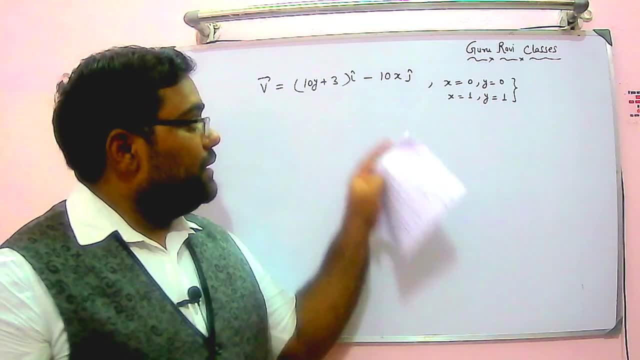 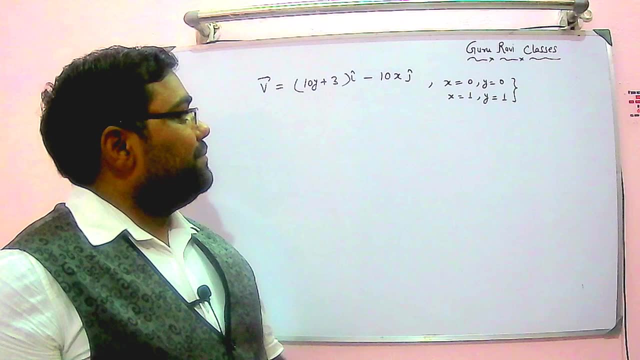 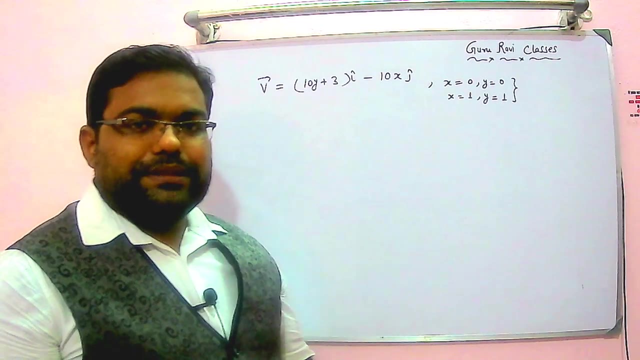 about this is the velocity vector, which is given right, and we need to find out the circulation around this contour, how to solve this. so look at this equation. basically, this equation is a two-dimensional case of fluid flow where u and v are given right, basically. so we can simply say: 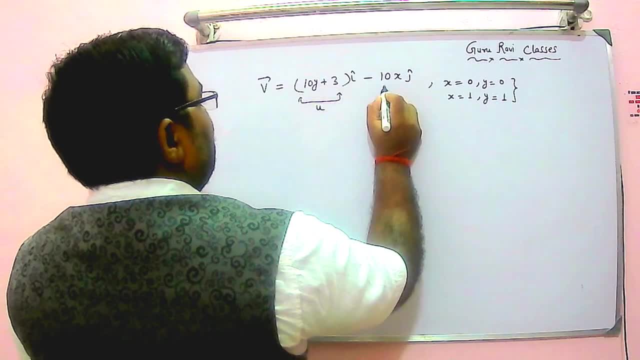 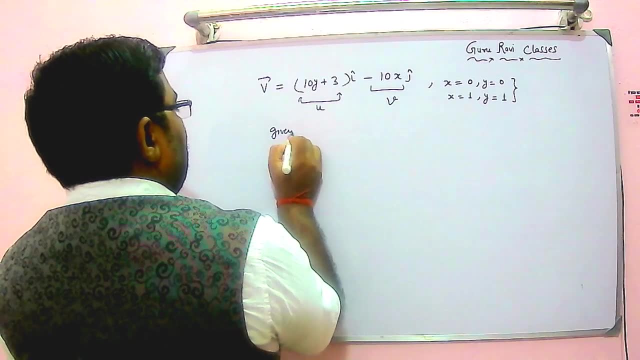 this complete thing is small u and this include minus like a, v. So in the incomprehensible state v times v we see u has a total weight of 3rea. so this is the velocity vector which is given by a given flow. so we can say u is equal to z here that means v is igual to minus. 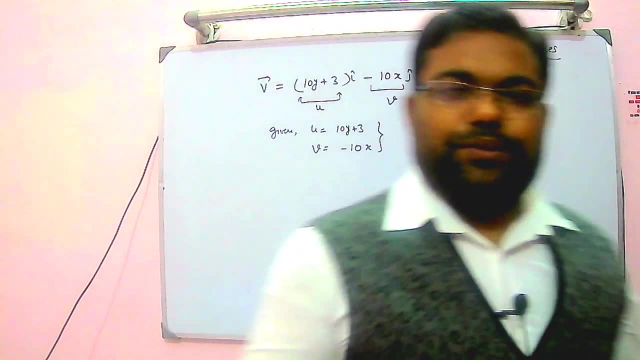 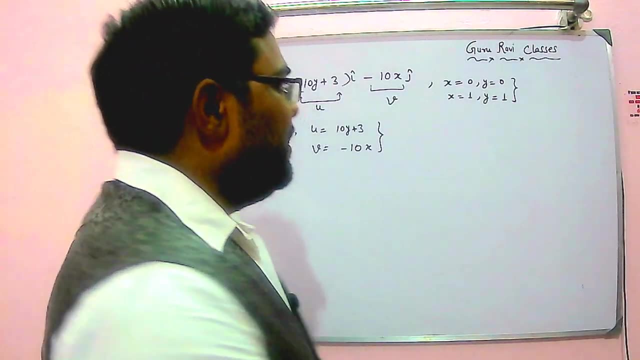 z. if z is in finans X required, then u is equal to z, the value of vector x is equal to z, Y is equal to negative z and yourبة white square root over z is our vector xz, priest first, will be equal to minus z. this will be your vector. x will be the vector z and ring headlights will be zerosfeito. 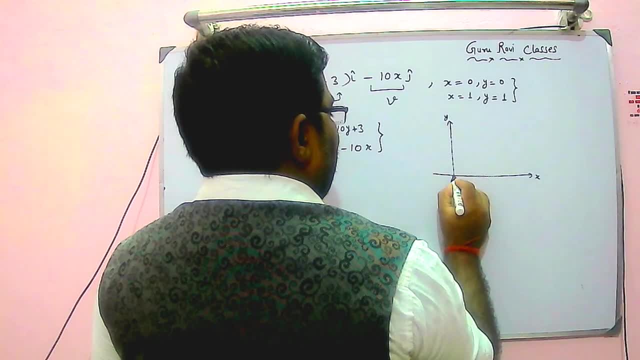 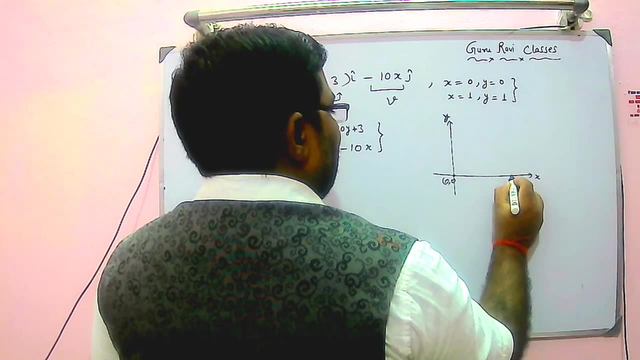 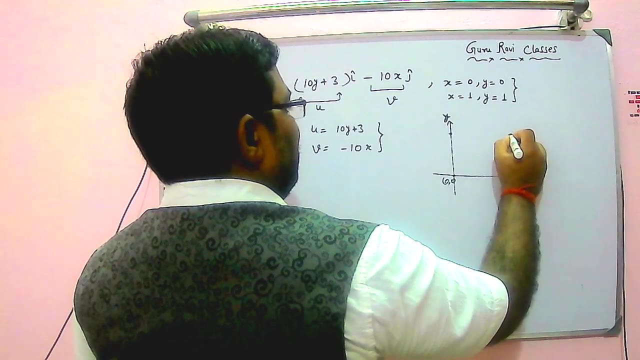 I and there is is a y. first point I am getting here which is 0, 0 right. when x is becoming 1, y is becoming 1 and similarly, if you look at y, is also becoming 1 right. so I can get here one point and then 1 and 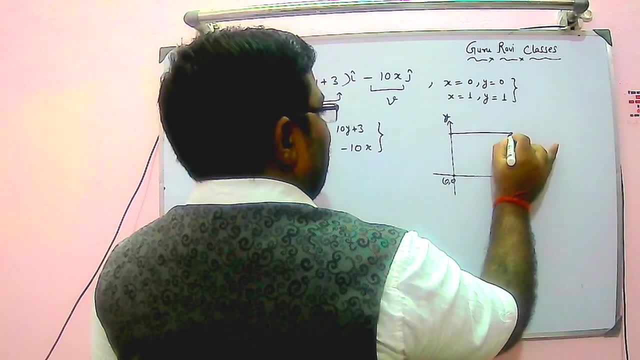 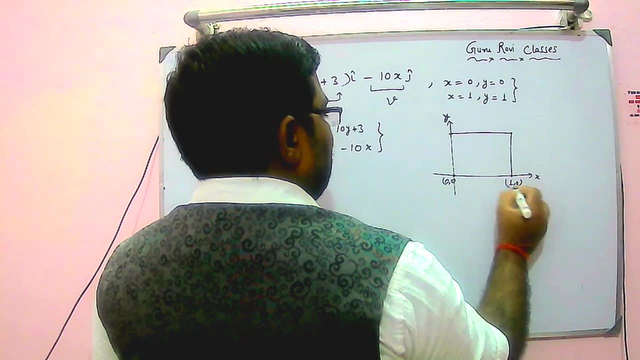 1, which I will get here. so this is becoming this kind of you know square, kind of you know structure. I am getting so 0, 1, then this is 1, 0, this is becoming 1, 1 and this is becoming 0, 1. so I got. 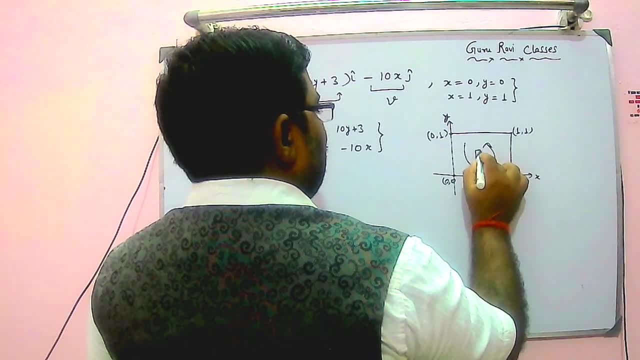 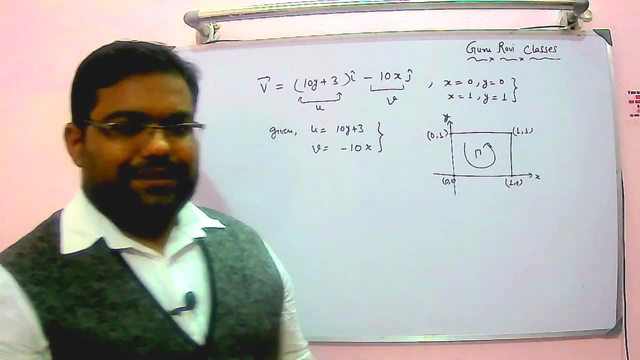 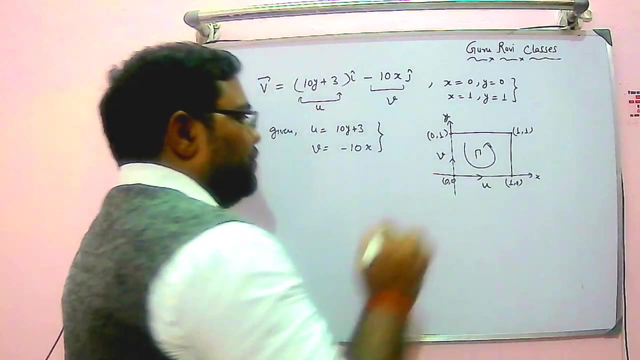 this one and we need to find out the circulation around this. so circulation is given by this symbol. tau tau is saying me the circulation. so I can say this is u right along x, is u along y, it is v, so u and v. also I have written. 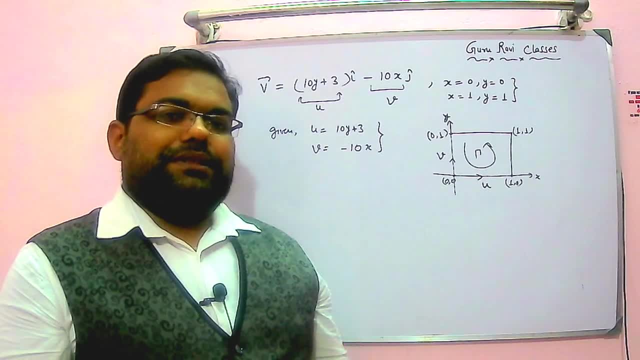 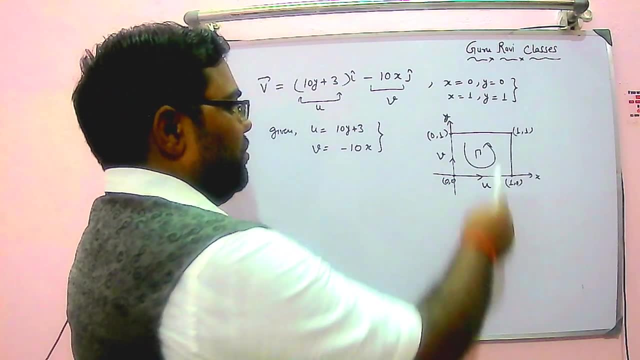 So what is the circulation definition says? circulation definition says that it is the. it is the line integral of tangential component of velocity taken around any closed curve. this is a closed curve, basically right. so starting from here and going like this, and we need to find out, 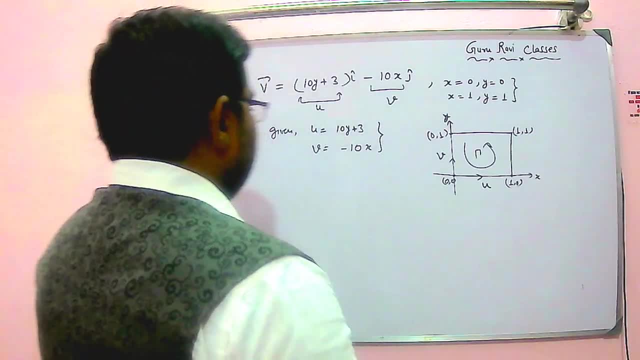 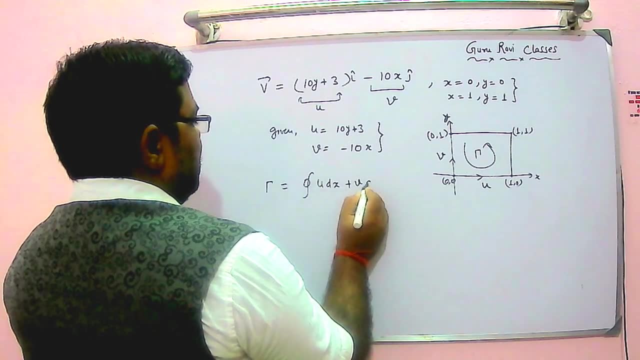 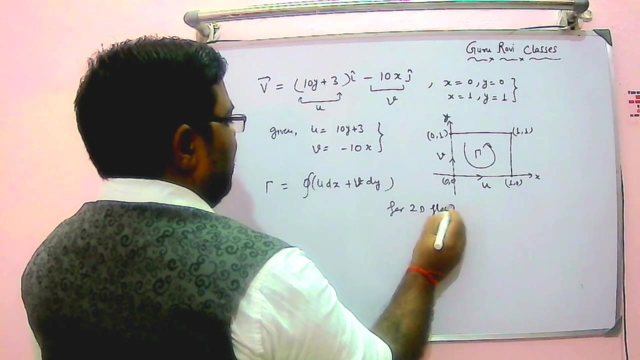 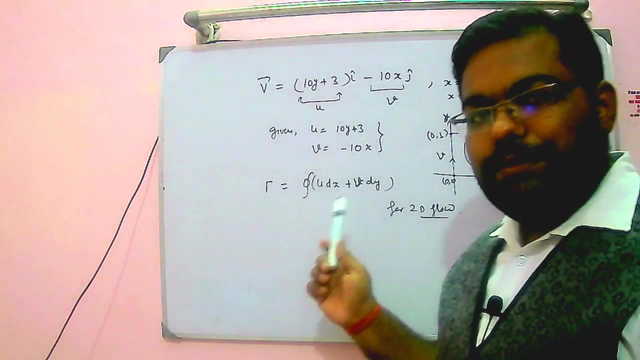 the circulation for it. so how to do that? so circulation is nothing but cyclic integration of u dx plus v dy. this is v dy 4, two-dimensional flow. and given, you know, velocity vector, is the velocity vector for a two-dimensional flow. Clear or not, It is for two-dimensional flow. 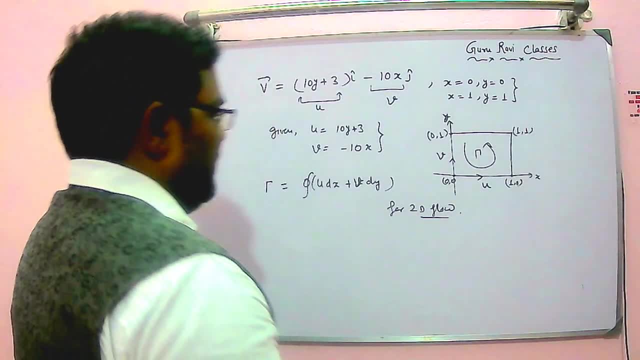 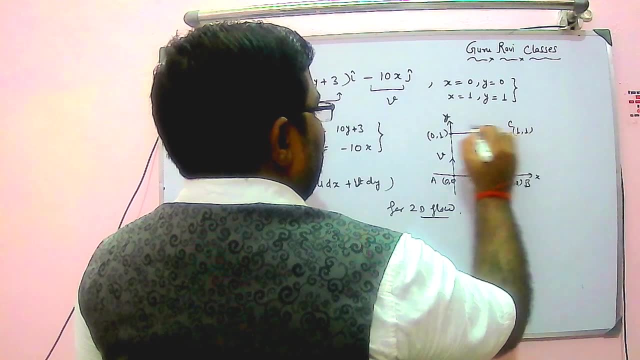 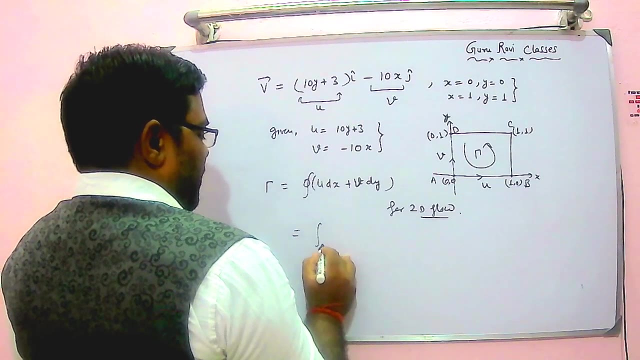 Now how to write that. One thing First is this, So I can say this: A, this is B, this is C and this is D. if I say So, I can say, like cyclic integration: along AB, Along AB. only U is there. 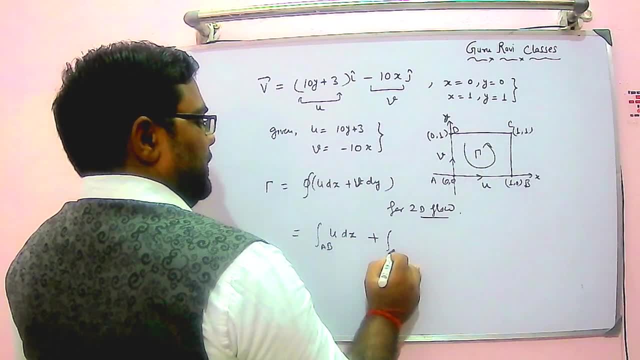 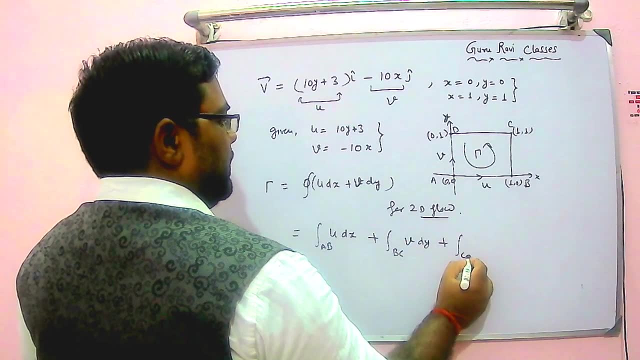 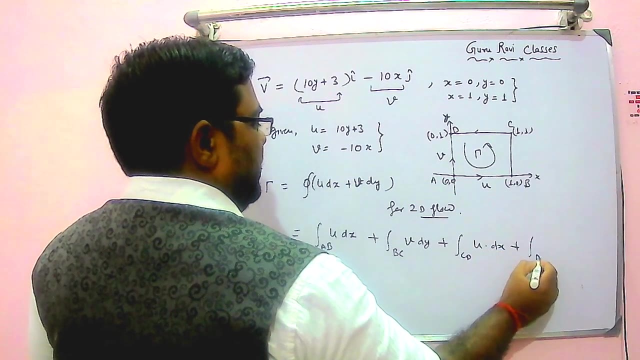 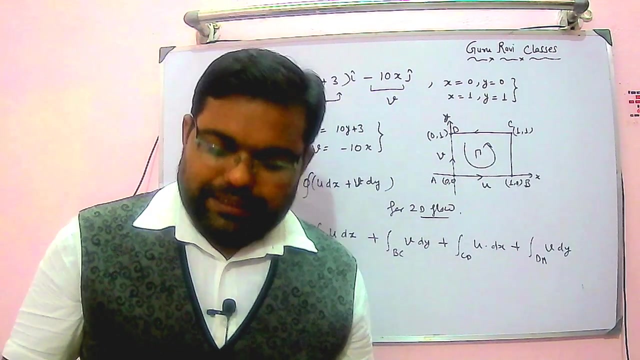 U DX Along BC. here only vertical component is there. VDY Along CD. again U will be there right U into DX and along DA here VDY. So sign convention. we will consider as per the limit When we are putting the limit and as 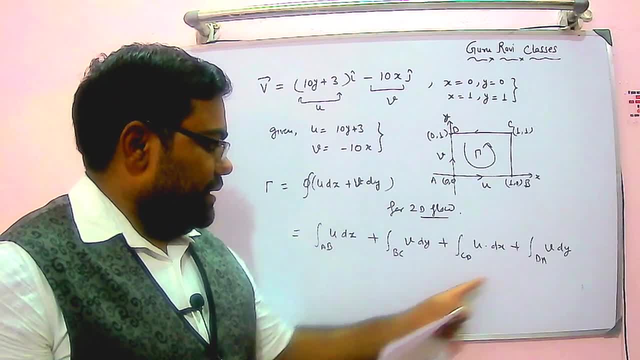 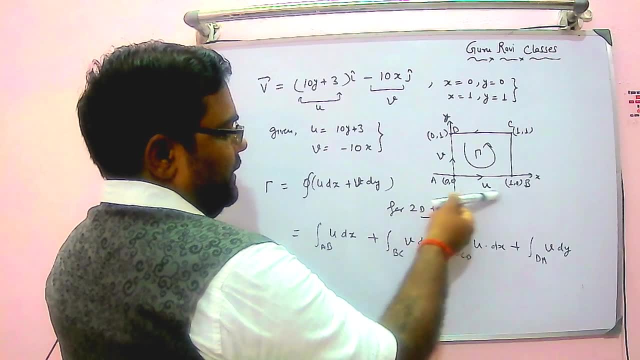 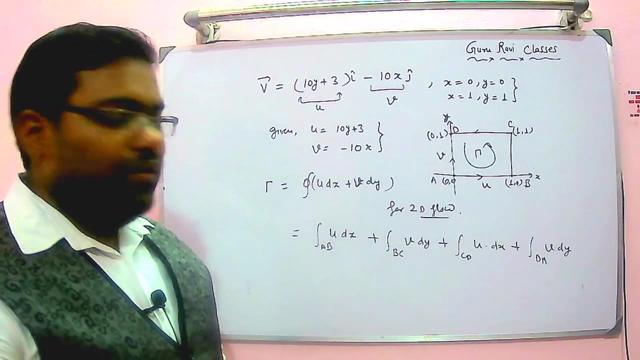 per that sign convention will be considered. Just, we have seen here AB, BC, CD and DA. Now, at this point, what is the value of Y? Y is 0, only X is equal to 1, right X is equal to 1.. 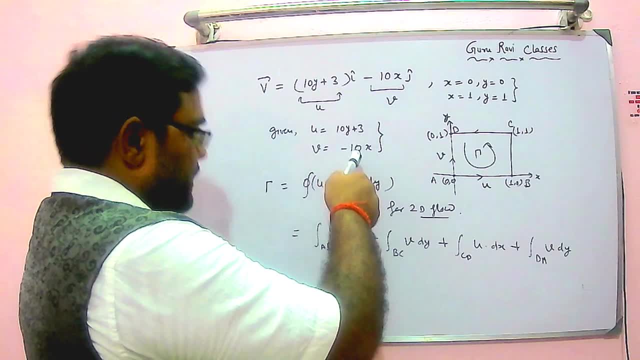 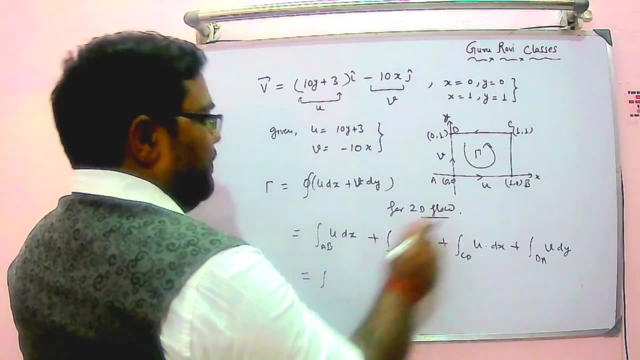 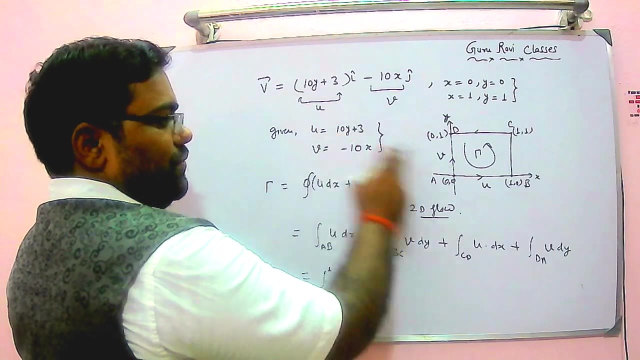 So look at the U equation: U is here, right, U is here 0. That means U is equal to only 3, which I am getting. So I can say here: and limit 4X is equal to 0 to 1.. So 0 to 1 and U value is only 3, because Y is 0 here, right? So 3, DX. This is the first. 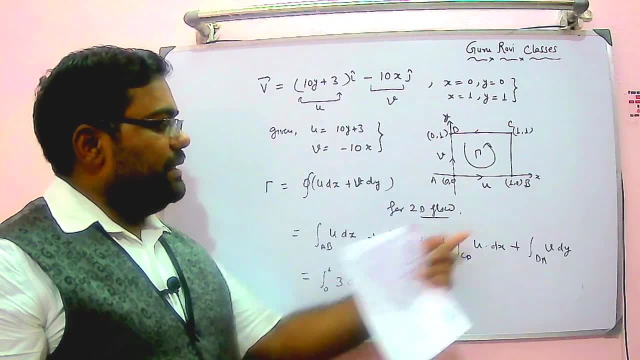 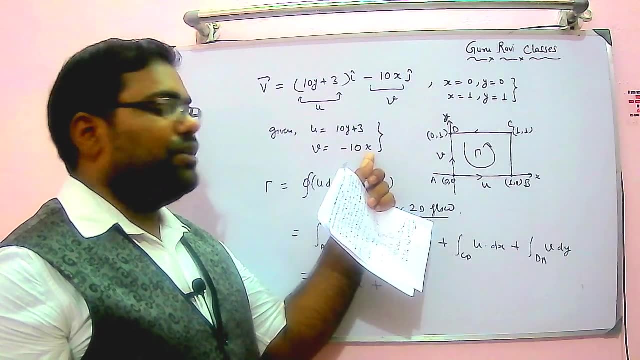 term which I can write. Second term for BC, which is here, Here, only V component will be there: vertical component velocity which is minus 10 times of X X value. here X value is equal to 1.. So if you substitute X is equal to 1, I can get velocity is: 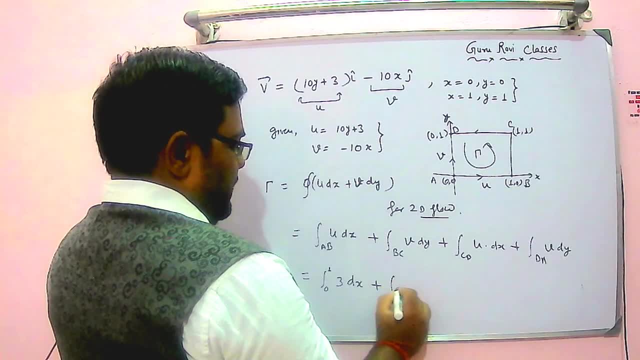 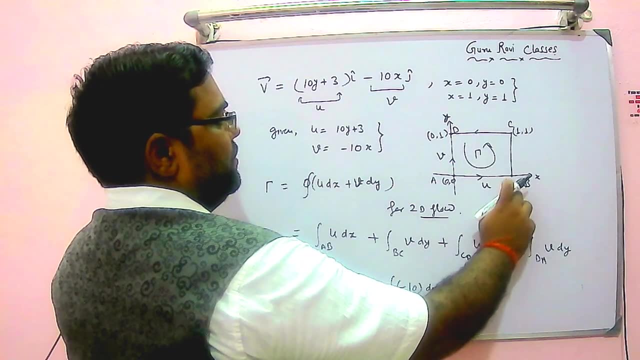 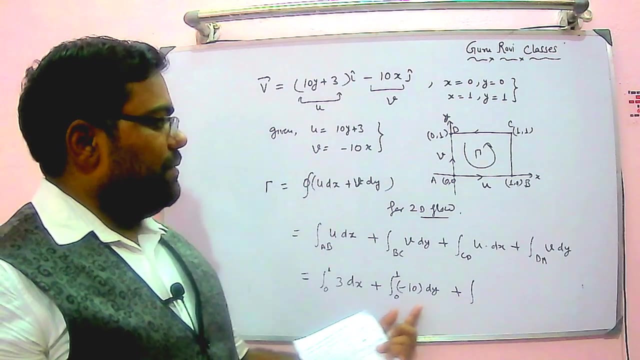 equal to minus 10.. So integration minus 10 DY. What is the limit for Y along this, Starting from 0 and going to 1.. 0 to 1 plus 2. I have written, Now I have to write here Along: this only U is. 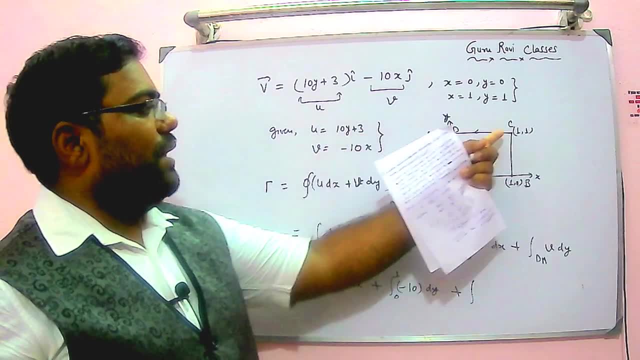 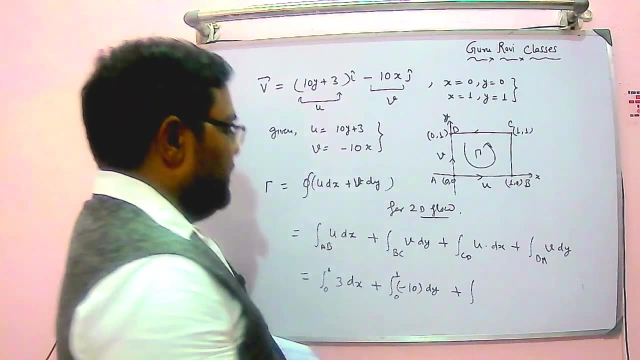 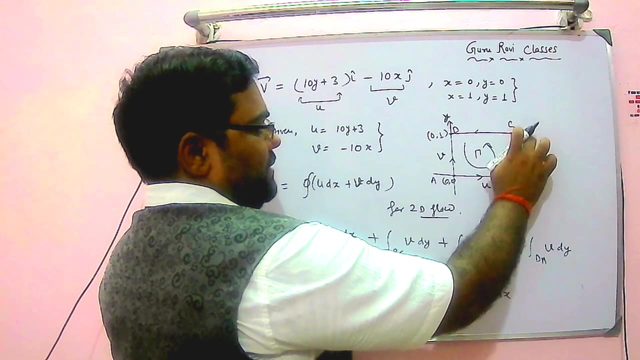 there. So U equation is 10Y plus 3.. What is the Y? This line? Y is equal to 1.. Clear or not? If you substitute Y is equal to 1, this will become 13,, right, So 13 DX. What is the limit for X? It is going from 1.. X is 1 here. 1 to 0 plus Now. 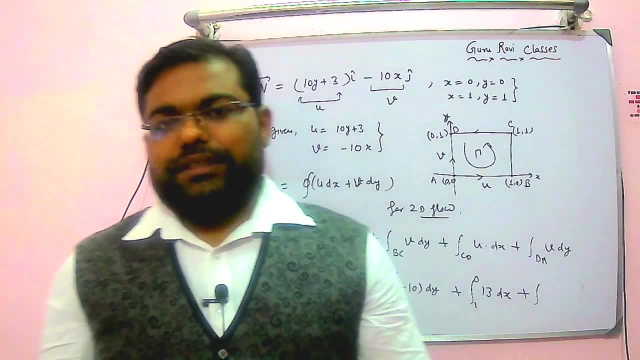 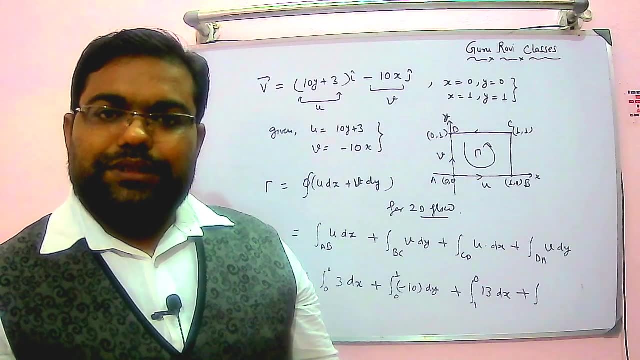 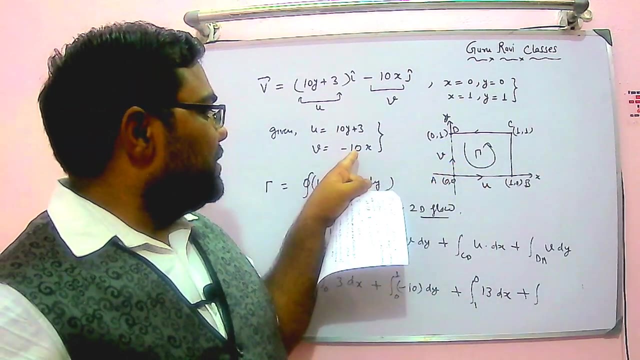 along this. DA, DA again. velocity is V right. V is minus 10 times of X. What is the X here? X is 0.. X is 0 here. What is X here? X is 0.. So when you put the X is equal to 0, velocity will become 0. 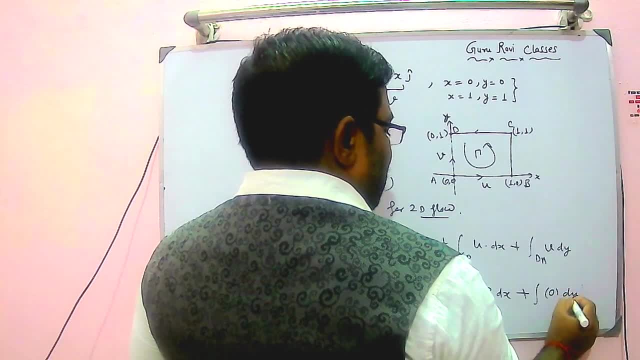 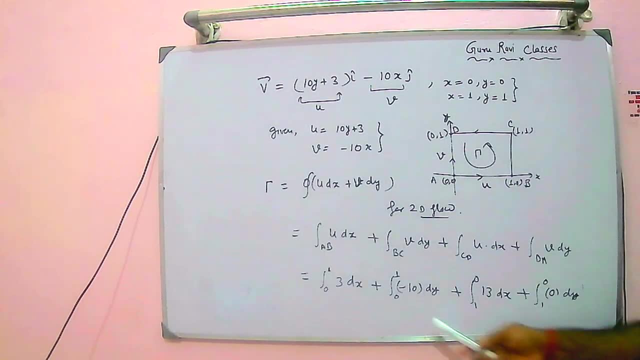 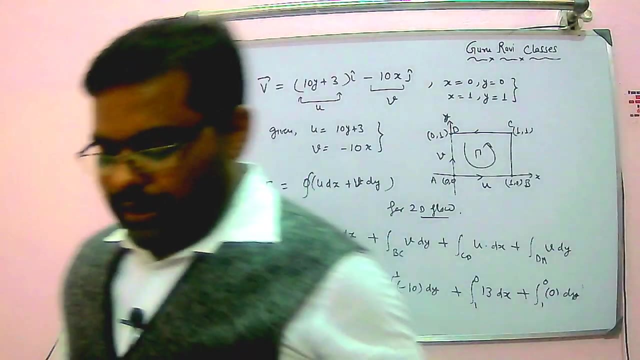 So 0 DY limit again by 1 to 0.. 1 to 0.. Clear Now. just you have to integrate these 4 things right- 1,, 2, 3 and 4- and you will get the answer. So integrate 1 by 1.. So this become 3,. 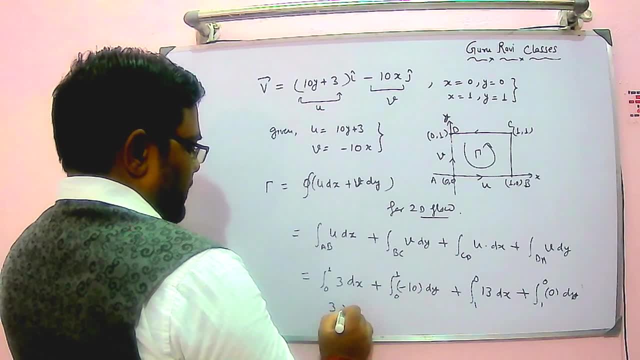 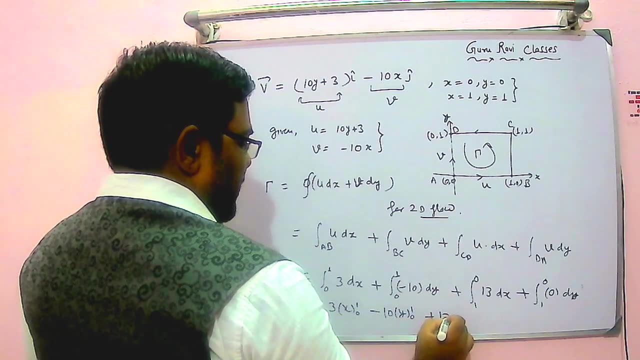 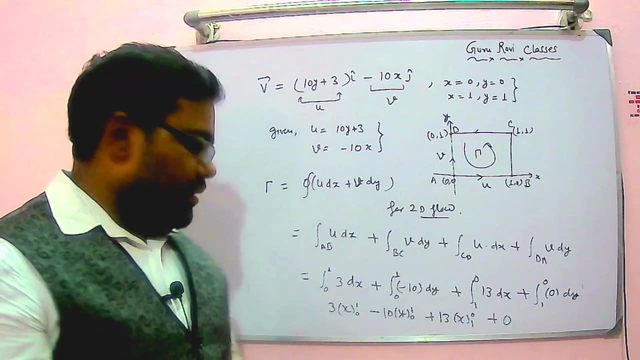 X, So 3, into X X, 0 to 1.. This is become 10Y 0 to 1.. This is become again 13X, 1 to 0. This is becoming 0. This is 0. There is no meaning of it. So, if you solve this, if you solve this, 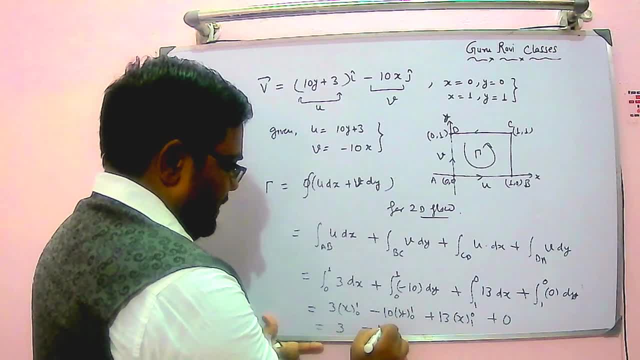 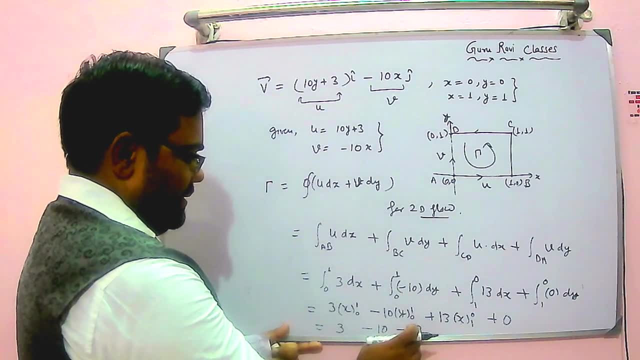 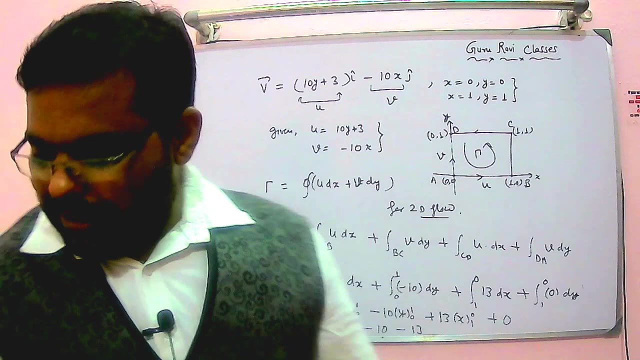 this will give just simply 3, right. This is becoming 10 and this is becoming basically minus 13.. So if you add this, this become 23 and plus 3.. So I can get minus 12, right. So I can. 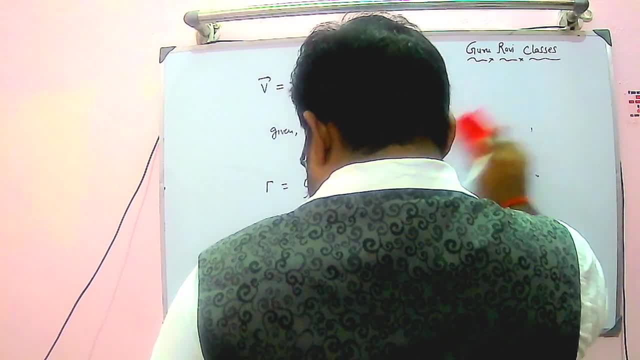 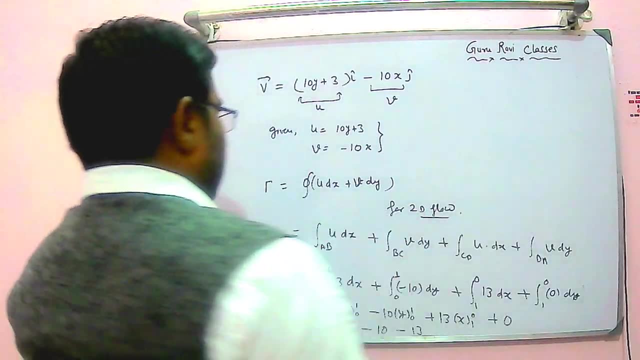 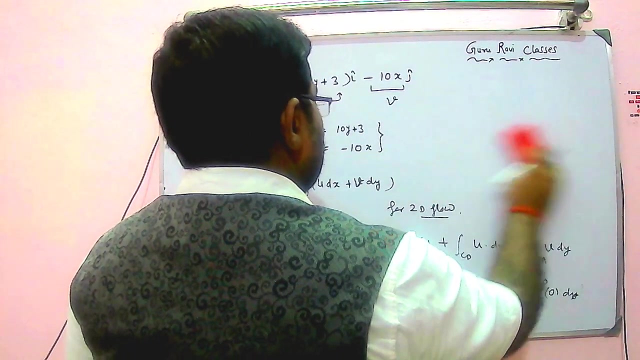 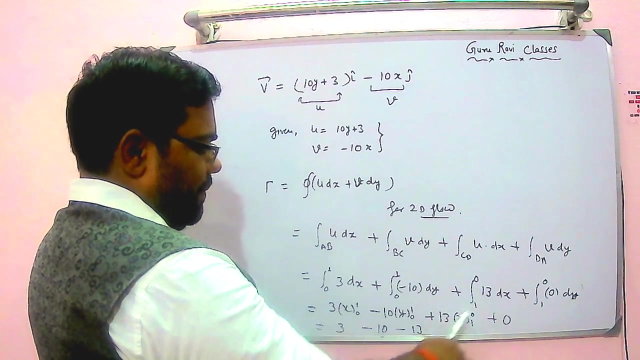 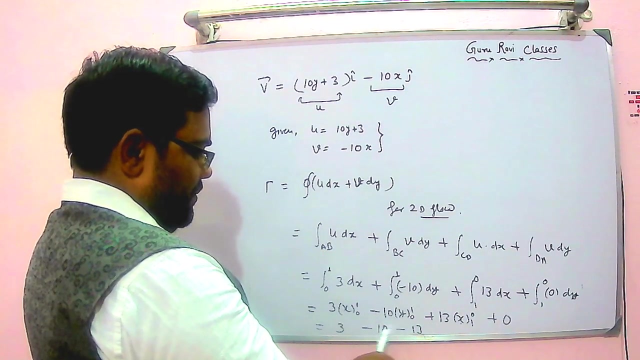 write here, So this is becoming minus 13 and this is becoming minus 10.. So if you add this, everything, so this is become 23,. right 23, and out of 23, 3 is going to minus 20.. So circulation is coming. 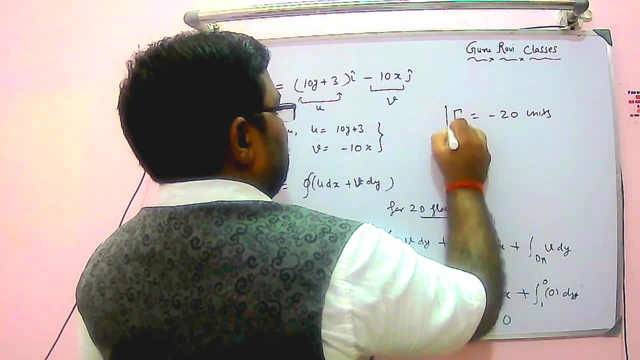 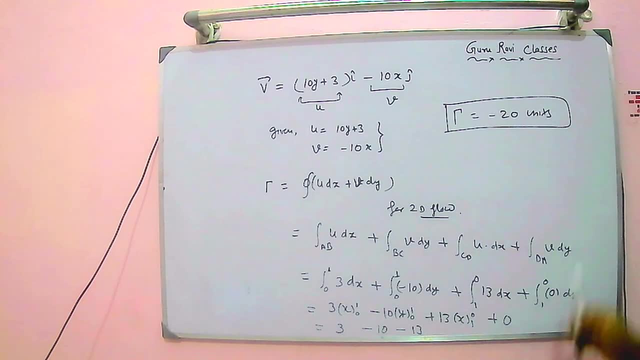 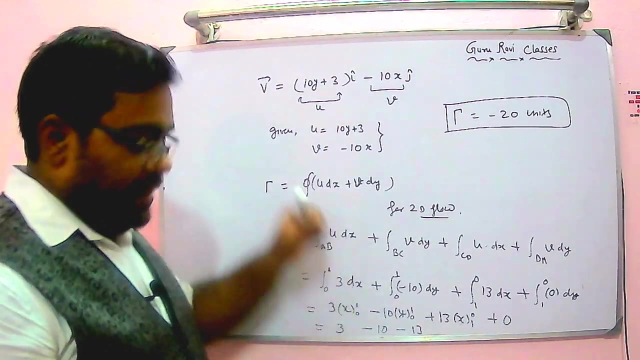 minus 20 units. This is the answer for this problem. So like that you can solve, Like this you can solve. So again, I am repeating This problem So it will be better understanding for you. So this is the velocity vector, which. 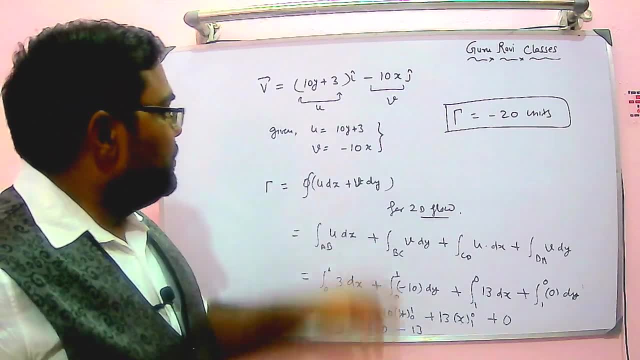 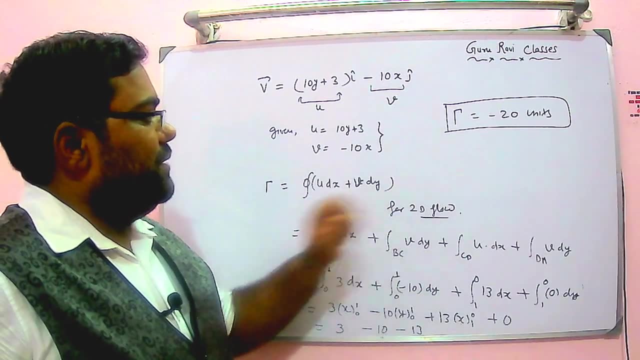 is given 10Y plus 3 minus 10X, right, So I can write: U is equal to this and V is equal to minus 10X. So then I have written: circulation is equal to U, DX, B, DY, right, So I can write. 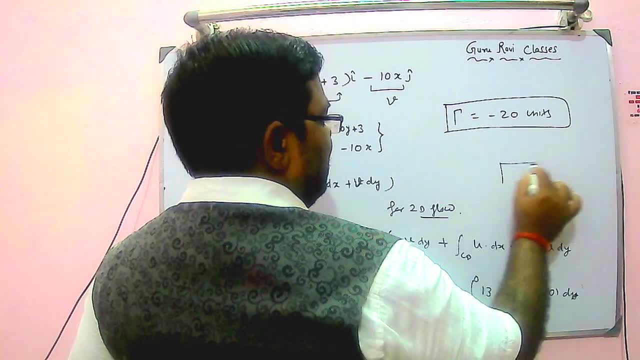 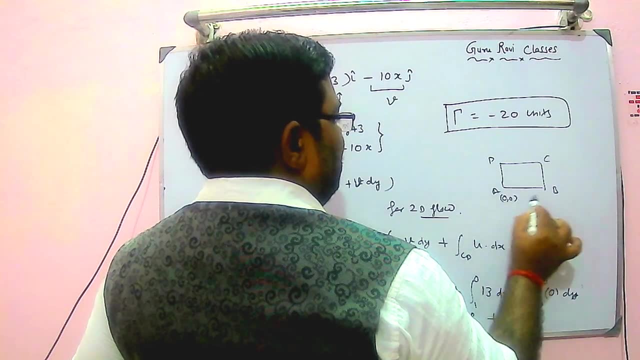 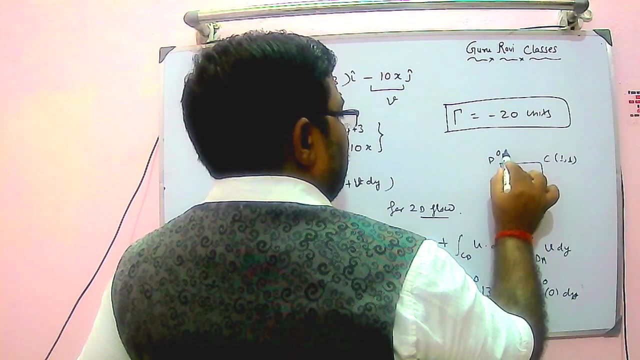 ABCD, How to get ABCD, which is something like this: It is coming right. So this is A, this is B, this is C, this is D. and here I know this is 0, 0.. This is 1, 0.. This is 1, 1.. This is becoming 0, 1,, correct, 0, 1.. So, and we are taking 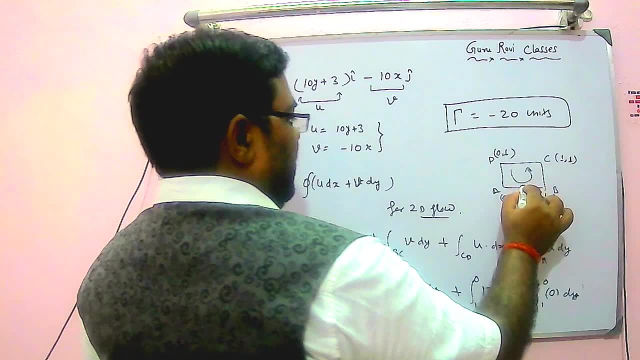 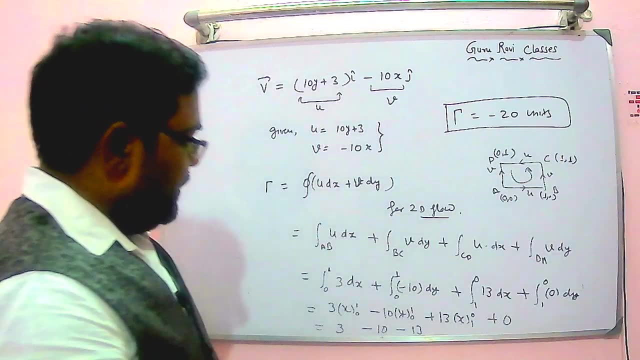 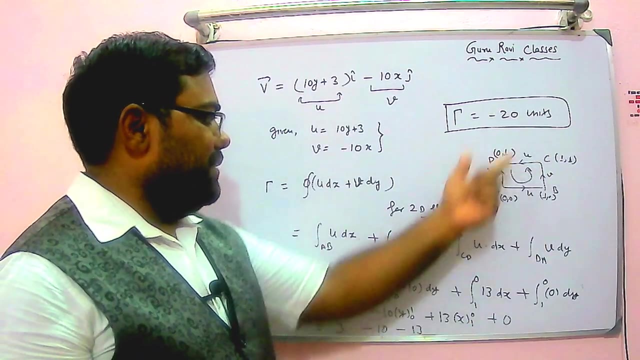 this kind of thing is positive right Circulation like this: Along this is U, along this is V, So V is here and U is here. So this is the thing, So we can write along AB, along AB. we have written U DX, because it is going like this: Along BC, V, DY, this is going like 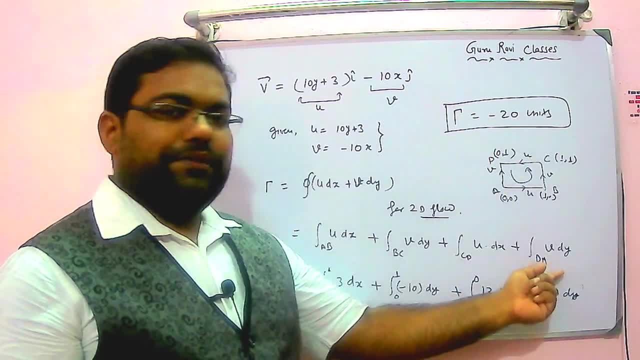 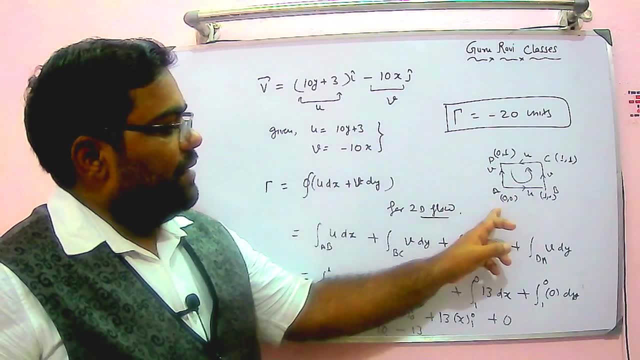 this Along, this U DX, along this V DY. Then we have to specify the limits. So look along: this U is 10Y plus 3, but here Y is how much: 0.. So I get only 3, right, 3, I have written. 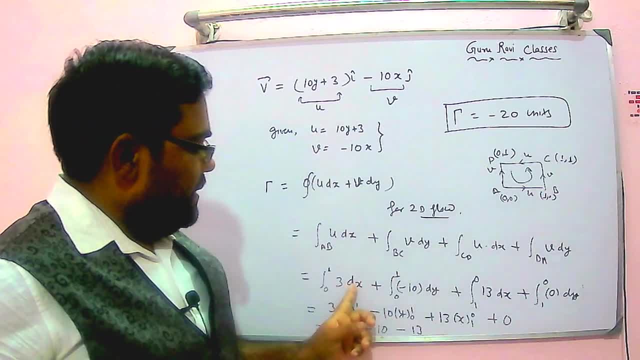 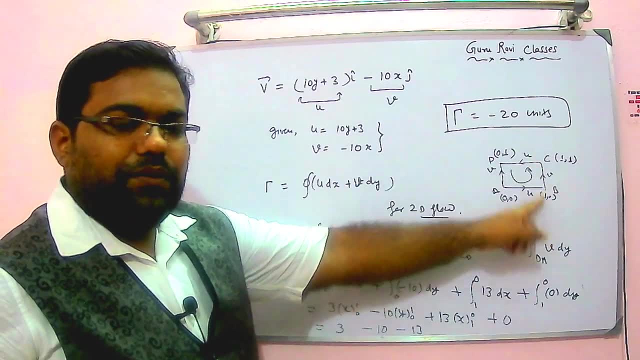 here, DX. what is the limit for X? 0 to 1,. I have written here Again. you look at the V: V is minus 10X, So V is going along this vertical line where X is equal to 1, basically. 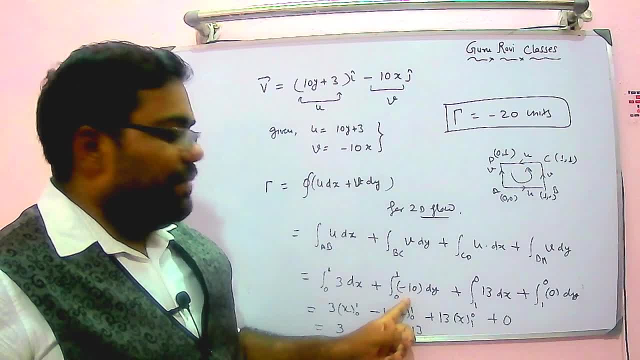 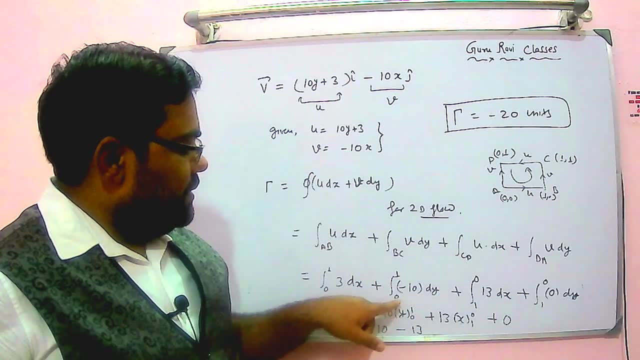 Look at here: X is equal to 1.. So X is equal to 1, I can get minus 10 DY. What is the limit Limit for Y? it is going from 0 to 1.. So I have written 0 to 1.. Then I am going along C to D direction, right? 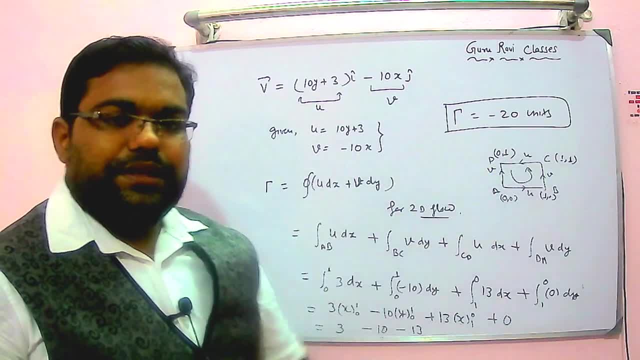 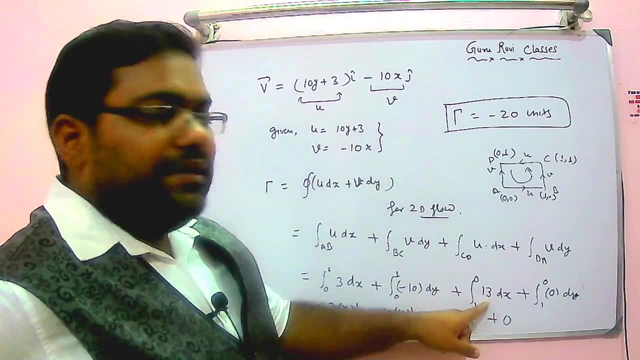 Where velocity component is small, u, which requires Y. What is the Y value here? That is 1.. If it is 1, here I get 13. DX Limit is going from X is going from 1 to 0 plus. 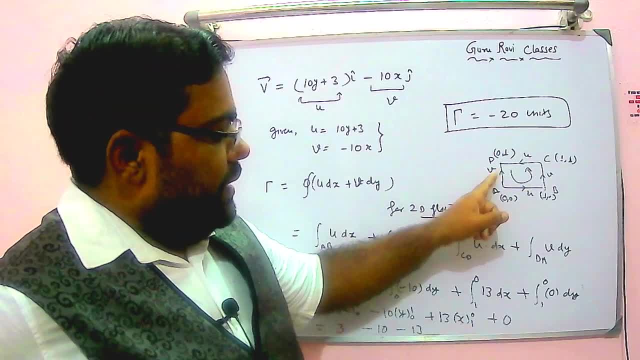 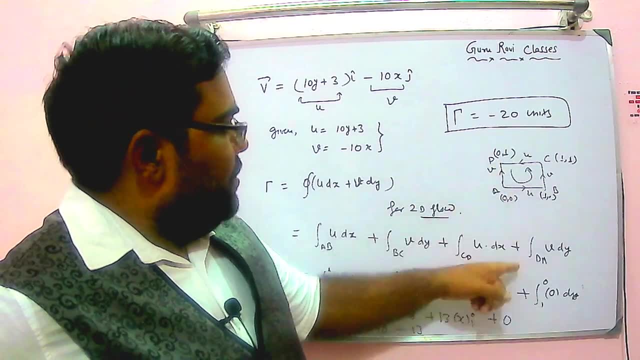 along this: This is a V right, Basically V, So V is minus 10X right. What is the X value over here? If you look at this point, X is equal to 0.. So if you put X is equal to 0, I get. 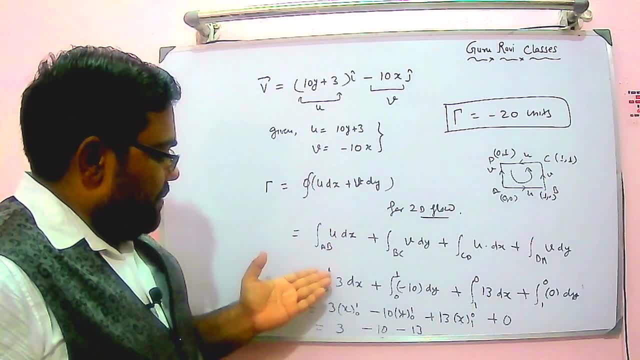 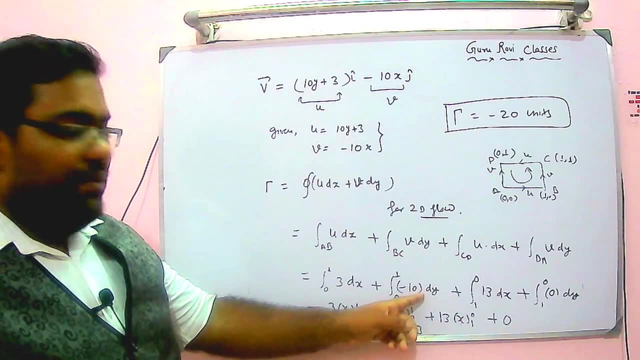 0 DY. Now you just integrate this. After integrating, I get here here 3,. here, I got 3, right. Here, minus 10 DY. So this is becoming minus 10.. Only I will get 1, right, This will. 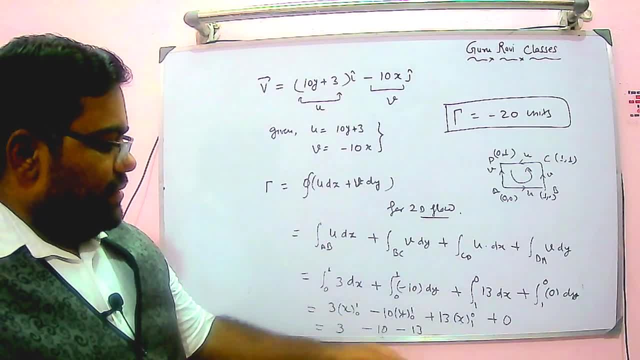 be minus 10.. And this last one, this is becoming minus 13.. So if you add this, this will be minus 10.. So if you add this, everything is 23.. How much 23? 3, you have taken out. 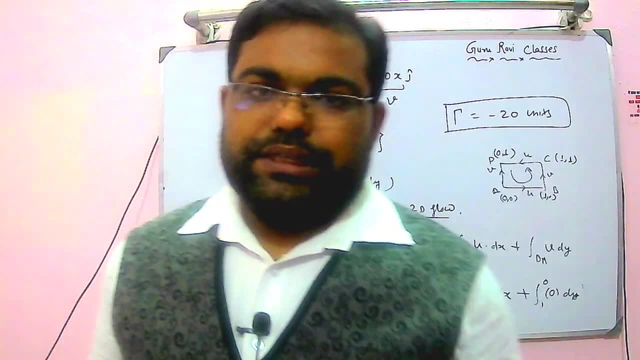 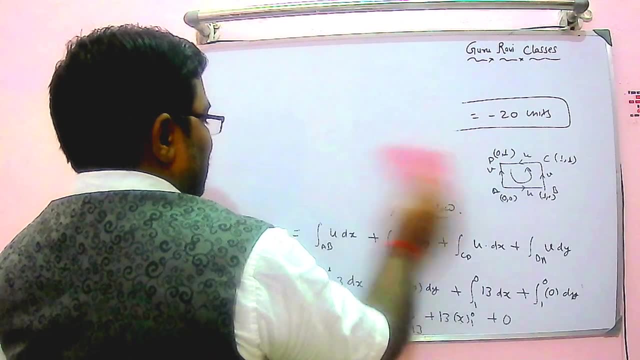 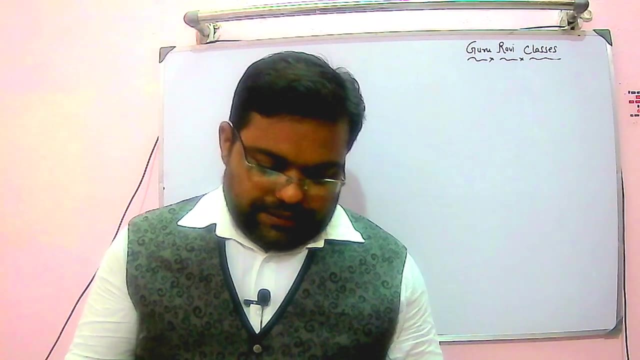 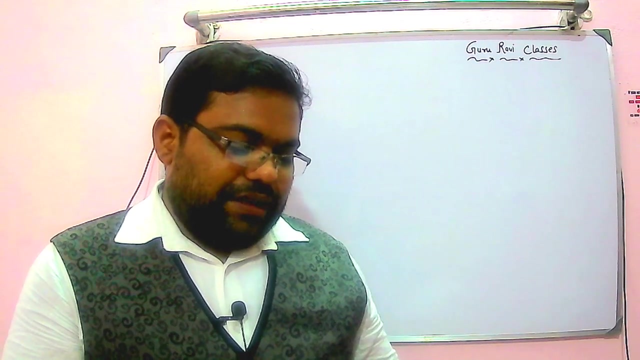 I got circulation as minus 20 units, So like that you can solve. This is the second numerical problem. Let us go for the next problem. So next problem says that determine whether the flow is rotational or irrotational for the velocity component. 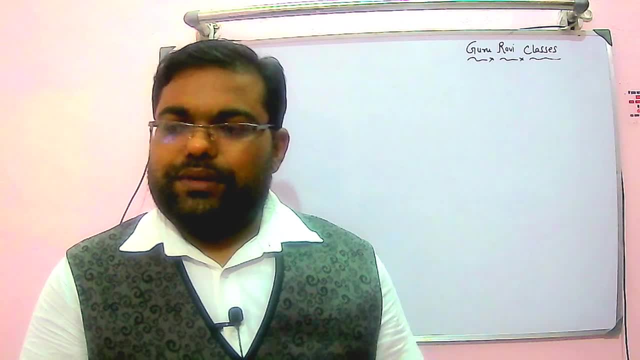 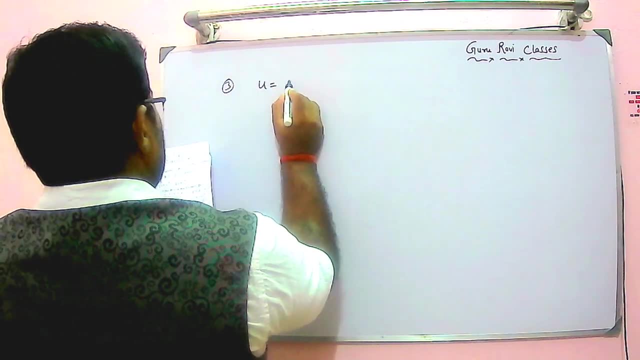 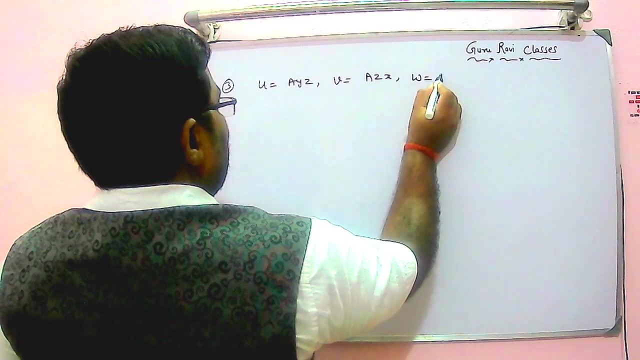 Some velocity components are given and you need to find out whether flow is rotational or irrotational. So what is the velocity components are given for, third, This is AYZ and V is equal to AZX and W is equal to AXY. These are the velocity components We need. 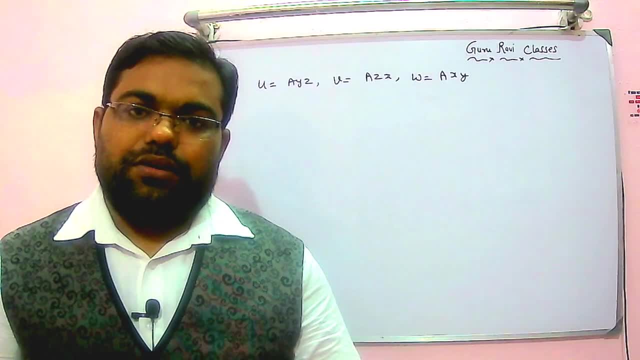 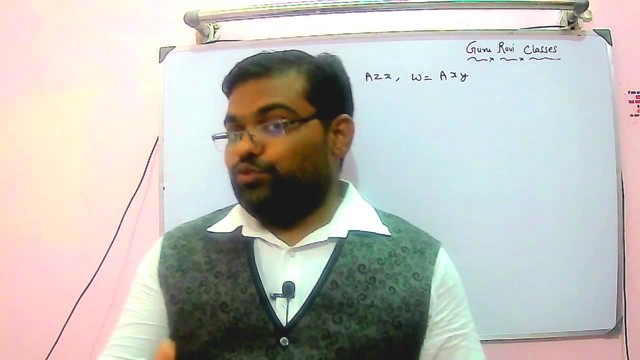 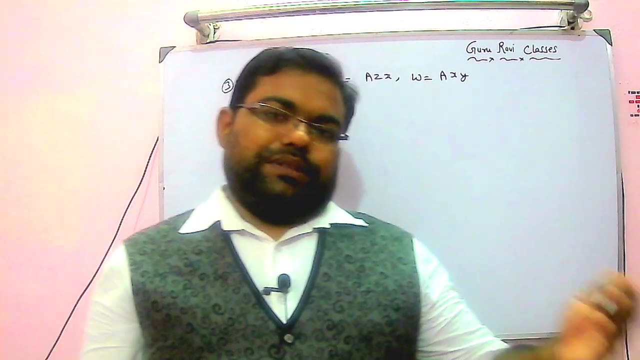 to find out whether the given flow is irrotational or rotational, right? So how to find it out? Either you can find out Y rotational Components individually or you can write: curl of velocity vector is equal to 0. Any one is possible, right? So I will go with the first case. right, That is rotational. 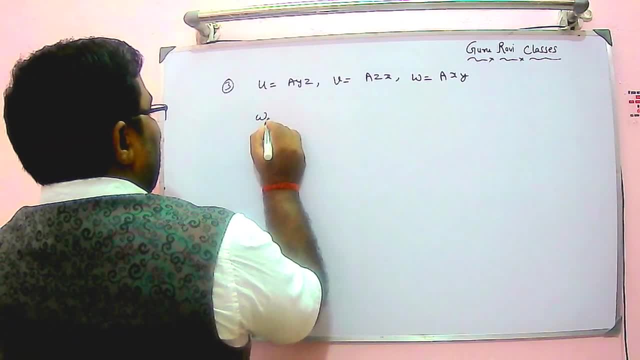 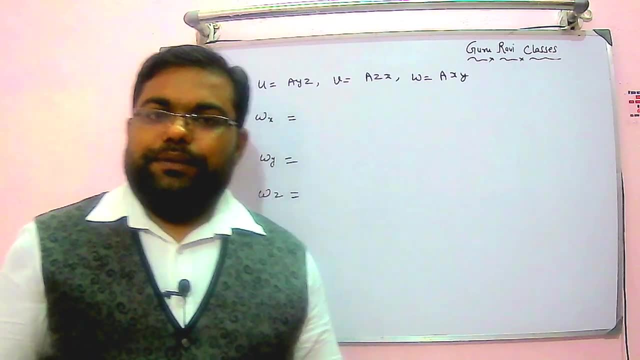 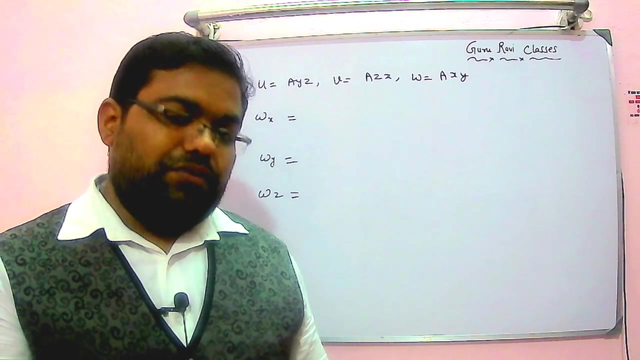 components, So WX, WY, WZ. I will find out this: If any one of, if all these are 0, I will say irrotational flow, If I am getting value of any one of the component, then I: 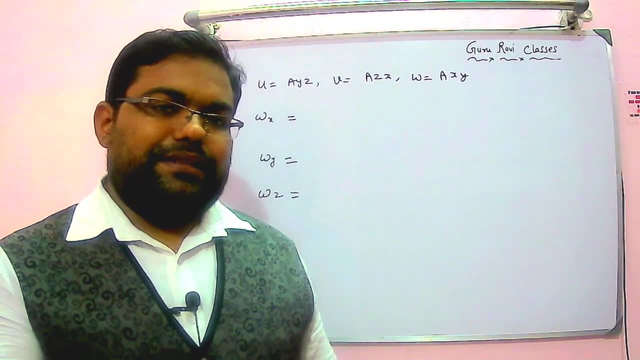 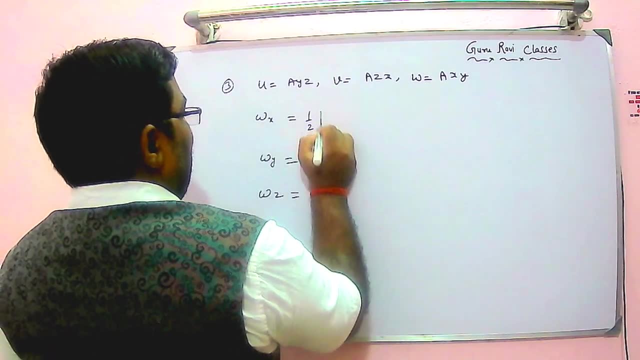 will have a definite value of rotation. right That I can say that flow is rotational, Clear or not. So let us rewrite the formula. So WX, we can write half. This is 1 by 2.. Here Y, here Z. 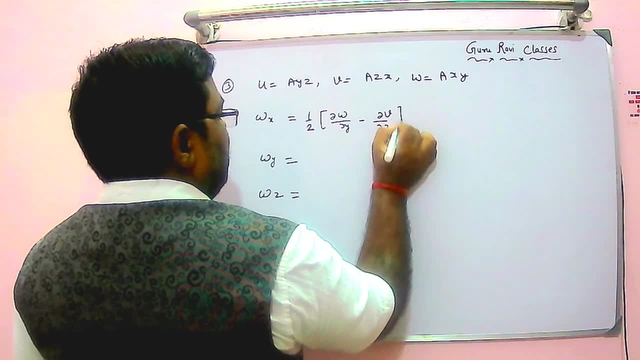 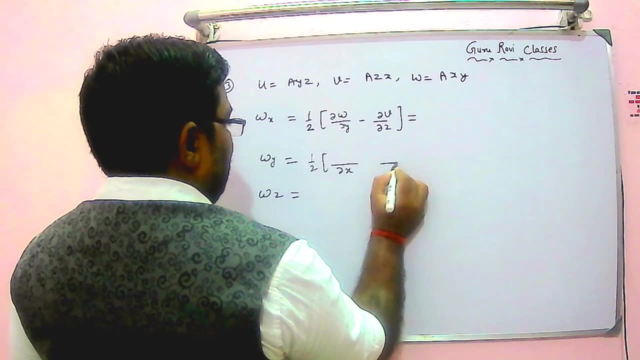 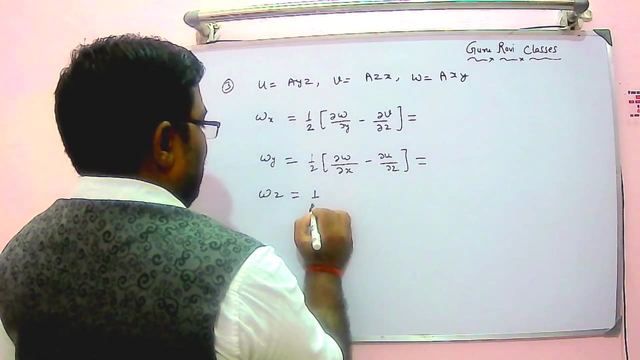 here W and minus sign and here V. So this we can calculate And this become half, and here X and here Z. Here we can mean W And here we can mean U. This is another formula. And half, here we can mean X and here we can. 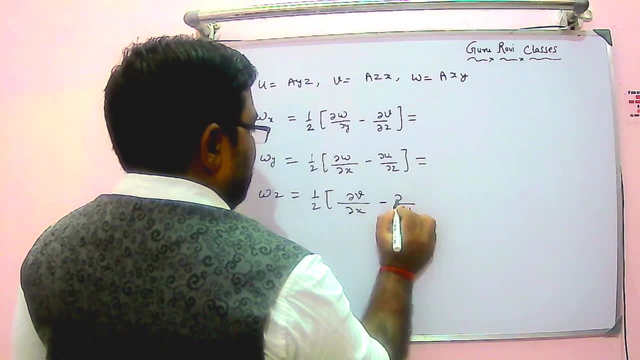 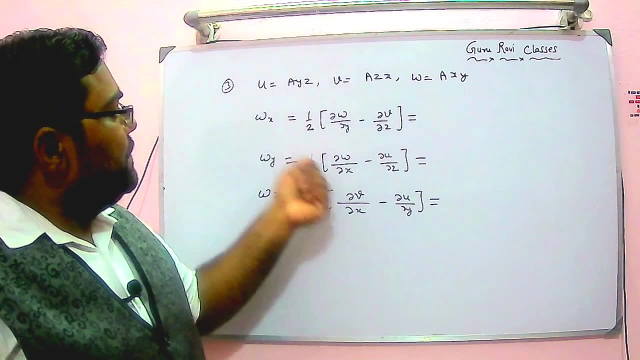 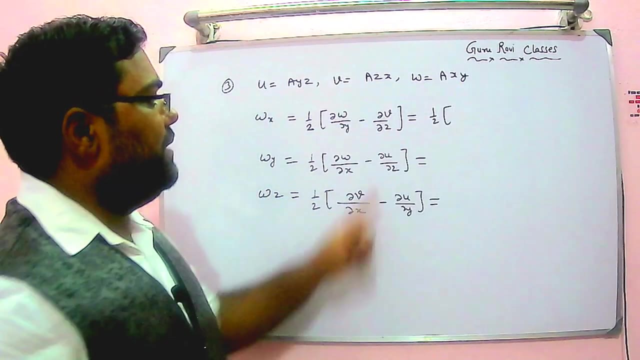 mean Y in between minus V and dou U. So these three velocity components we need to find it out right. Just look at this. So I will write here just simply: half W component is here AXY, and we have to differentiate this with respect to Y. I will get A into X. 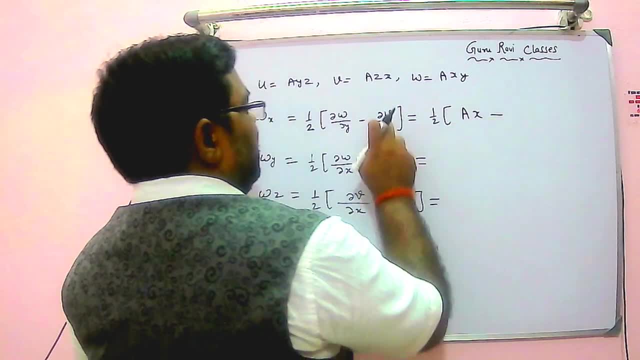 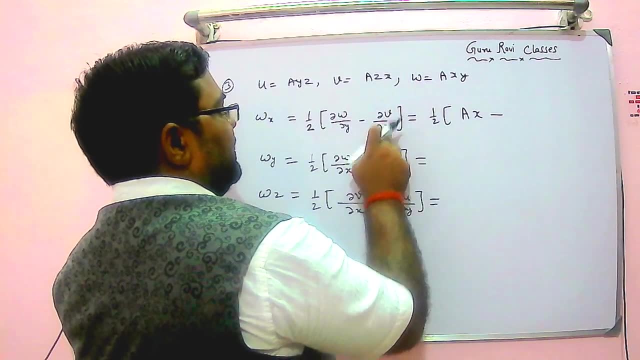 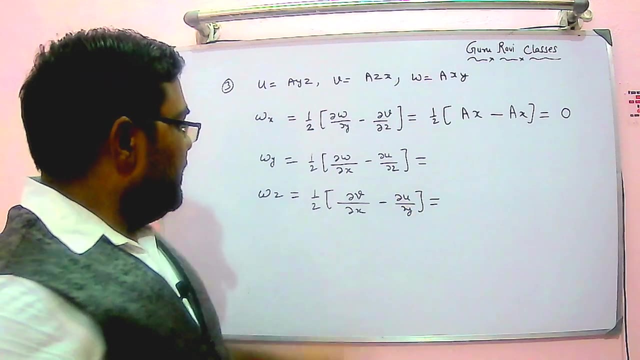 Right, I will write AX minus. Now look at velocity component V, which is AZX, And we have to differentiate this with respect to Z. I get AX. So look at this. This I am getting directly 0. Clear. Next one. Now, W component need to be differentiated with respect to. 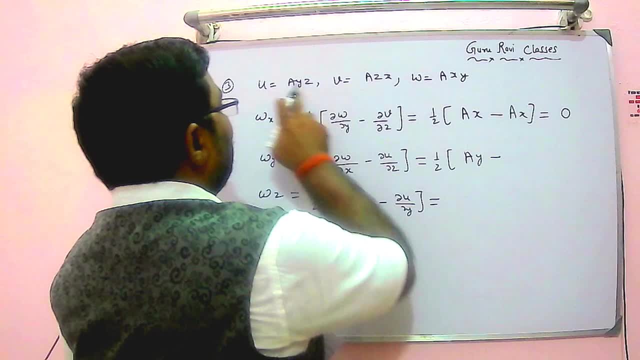 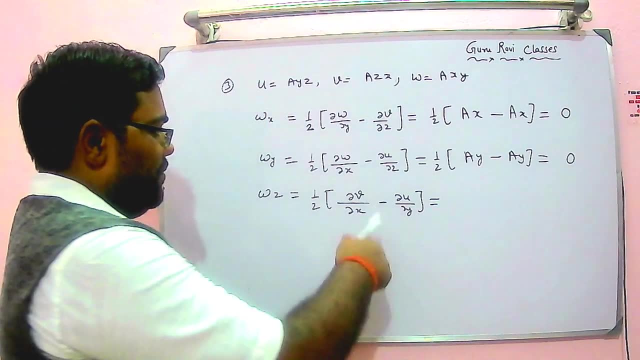 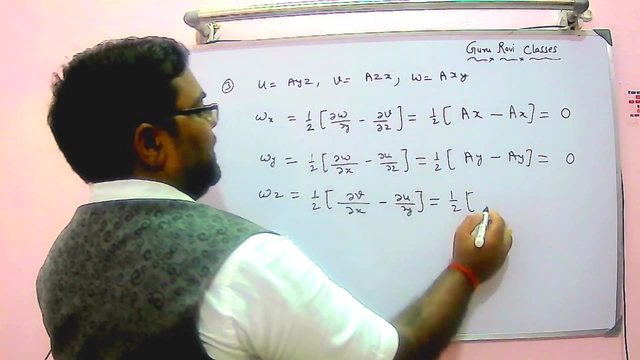 X, I get AY, minus U component with respect to Z: I get AY. This is also becoming 0.. Let's try for the third one. So half velocity component V with respect to X. V is here. With respect to X, I get AZ, minus U component with respect to. 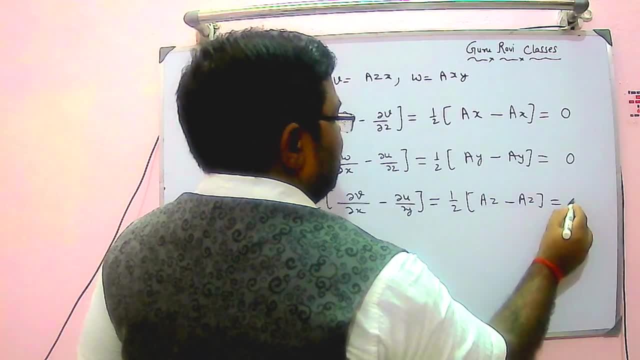 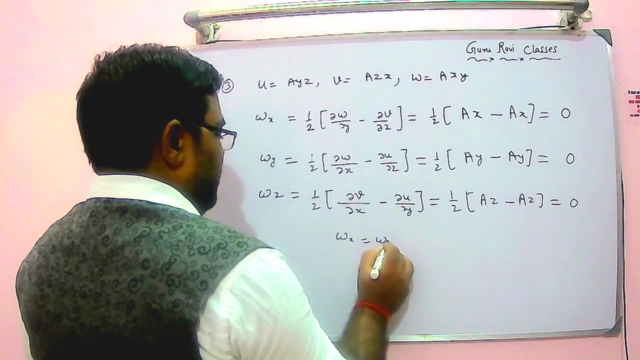 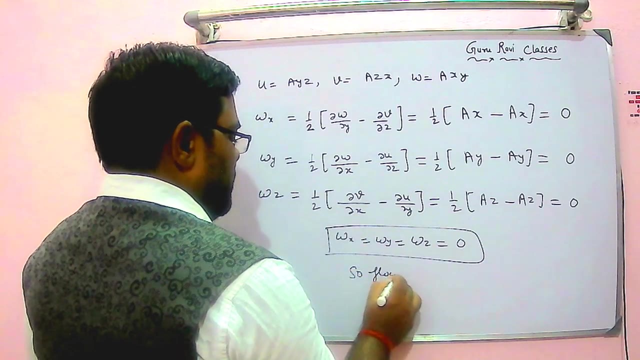 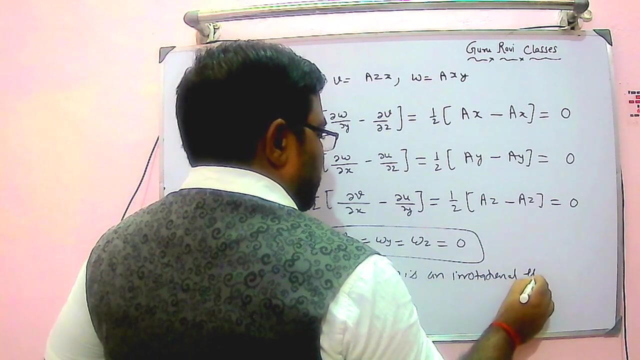 Y. I get again AZ. This is also equal to 0.. What we came to know from here. So WX is equal to WY, is equal to WZ, is equal to 0.. So flow is an irrotational, irrotational flow. That's all Over. Like that, you can. 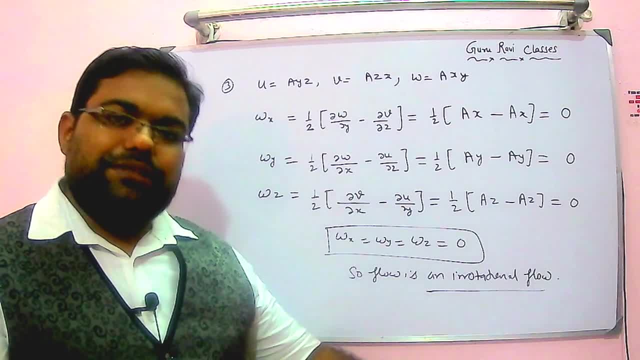 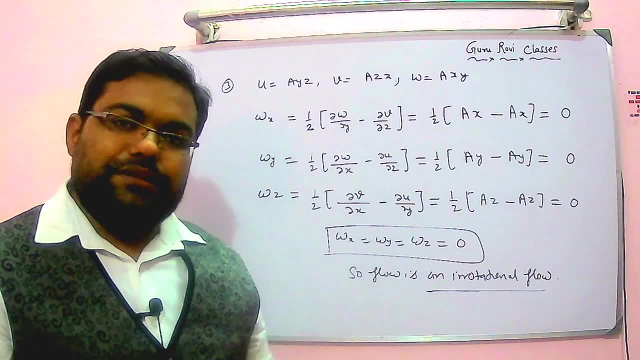 find it out. That's the one way: or curl of velocity vector, or curl of velocity vector, if you apply, If that is becoming equal to 0, you can get. you can say this is irrotational flow. If it is not equal to 0, then rotational flow. 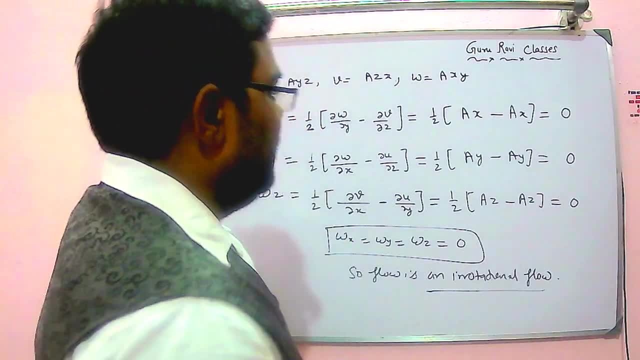 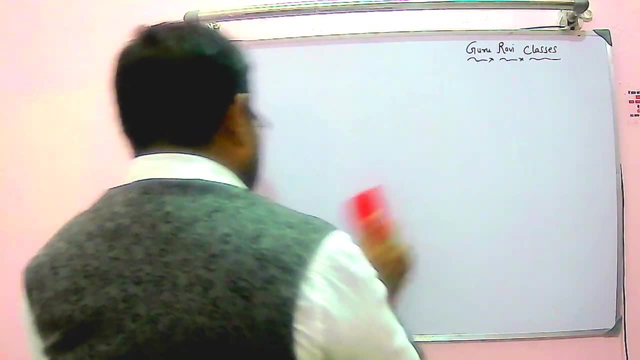 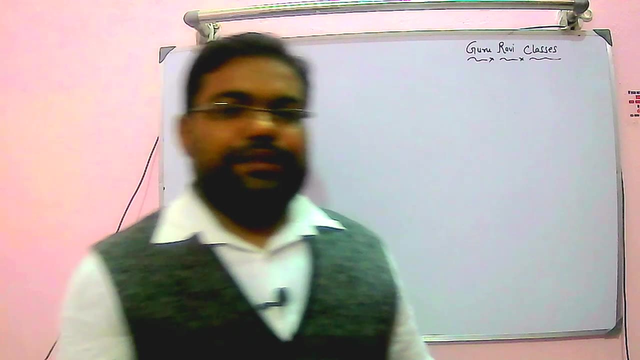 This is the third problem, Basic, fundamental problems on the fluid flow. So I am- I am going to next problem right now, from the wing sections. Alright, That is, I have done force calculations, Alright, From that. So what is the time? now? It's 28.. Still, we are having. 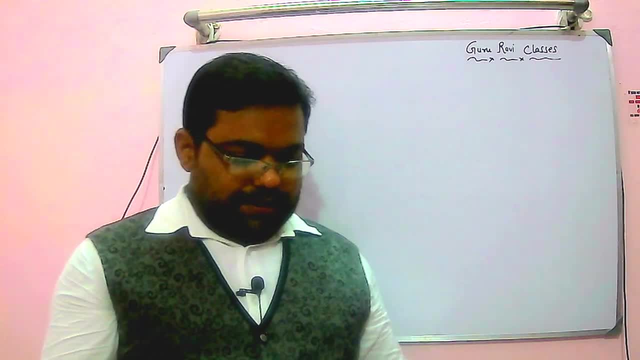 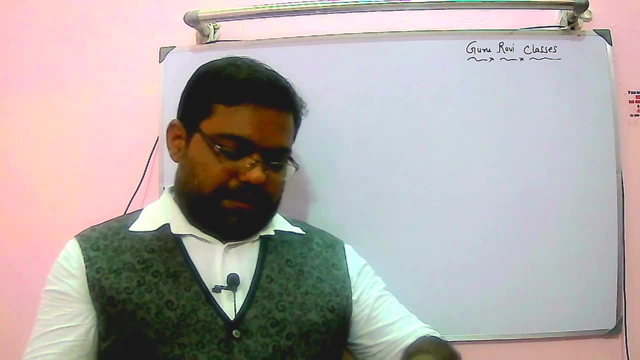 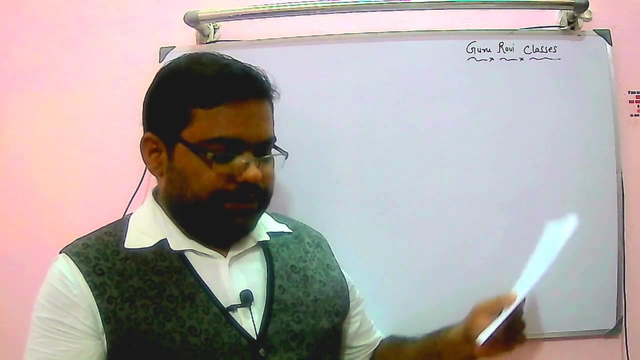 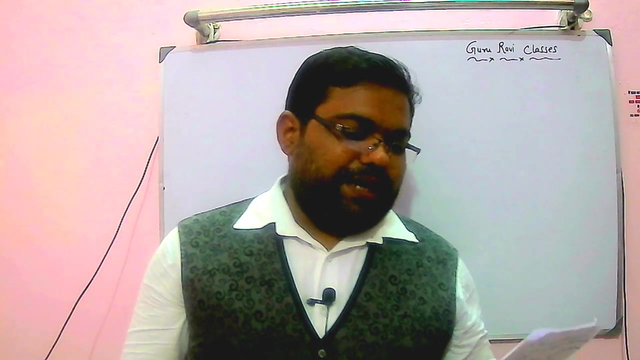 time. So let's take the problem. This is slightly lengthy problem and we have derived the expression for this as well, So I am dictating Again. note it down: Consider two comparable aircraft in level flight. They are flying like this horizontal flight. Consider two comparable aircraft in level flight and are: 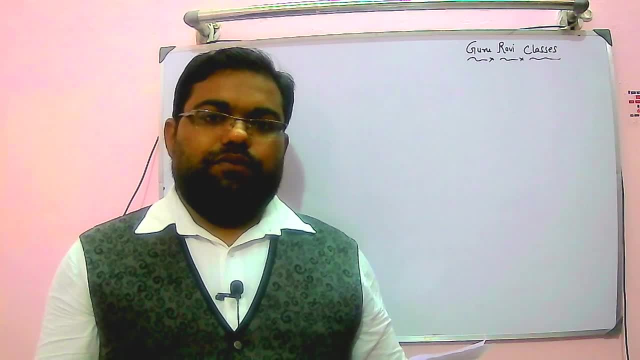 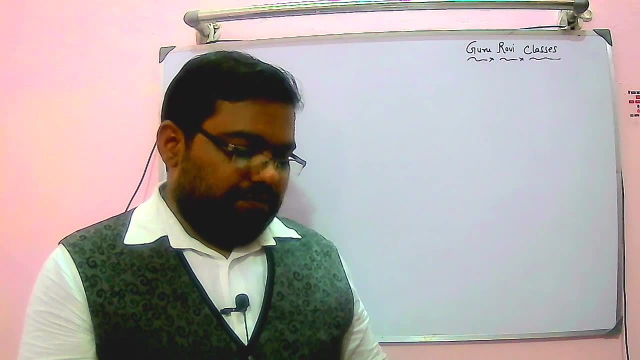 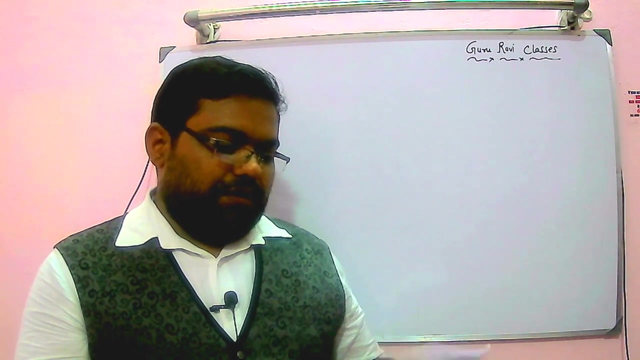 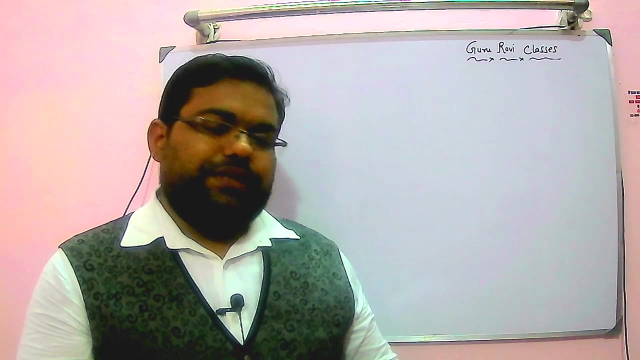 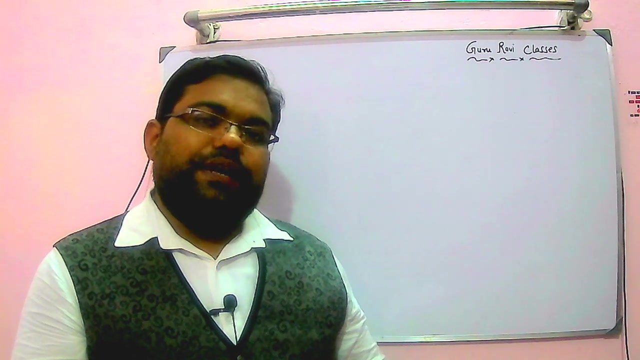 flying with true air speed of 160 km per hour under standard air conditions. Full stop The aircraft are identical With weight, wing areas of 10 kN and 45 m2 respectively. Full stop Wing spans of the aircraft are 14 m and 20 m respectively, So wing span is different. For one it is 14. 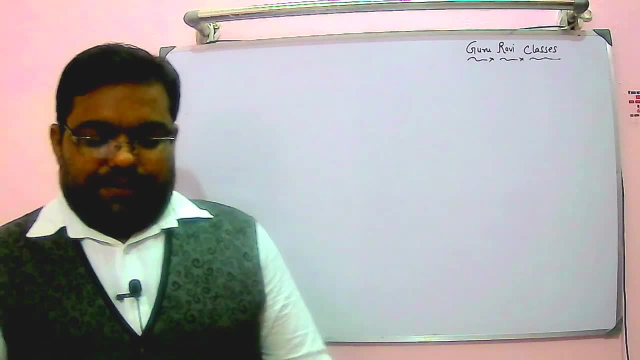 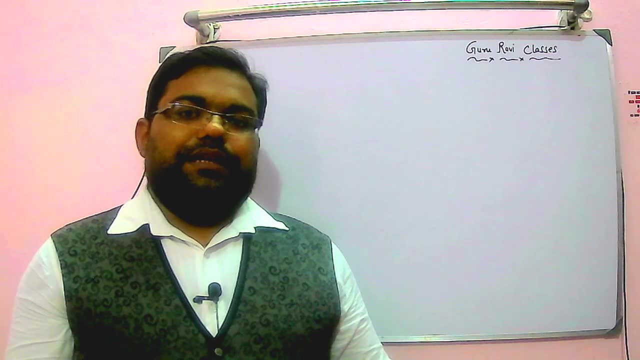 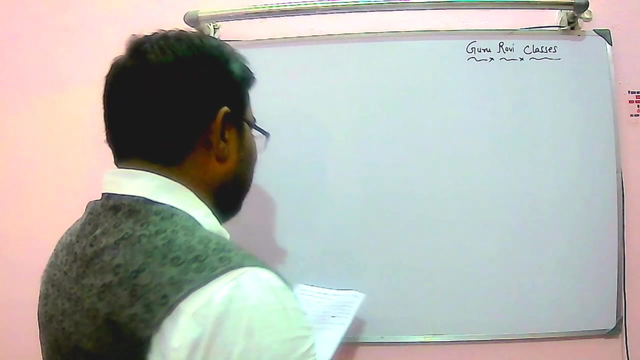 m, For another it is 20 m respectively. Determine the difference in geometrical angles of attack, The difference between the geometrical angles of attack for the two aircraft. So let's take what all things are given. Two aircrafts are given, both are comparable, So for both, 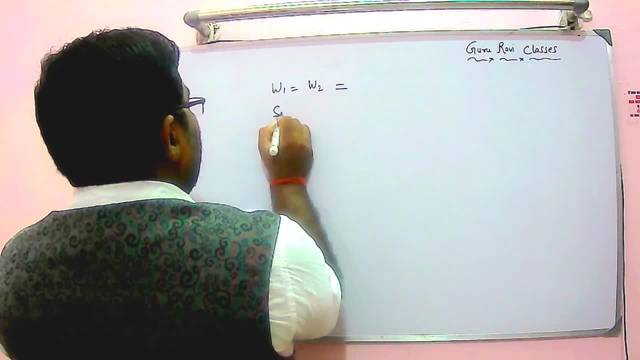 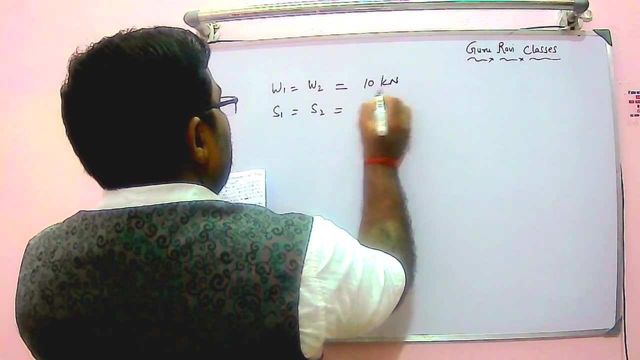 W1 is equal to W2 is given Wing area S1 and S2, both are given. So how much it is this? This is 10 kN, Alright, And this is 45 m2.. So how much is it? 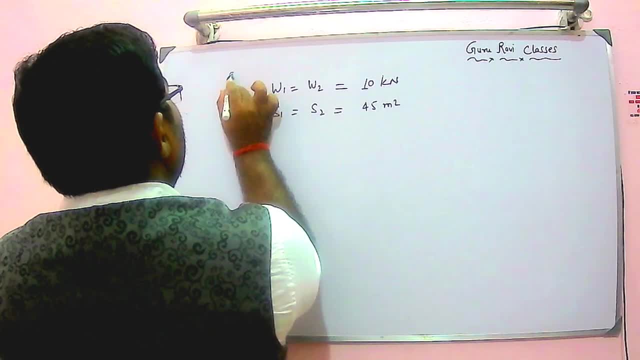 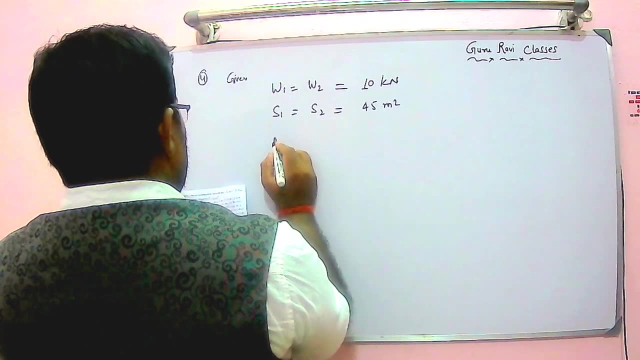 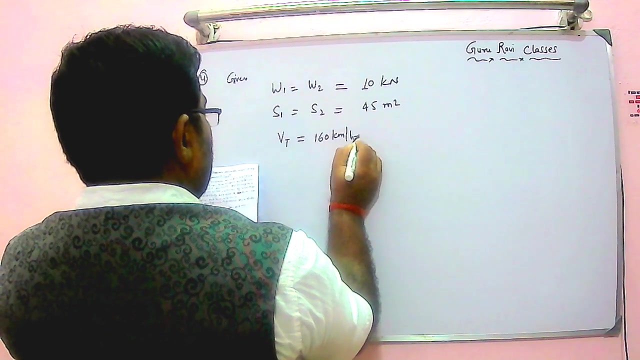 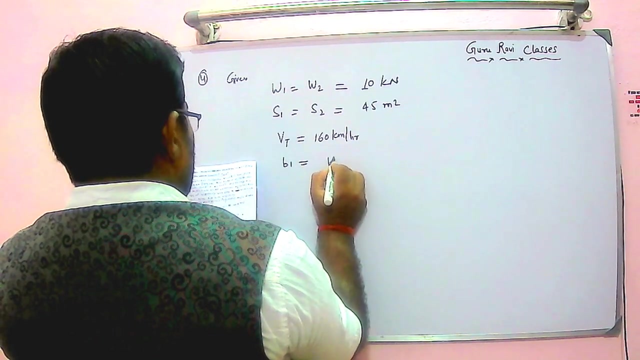 This is 15 m n2.. meter square: this is basically given data. given is the problem. number four and another. both are flying at true airspeed, v true is given 160 kilometer per hour. right and wingspan are different. b1 is given as a 14 meter and b2 these are the wingspan. i am writing 20 meter respectively. 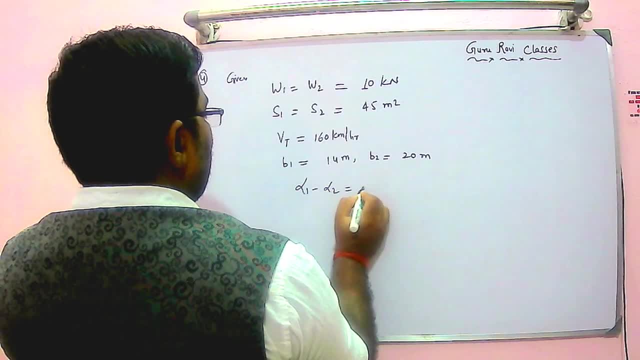 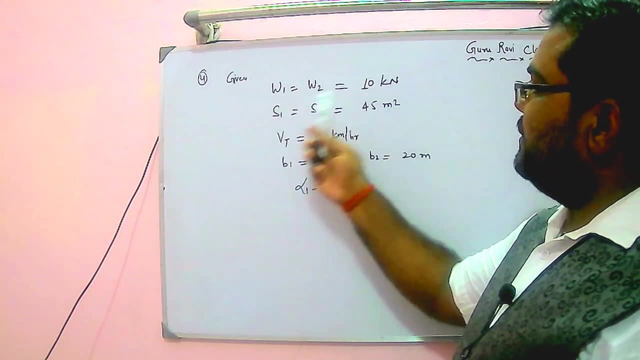 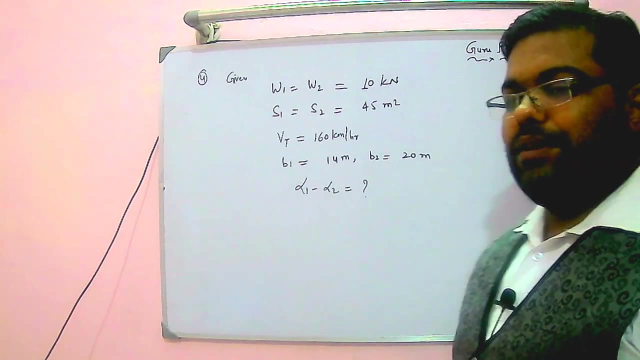 and we need to find out alpha 1 minus alpha 2. this we need to calculate. so look at the data. so data is here. weights are given, s1, s2, b- true is given, b1 and b2 are given. these are wingspans and alpha 1 minus alpha 2 need to be calculated. so now we will go very basic, fundamental. 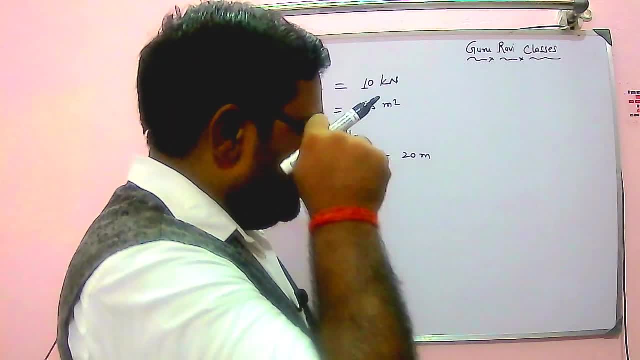 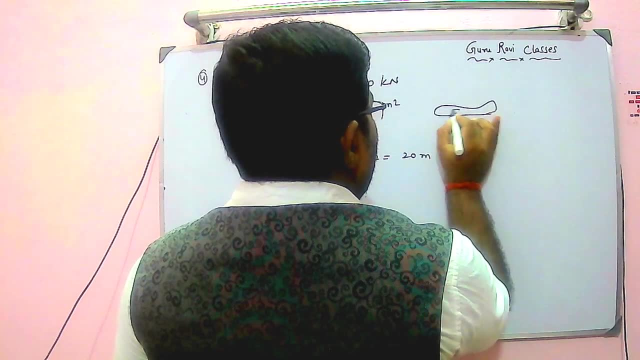 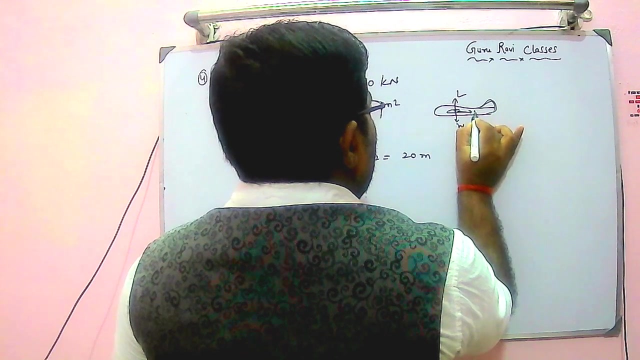 you know approach, that is, it is said like they are flying horizontally. so aircraft is flying like very, very, you know, ah, nearly horizontal flight. so this is the case is flying like this: in this case, lift will be exactly equal to weight and thrust will be equal to drag. so lift is equal to weight and thrust is. 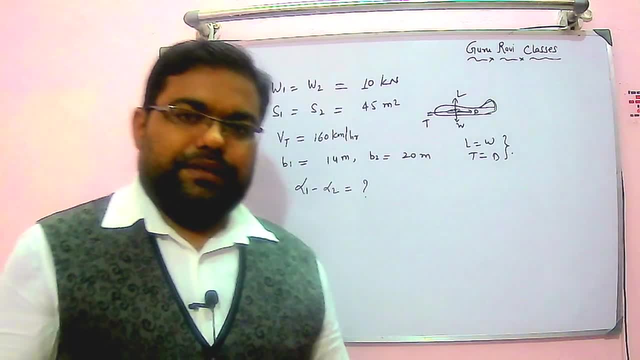 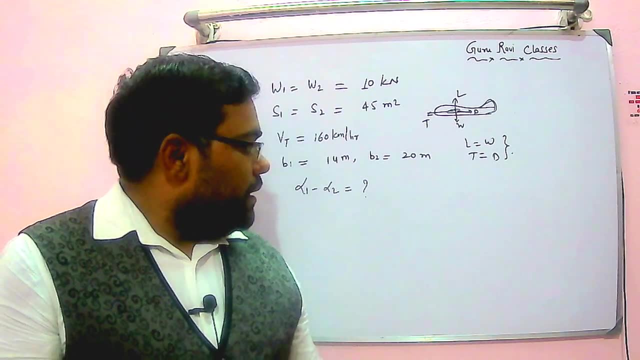 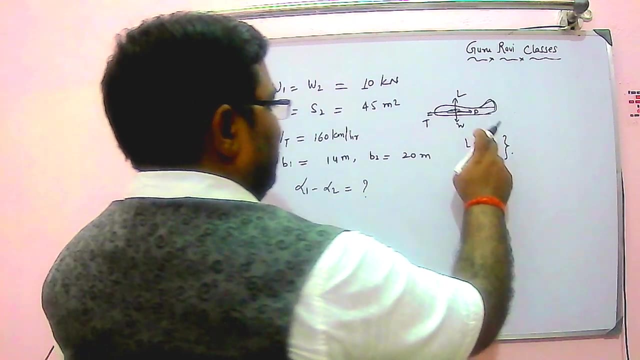 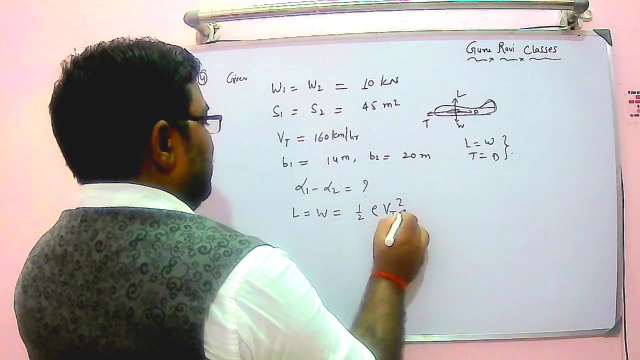 equal to drag. this is the condition for horizontal flight and it is flying in standard air conditions. for that properties we already know from international standard atmospheric table, or for air, we know the properties. so let's start this concept right, this approach: lift is equal to weight, is equal to half row v, true square s into cl. 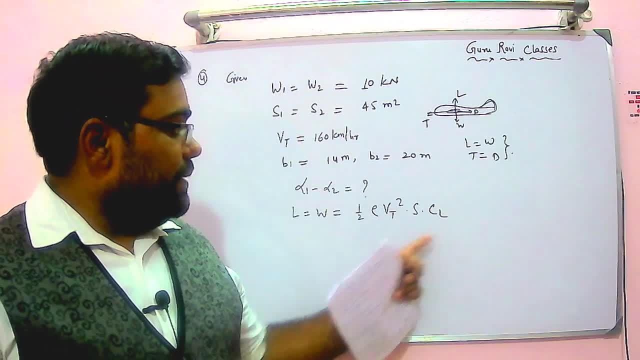 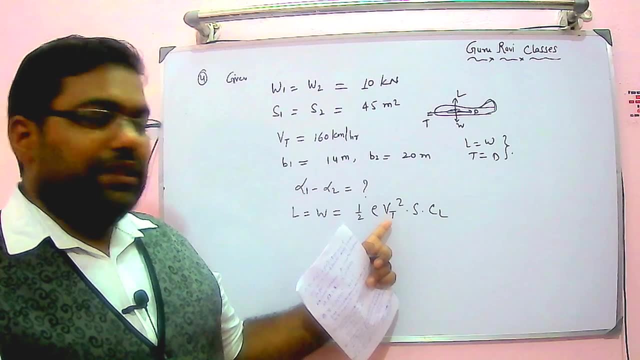 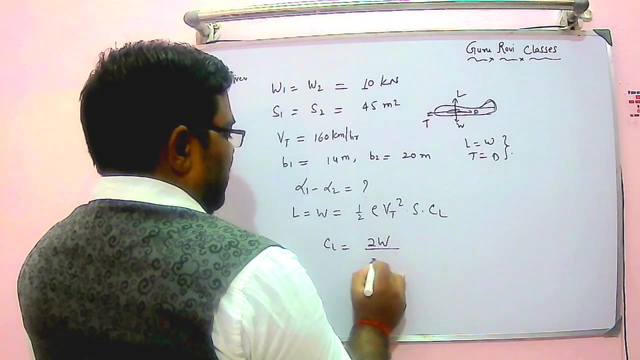 we need to find out the coefficient of lift first, and coefficient of lift will be same for both, because wing areas, weight, both are same, right and surface area means everything is same and true. air speed is also same. so from here we can write: cl is equal to two times of weight divided by density. 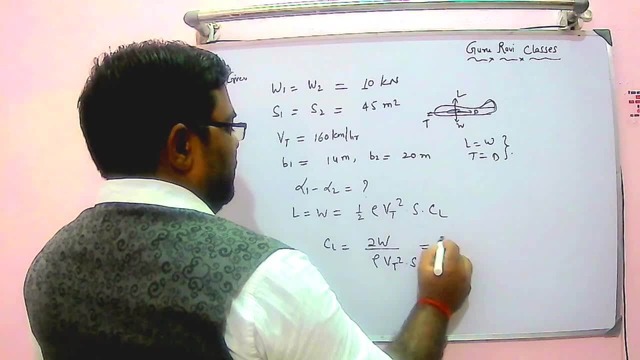 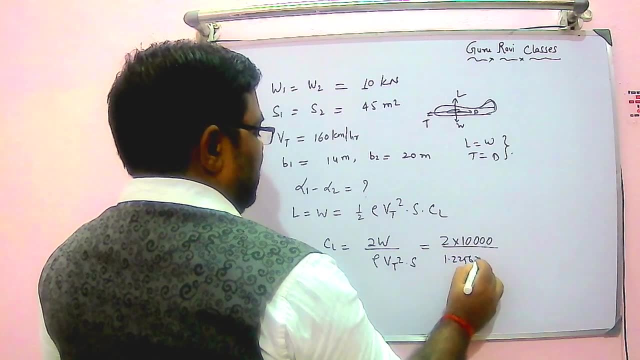 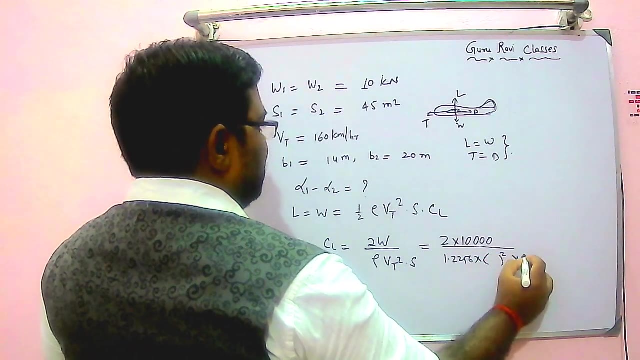 v true square into s. so you can write two times of ten thousand right. kilo newton is becoming ten thousand divided by density, one point two, two, five, six into v true, you change into meter per second. put the value here right, whole square into wing surface area is forty five. so if you put it you: 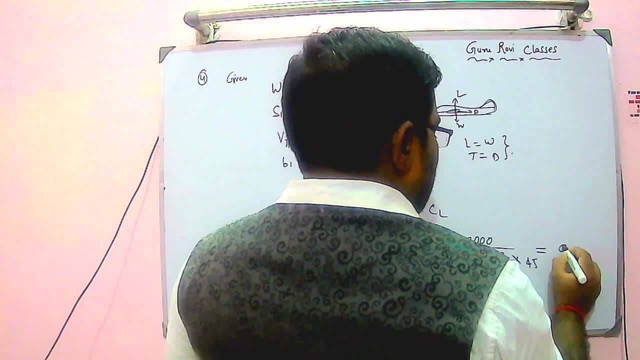 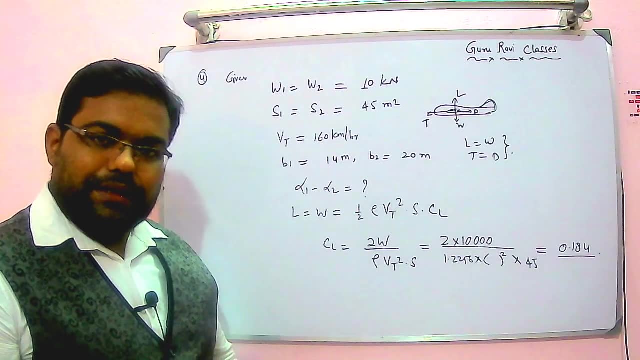 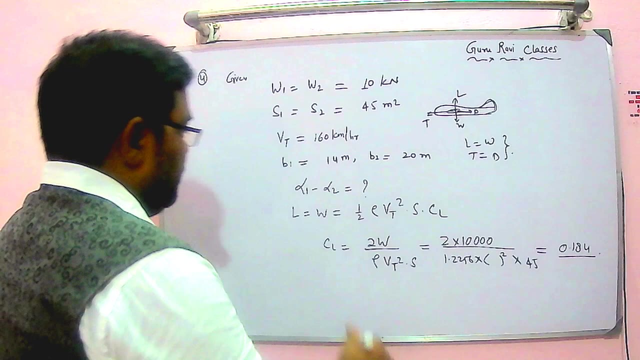 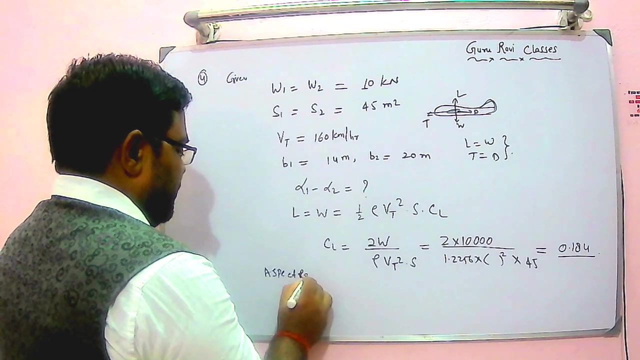 will get the cl value which is coming around: zero point one, eight four. so this is the cl value for both cl1 and cl2. both are now the same. clear up to here. there should not be any doubt. uh, now, as wing span is different, right, so, uh, we can go for aspect ratios, aspect ratio- right, so we can get aspect. 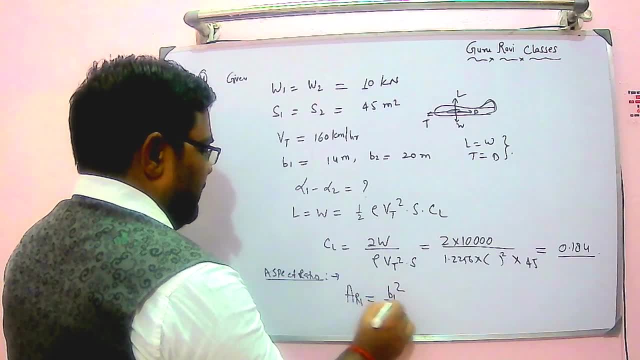 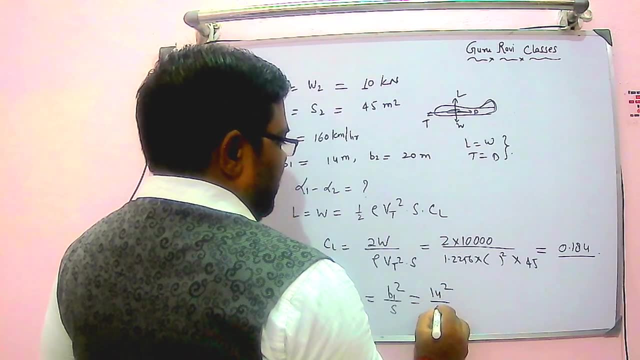 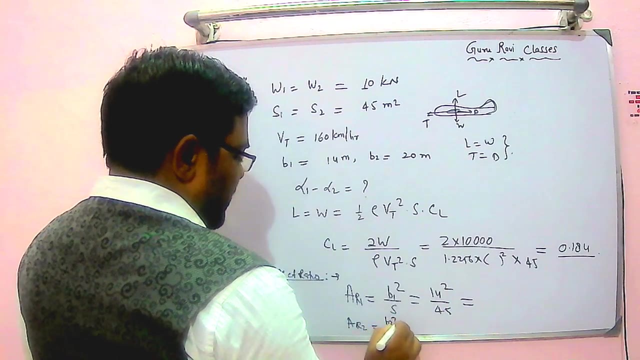 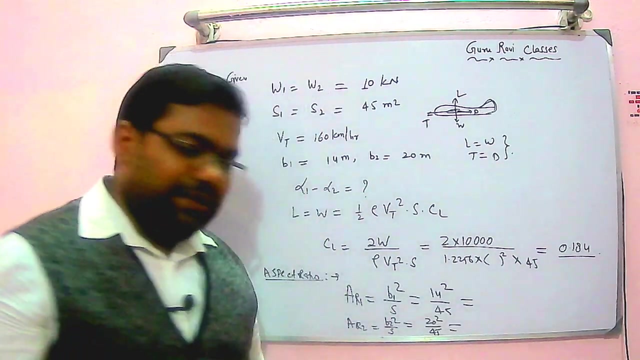 ratio, one that is nothing but b1 square divided by wing span right b square by s. so this is 14 square divided by 45. is the one answer. another aspect: ratio 2. this is b2 square divided by s, so b2 is 20 squared divided by 45. just use the calculator and put the value i will give. 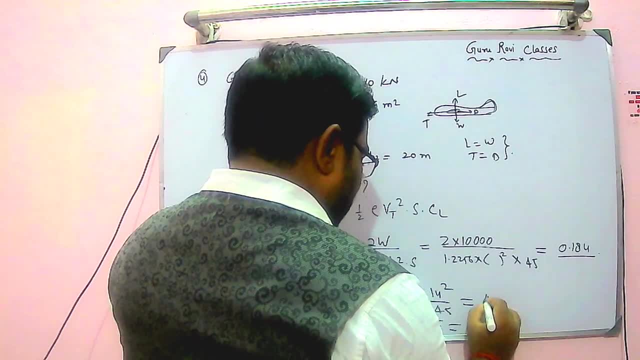 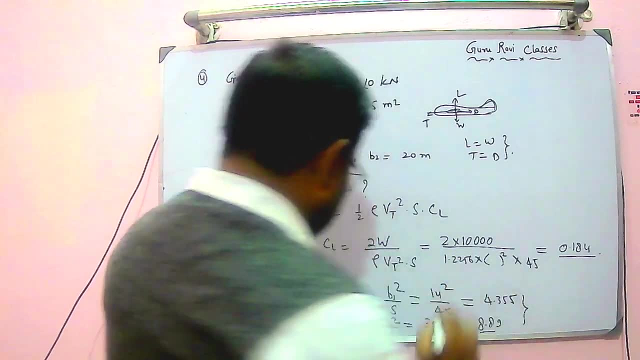 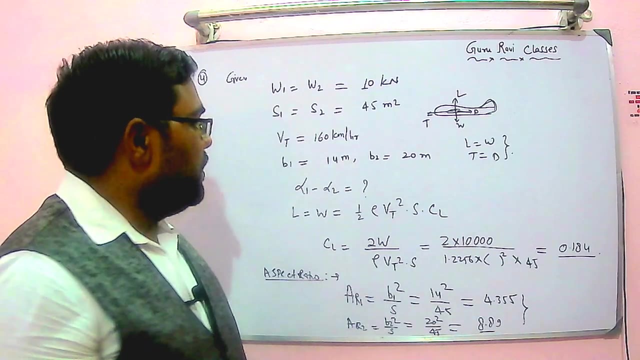 you direct value. so aspect ratio 1 is coming around 4.355 and aspect ratio 2 is coming 8.89. so i got two aspect ratios right for two different areas: curves. this is given now. now how to start these two these things you calculated. now we'll go. 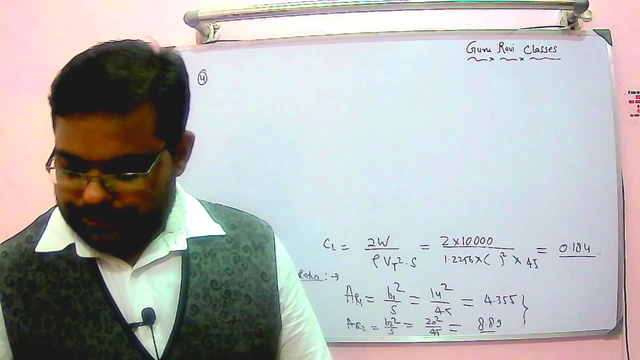 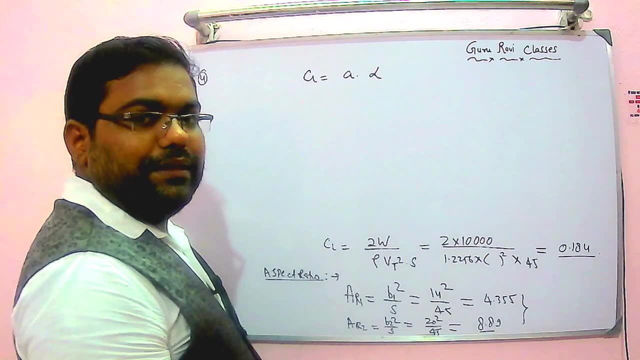 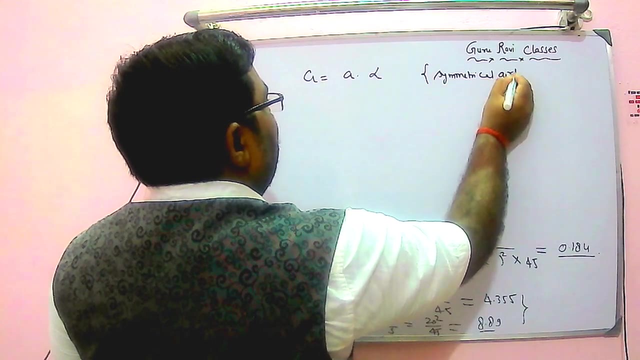 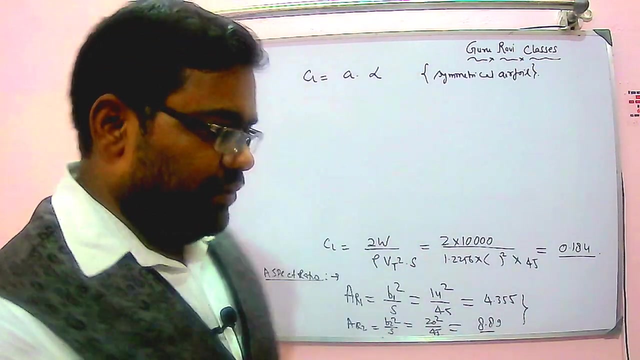 to the next step. all right, we know cl is equal to a. into alpha right. this is basically. we are assuming symmetrical f oil, symmetrical f oil, all right. and we are dealing with the wing. so for wing, we know the uh equation. that is a, so cl. 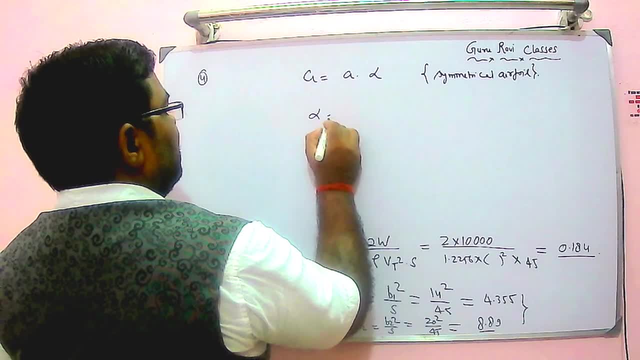 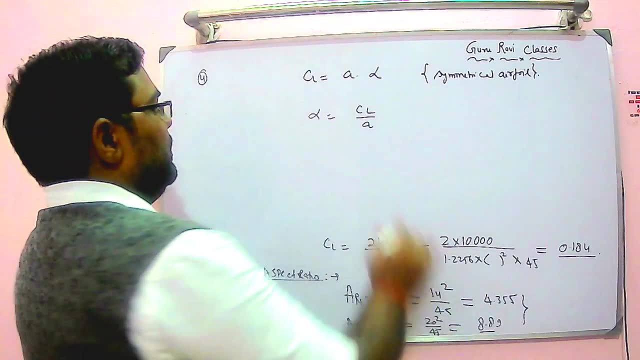 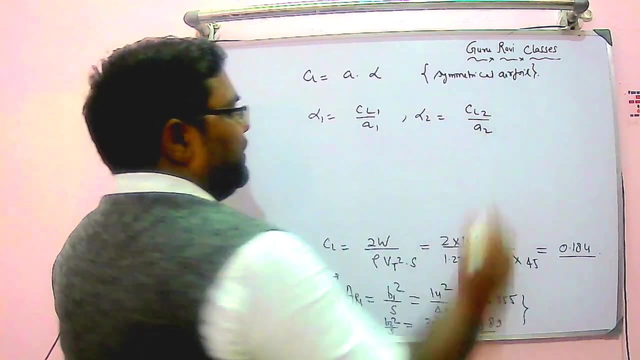 so we can. we can say from here: alpha is equal to cl divided by a. can we say cl divided by a? one thing? so if i say alpha 1, then cl1 by a1 and alpha 2 is equal to cl2 divided by a2. can i say yes? 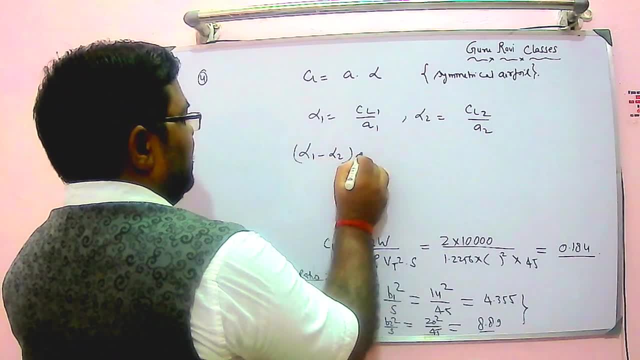 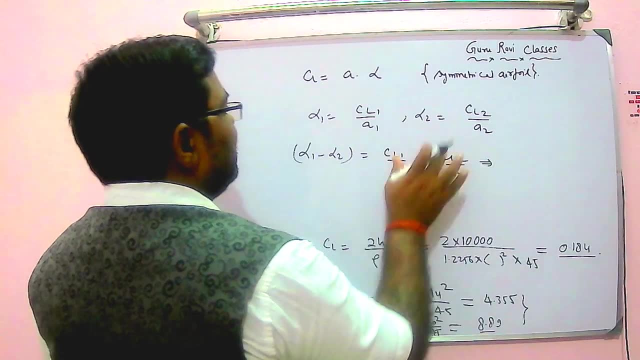 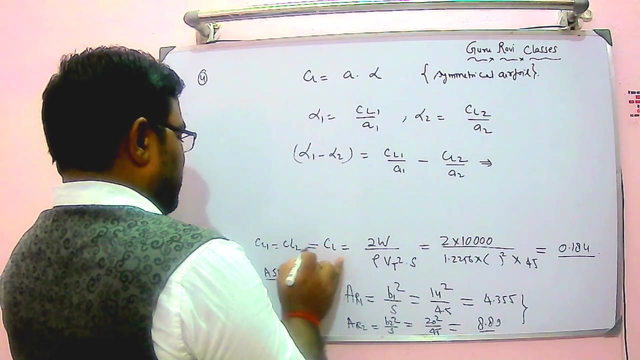 so alpha 1 minus alpha 2 can be written as cl1 divided by a1 and cl2 divided by a2, but we know cl is same right for both. this is here cl1 is equal to cl2 is equal to cl, which is given. 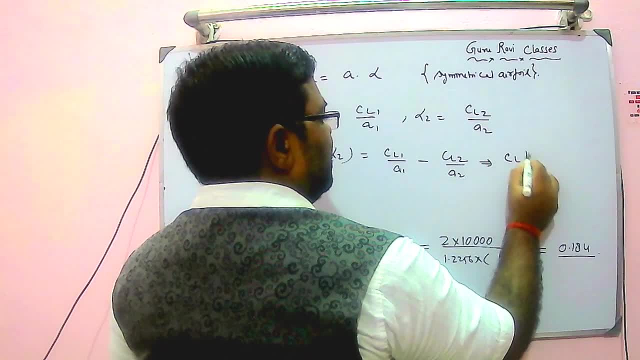 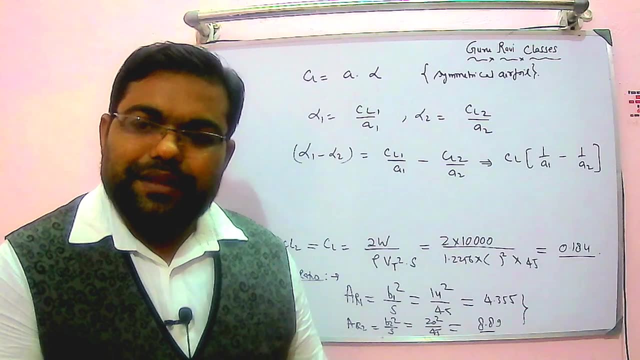 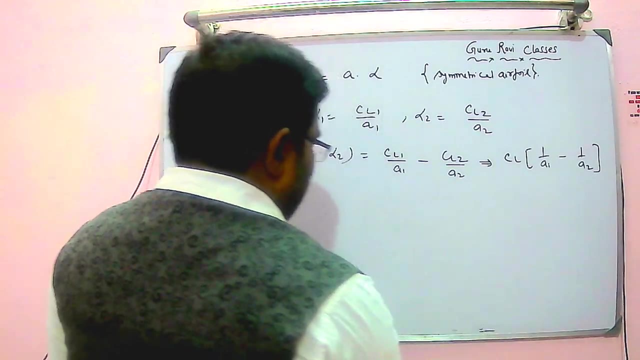 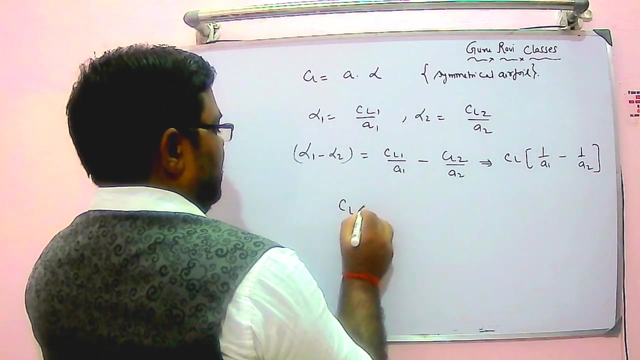 all right. so cl is common. so i can say cl is common. so i can say 1 by a1 minus 1 y a2. clear, Can I write like this? We have also derived an expression for the relationship of A with A0, right A with A0. So I will write here: So CL is CL bracket. I can say this is 1 by A0 plus 1 by. 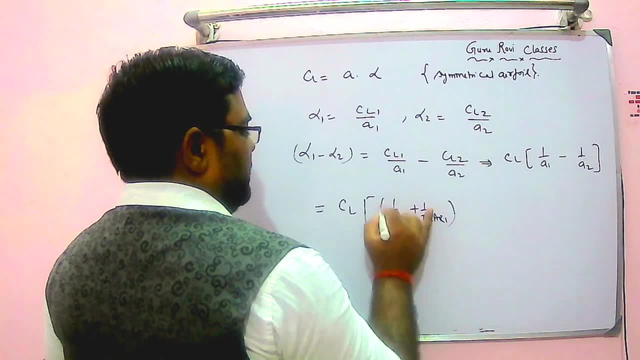 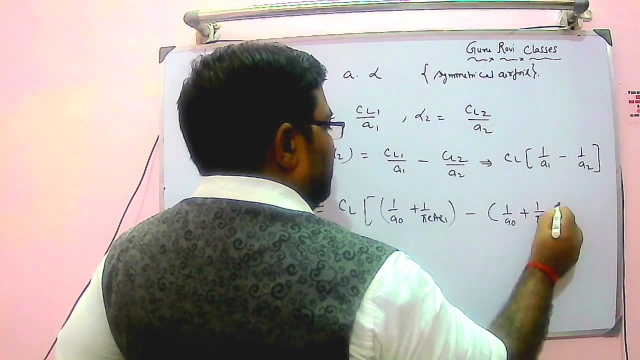 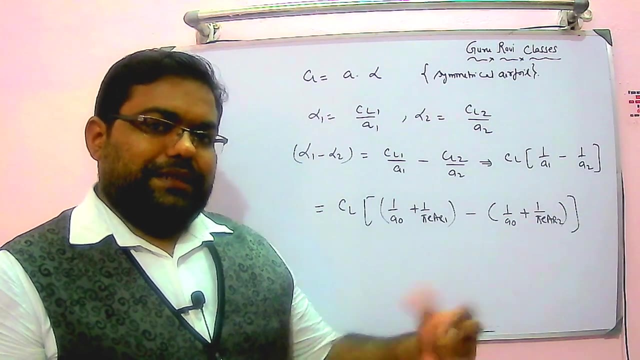 pi E aspect ratio 1, one term minus 1 by A0 plus 1 upon pi E aspect ratio 2, another term. So 1 by A is equal to 1 by A0 plus 1 by pi AR. That relationship we already derived in, I think so. 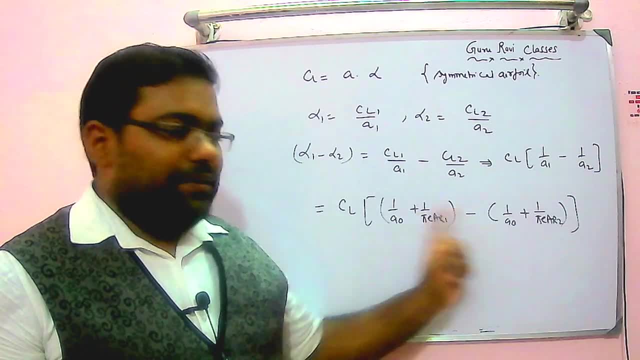 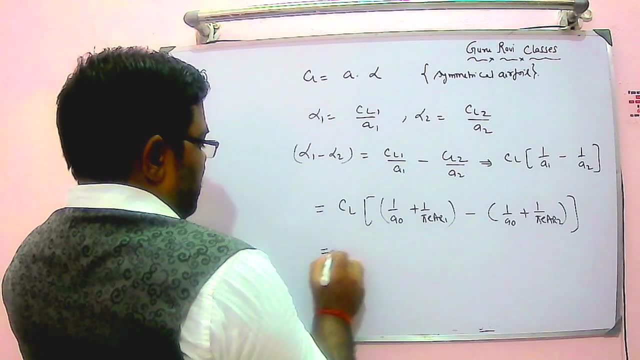 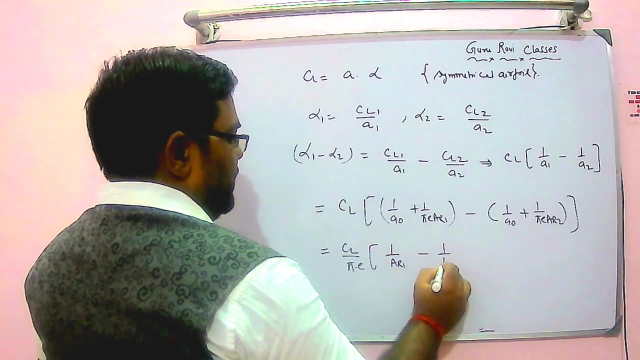 previous lecture So that can be kept here. So if you subtract this and this term will be cancelled out, I will get pi E. that is common. So I can write CL divided by pi into E and this inside will become 1 by A aspect ratio, 1 minus 1 by A aspect. 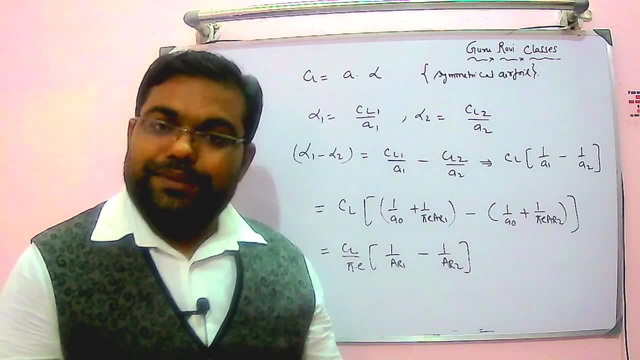 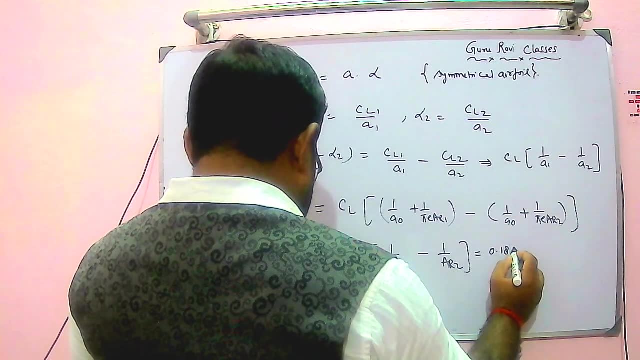 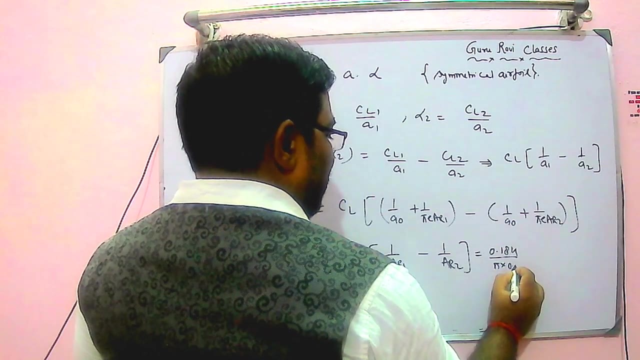 ratio 2. Clear. I can write in this way Yes or no. So now substitute the value. CL is 0.184, approximately divided by pi into E 0.85.. Always consider Oswald efficiency factor 0.85.. 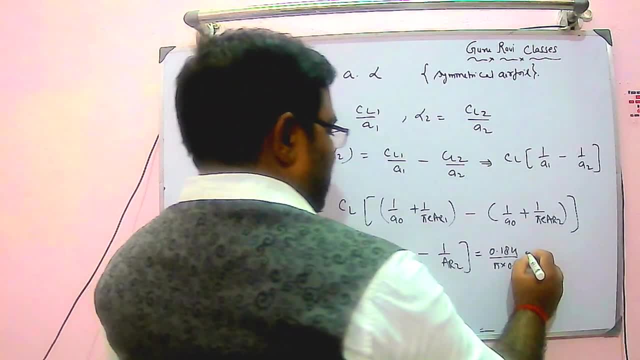 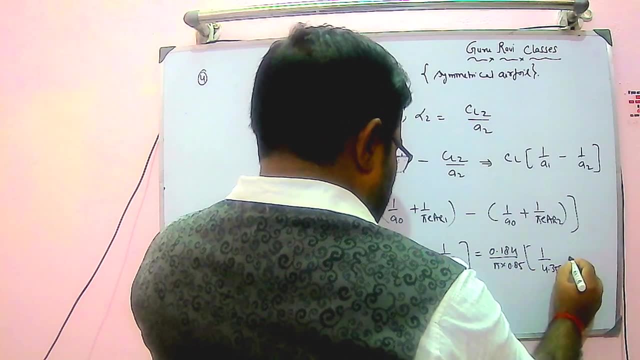 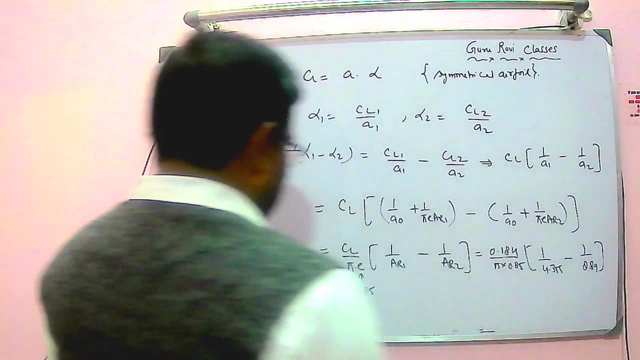 All right, You substitute here And then in bracket 1 by A aspect ratio 1.. A aspect ratio 1 is 4.355, right Minus 1 by A aspect ratio 2 is 8.89.. Just solve this, You will get alpha 1 minus alpha. 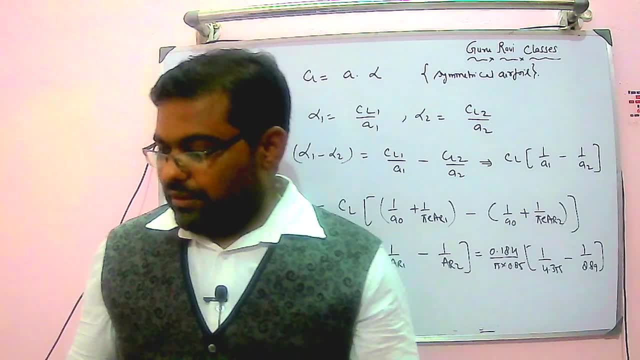 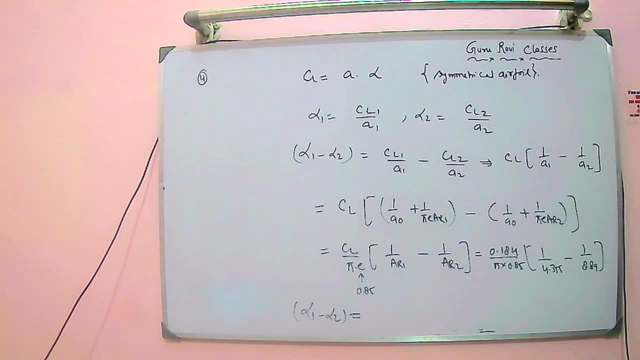 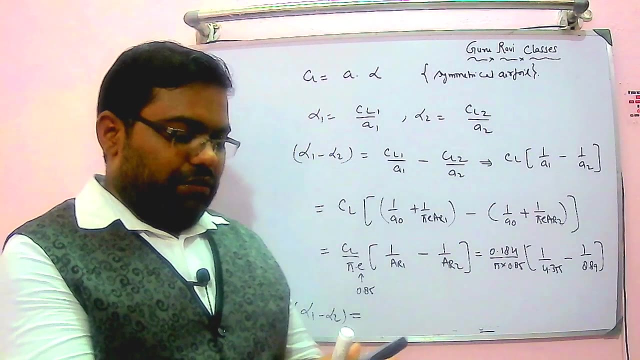 2 difference. So I need a calculator for this because I do not have answer, So I will take the calculator now. So here is my calculator. So if I solve this right, If I solve this, just substitute the value. 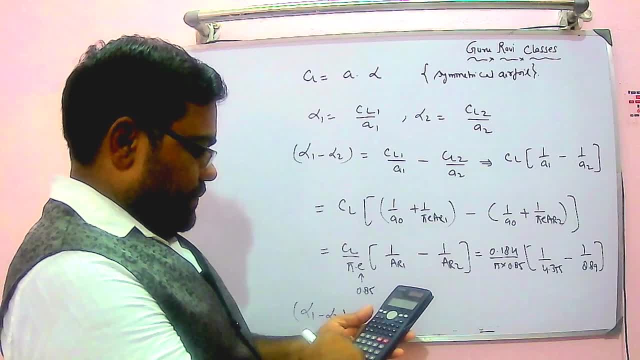 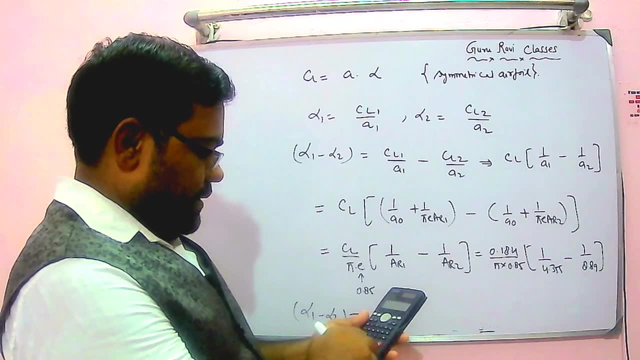 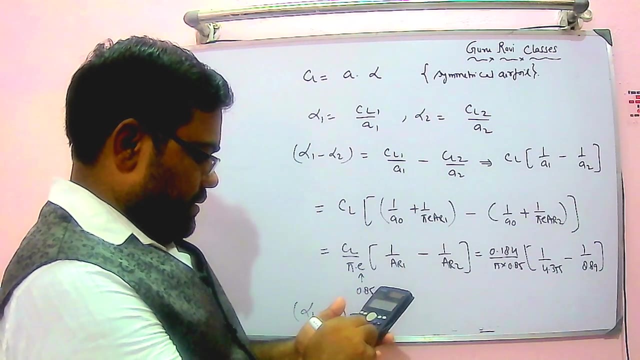 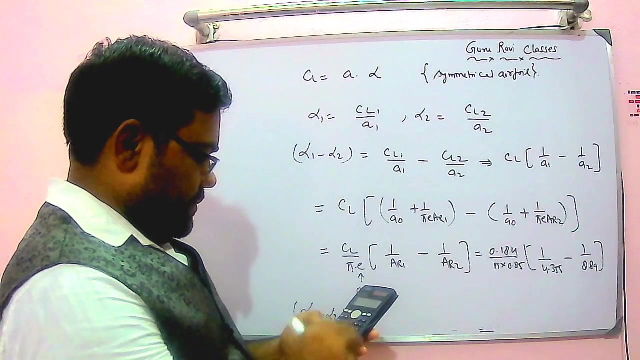 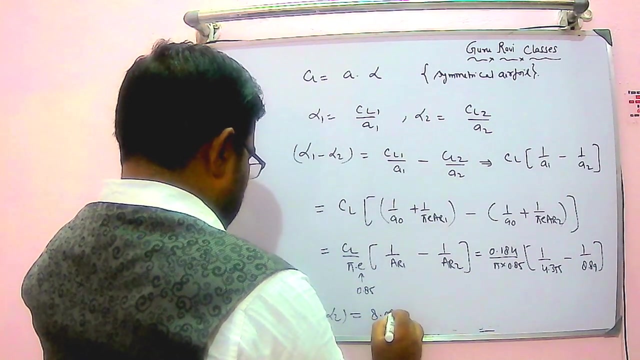 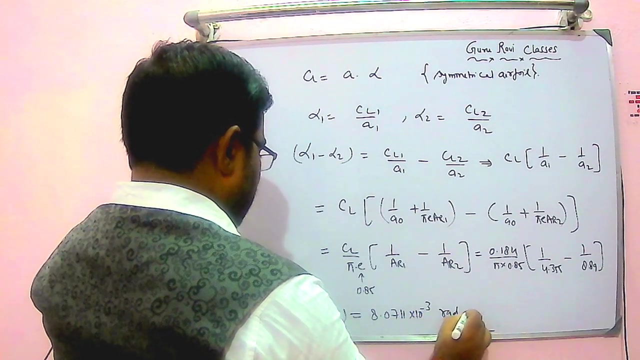 So I will say 1 divided by 4.355 minus 1 divided by 8.89 into 2.184 divided by pi. So this I got around 8.0711 and 10 to power minus 3 radian. All right, If I am putting E is: 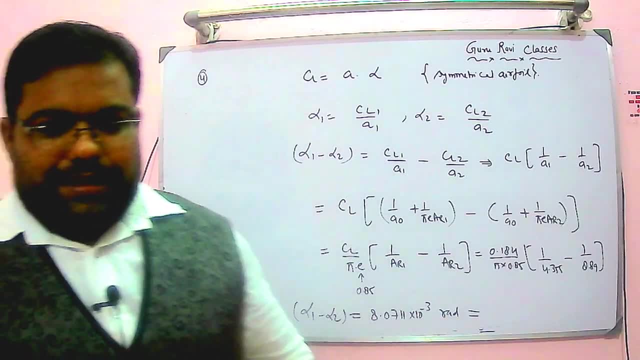 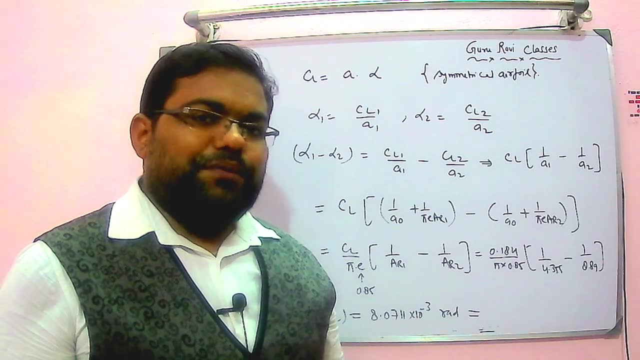 equal to 0.85.. So basically nothing is mentioned, whether it is a straight wing right Or it is a tapered wing. So I would suggest at this point, either you can put E is equal to 0.85, or even if 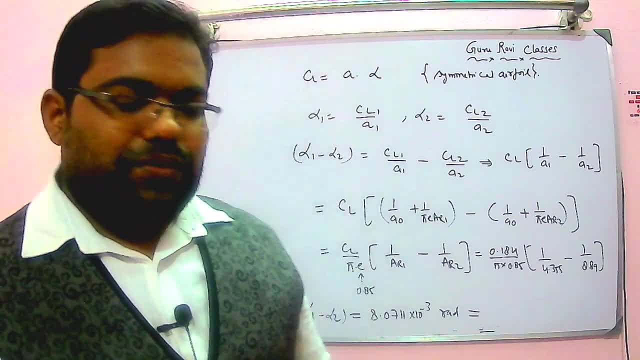 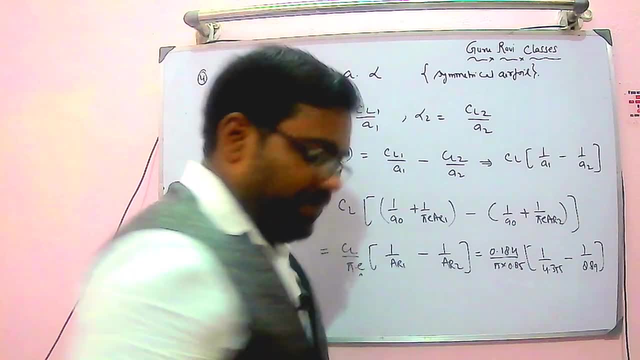 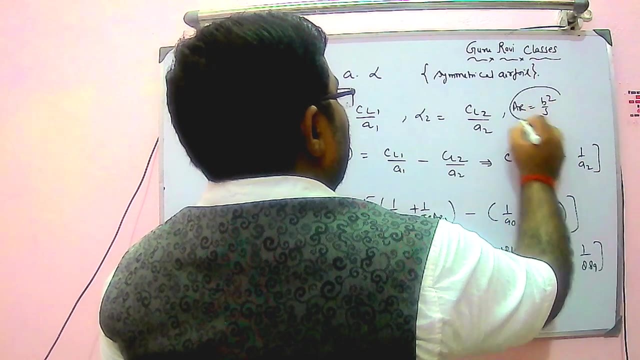 you are putting, E is equal to 1, that will also make your problem easy, So I will do that modification. I have to make one assumption right, So assumption is nothing. but already we have written: aspect ratio is equal to B square divided by S. This is applicable only for. 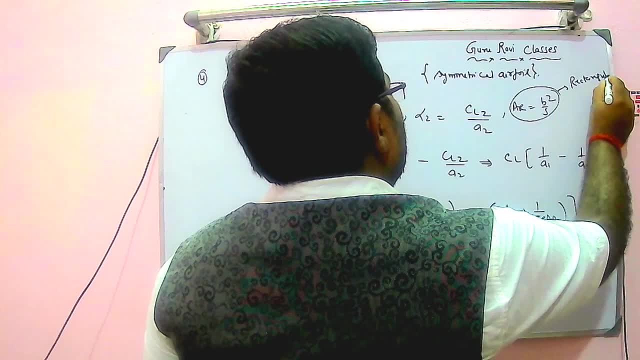 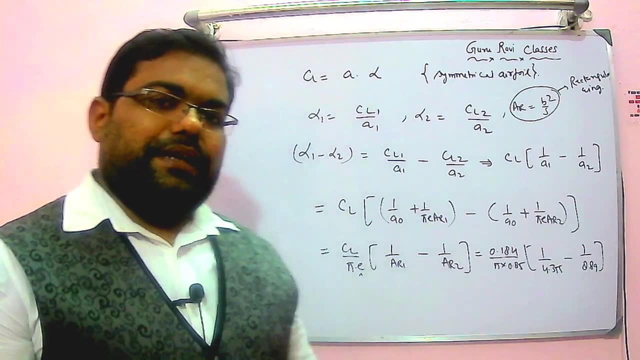 rectangular wing Wing right And for rectangular wing, basically also all efficiency factor is equal to 1.. There is no meaning of it. right, E is equal to 1. And for rectangular wing E is equal to 1.. So if you put 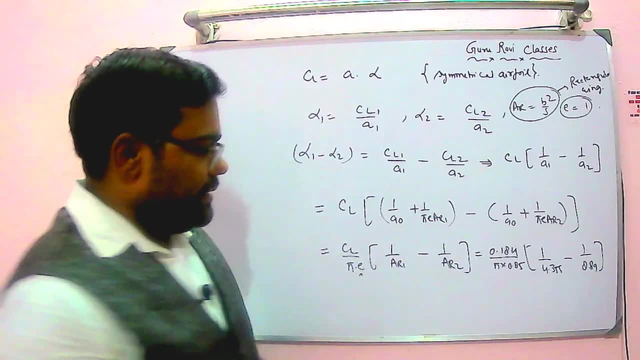 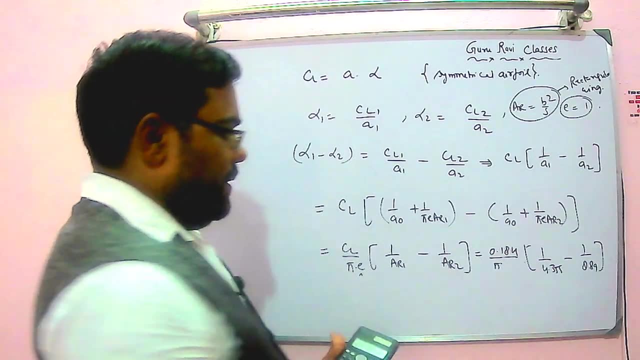 1, there is no meaning of E. now, right, So this you can remove, This you can remove, basically. So if you are going to remove this, so whatever value that you are getting if I multiply that with 0.85.. 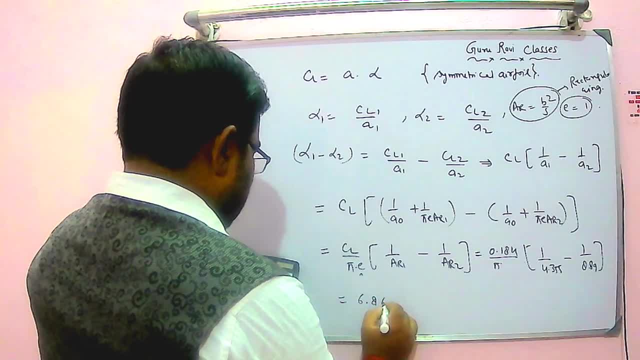 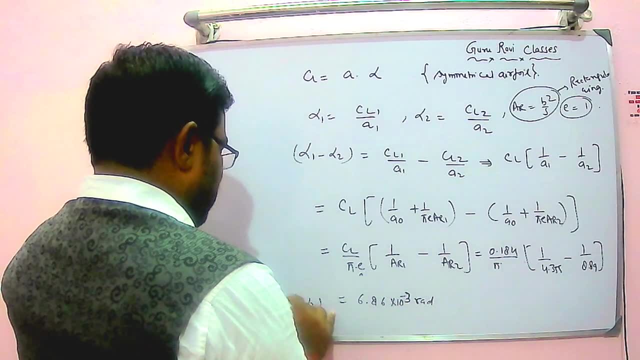 I am getting this value around 6.86, 10 to the power minus 3 radian right. This is alpha 1 minus alpha 2.. So if you convert that into degree, what do you need to do? You need to multiply by. 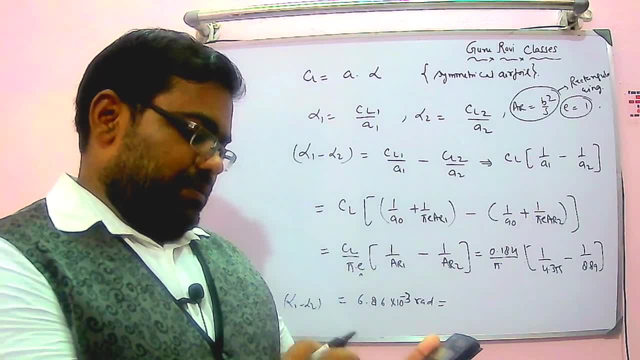 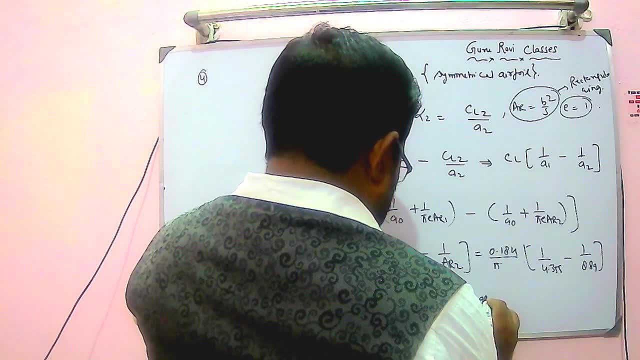 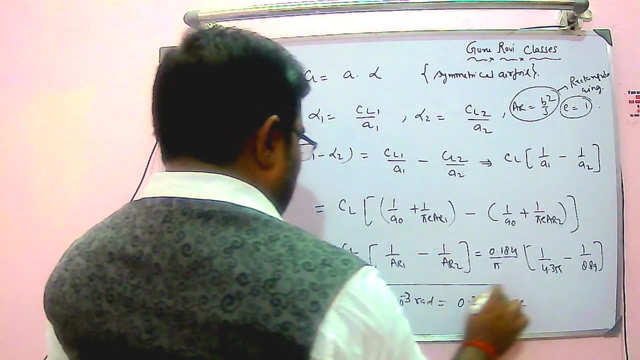 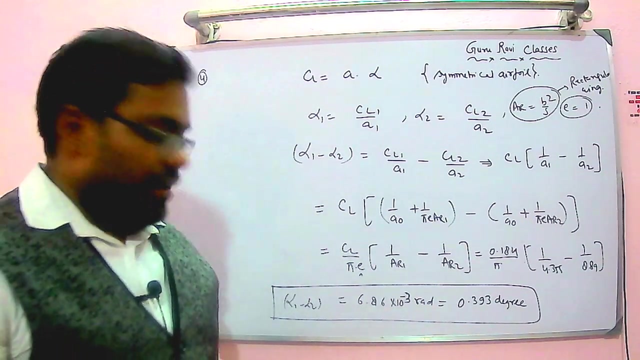 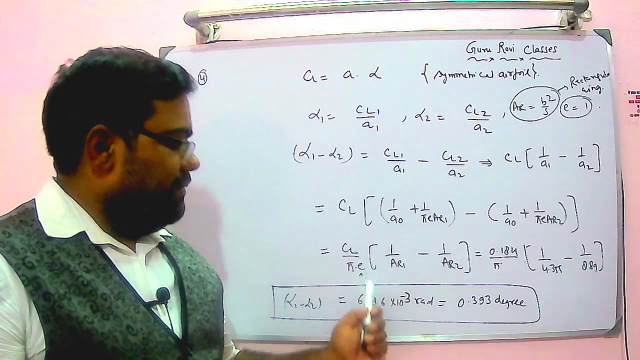 180 divided by pi. So if you do so, so it is coming around 0.393 degree. So this is the difference between the geometrical angle of attack, difference in geometrical angle of attack which is coming around 0.393 degree. Where also all efficiency factor, basically E, we. 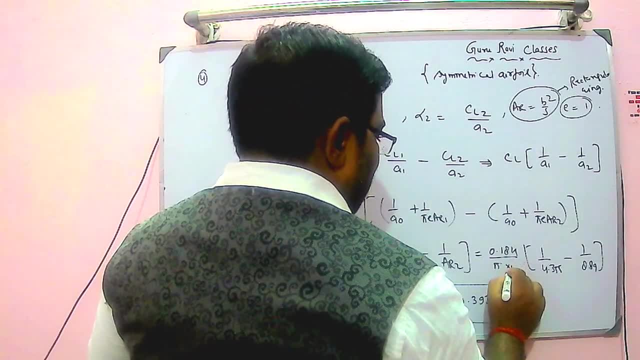 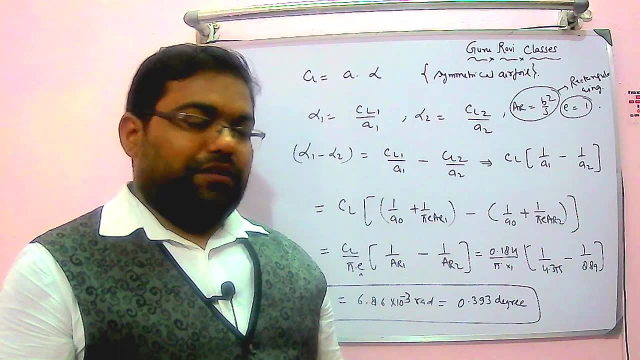 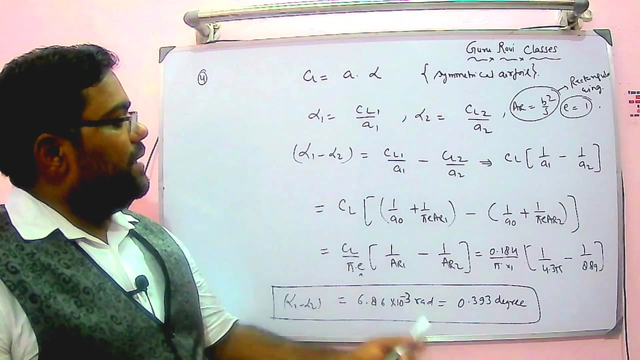 have taken as 1, because? why? Because we have taken wing planform area means profile as rectangular wing and for rectangular wing it is 1.. Like that you can solve. So I don't think so there will be any doubt in this Very simple step. 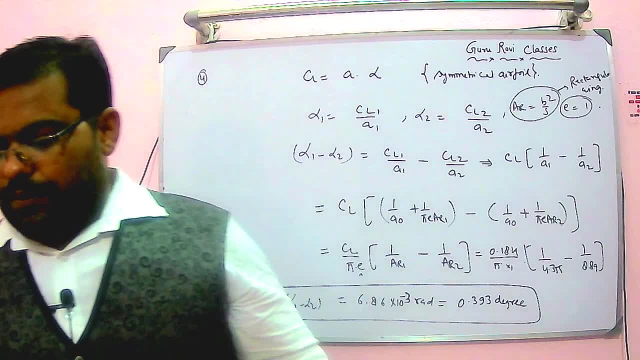 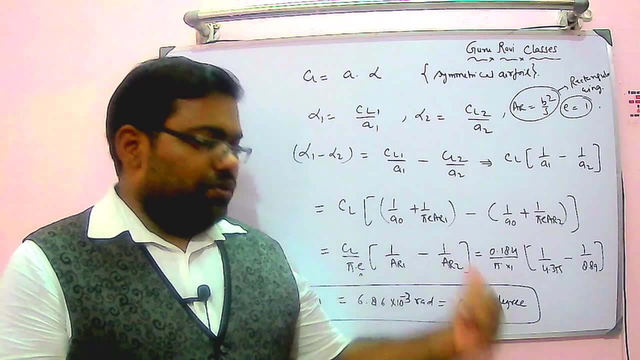 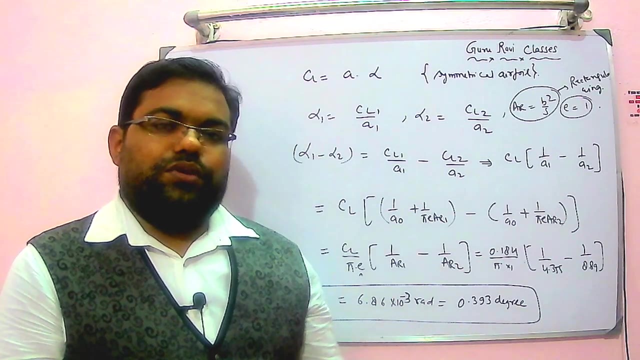 right like that you can solve. So I think for today this much is enough, right? If you want to explore more numerical problems, right Go through the reference book, or you can say standard textbook, John D Anderson: introduction to flight. There are around two or three more problems are given, right.